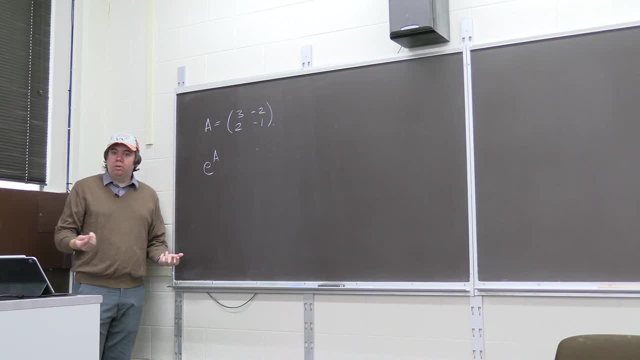 So the exponential function is defined for numbers, for real numbers. We can also define it for complex numbers. but how do you do e to some function, Some function of a matrix, e to the, a right. So any thoughts? How can we do this? 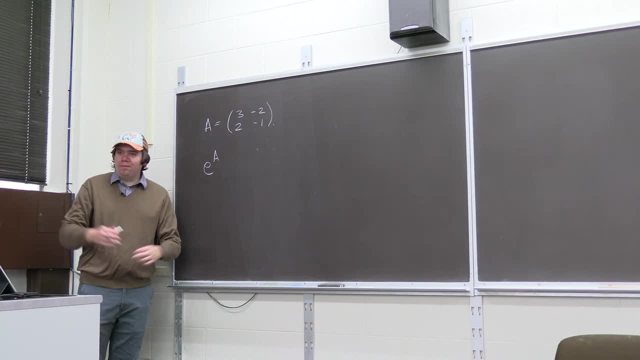 Yeah, okay, that's the right answer. But first let's give a wrong answer so we can feel like we built up to something right. So what you might do is you might be like: oh, let's just add each, let's just like take. 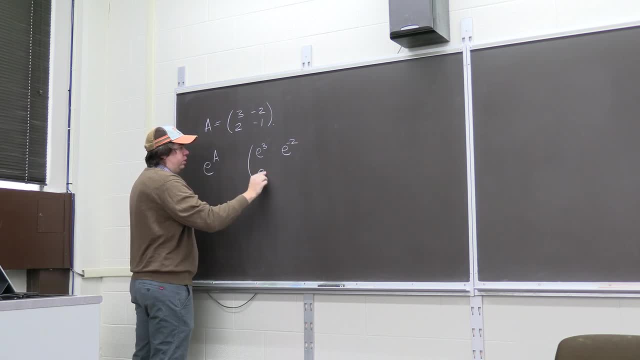 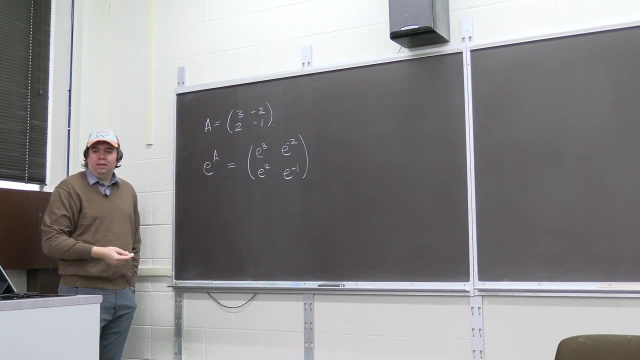 Let's take each entry and do e to each entry, right? So you might be like: oh, maybe we should define it this way. It's like it's simple but it's dumb And it's like: what's the problem if we define it this way? 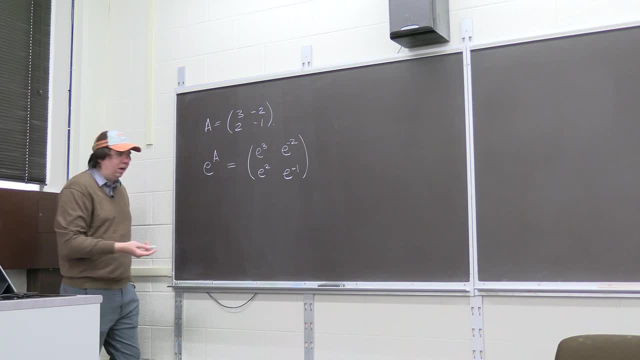 Well, this doesn't really respect the structure of a matrix, right Like? yes, it respects the values, but the reason we might be a little bit offended by that is when you think about just something like a squared, we don't define a squared. 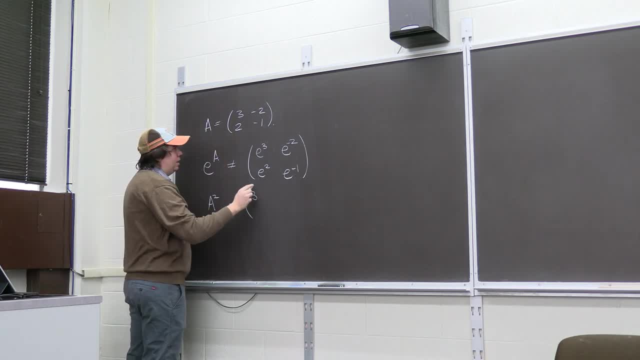 to be just entry, each entry squared right. It's not like it's just three squared minus two squared, two squared minus one squared Like. that's not how we define a squared. Instead, we define a squared by this. you know: interplay of the rows and the columns. 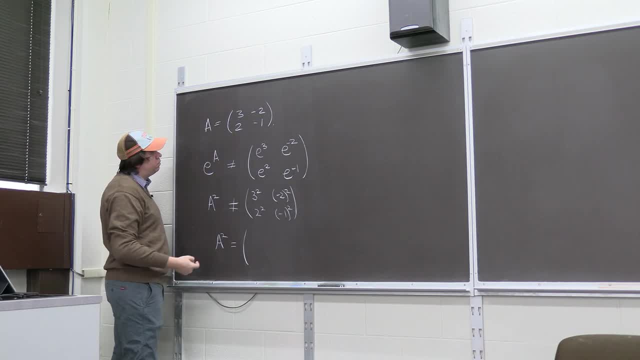 and doing our matrix, multiplication, Row times column gives you nine minus four, which is five. Row times column Gives you negative two and negative six and positive two, which is minus four. Did I get that right? Row times column is six minus two, which is positive four. 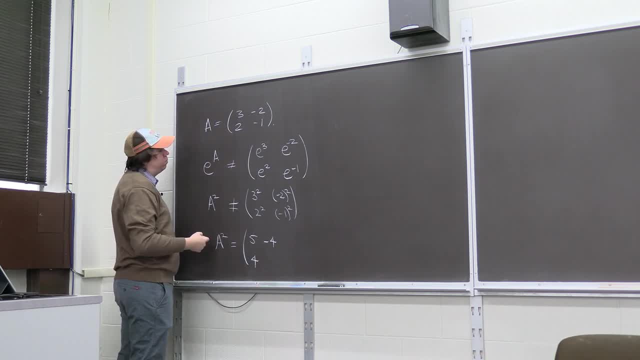 Row times column is minus four times minus four plus one, which is minus three. Does that look right? I think I did that right. Very good, So this is. you know, when we do matrix multiplication it's not just squaring each entry. 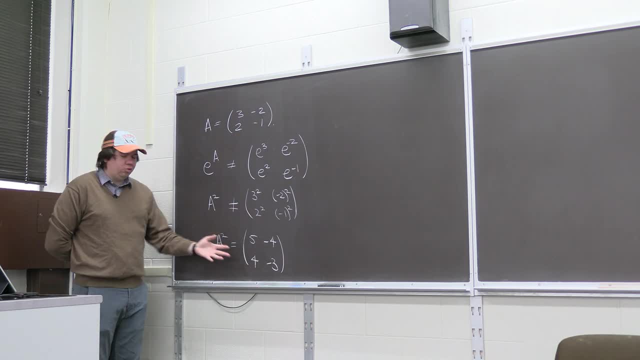 We actually? We want to somehow respect the structure a little bit more of the matrix And we want to respect how we define matrix multiplication. After all, the whole point of this course has been like matrix multiplication is a meaningful thing. Like matrices encode linear transformation. 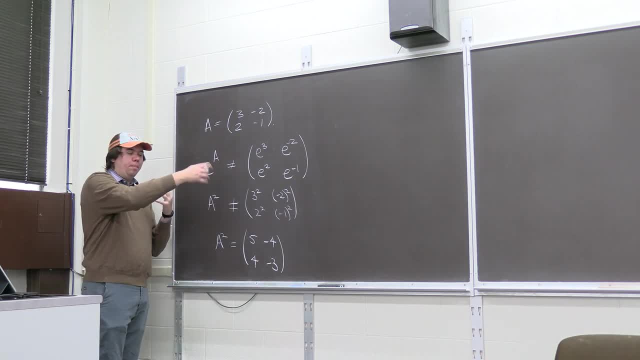 And multiplication between matrices is encoding compositions of linear combinations of linear transformations, And so it's like we want to respect that story. So we shouldn't just raise each entry. So what do we do instead? Well, exactly What was just said. 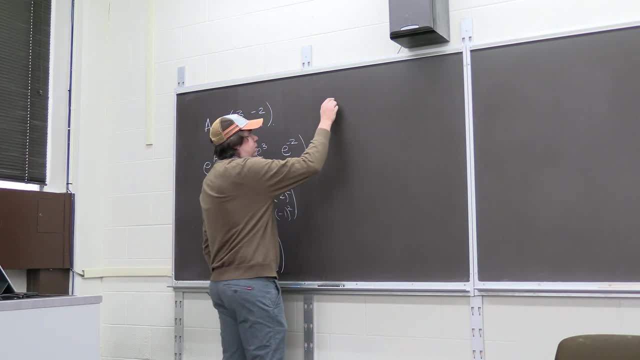 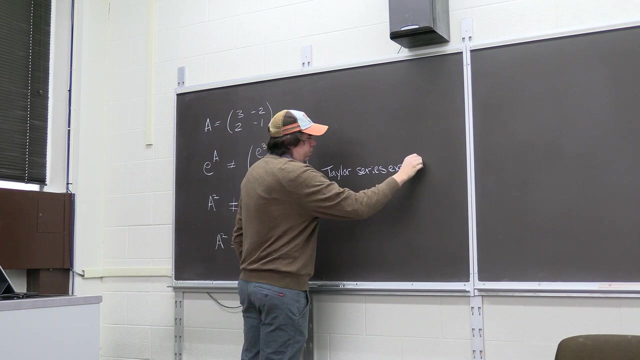 We know that the function e to the x, We know that e to the x can be written as a Taylor series. So we have this Taylor series expansion. This is like where you're covering calculus two right, Where, let's say, we expand it about the point zero. 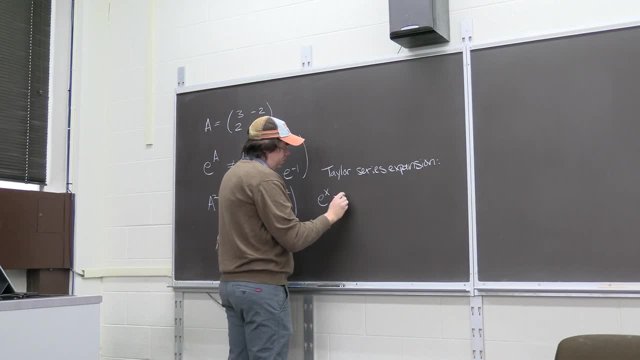 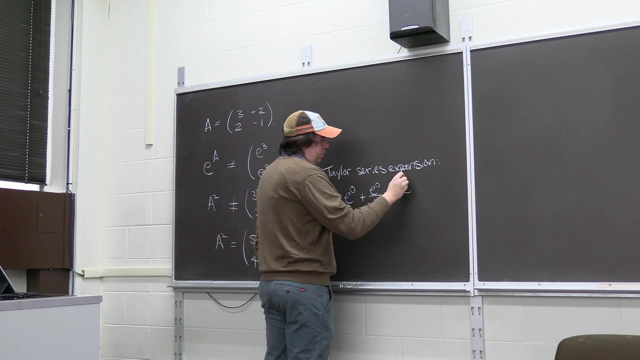 This would be just e to the zero, e to the zero Plus. then you do the derivative of e to the x, which is just well, the drive is all e. So this isn't very interesting. Just e to the zero over one factorial times x plus. the derivative is still e to the x. 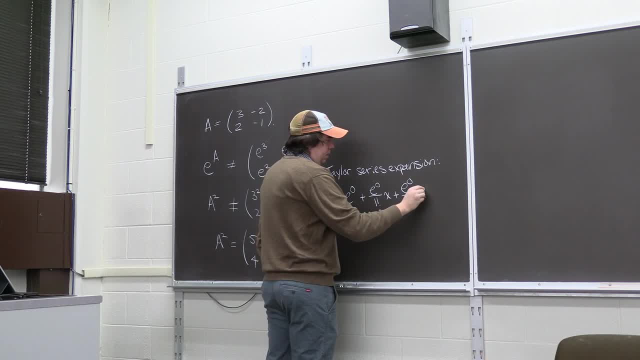 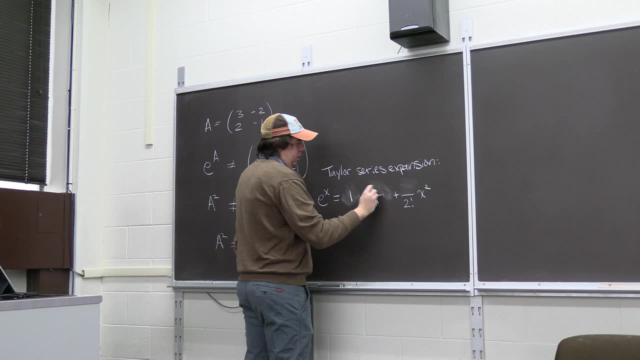 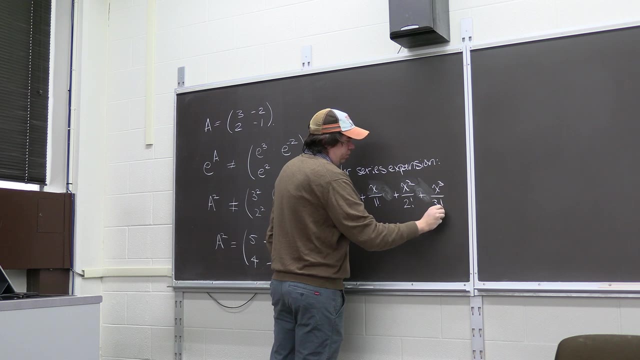 So it's e to the zero over two factorial times x squared, And so this just simplifies and you get the really nice series One plus X over one factorial plus x squared over two factorial plus x cubed over three factorial, and so on. 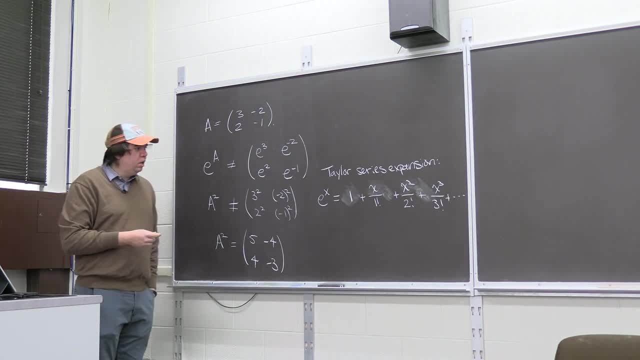 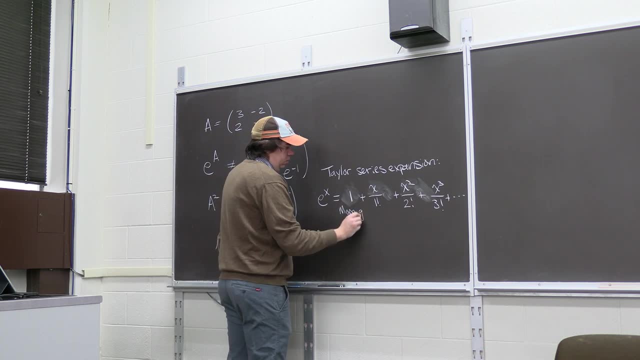 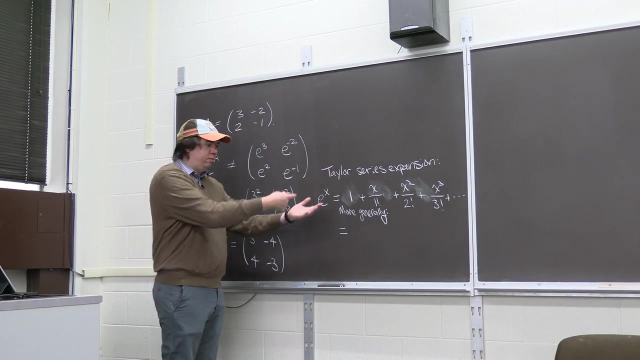 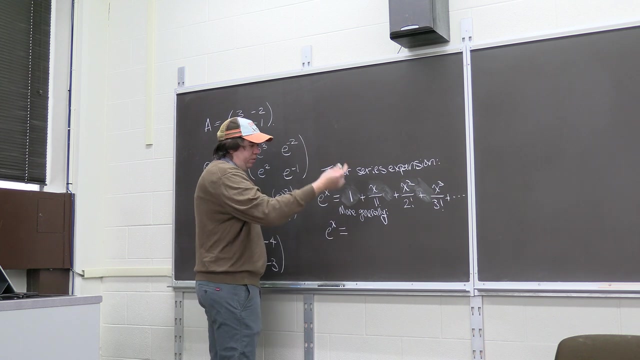 That infinite series right. More generally, If you want to expand about some point a, So some value a. You don't have to do around Zero, You can pick some, some number a. That's whatever value a you want. Could actually be any complex number you want. 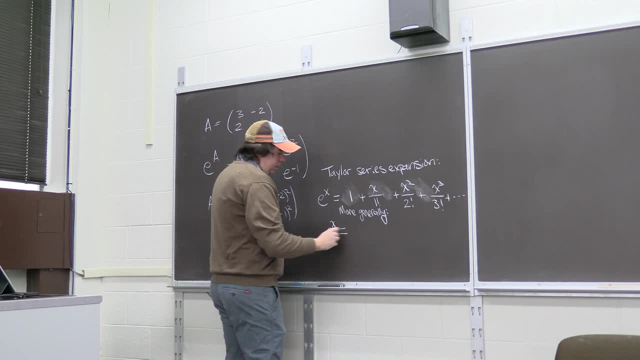 Doesn't have to be real Expand about i or whatever. Then this is just going to be of the form E to the a plus the derivative e to the x, which is still e to the a over one factorial times x minus a. 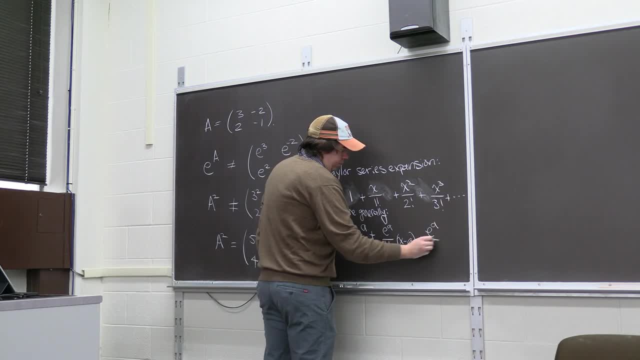 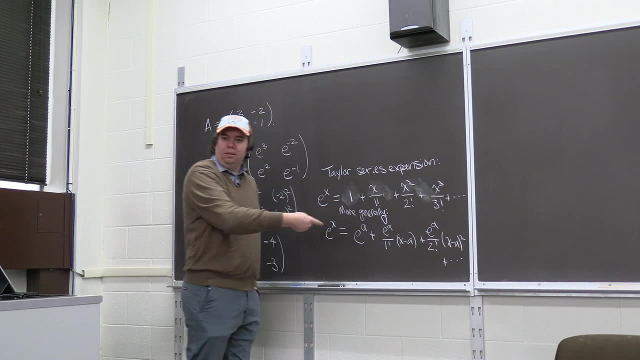 Plus the derivative e to the x is still e to the a, over two factorial times X minus a squared, and so on, forever. Right, Do you remember this a little bit, These Taylor expansions? So So let me just remind you in general what this looks like. 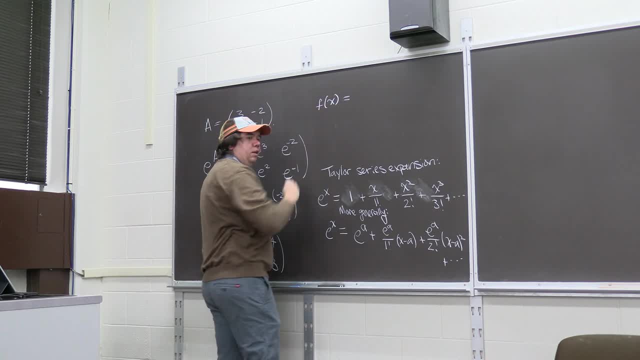 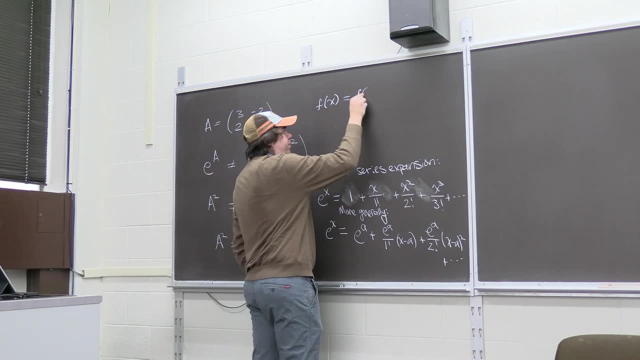 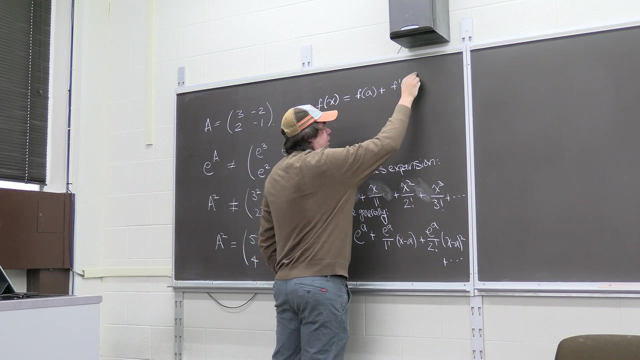 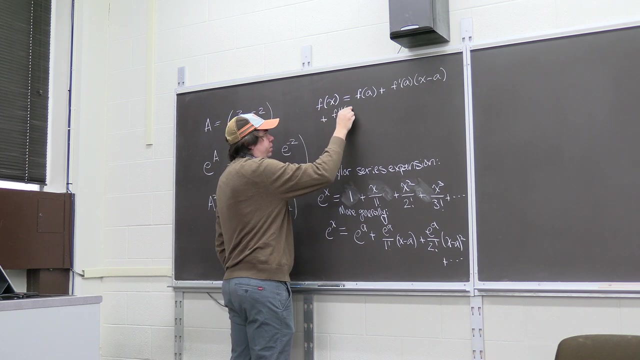 Given some function: f of x in general, the Taylor series expansion about some number. a is just f of a plus the derivative of f a times x minus a Plus the second derivative of f at a over two factorial. There's a one factorial there, but that's just one. 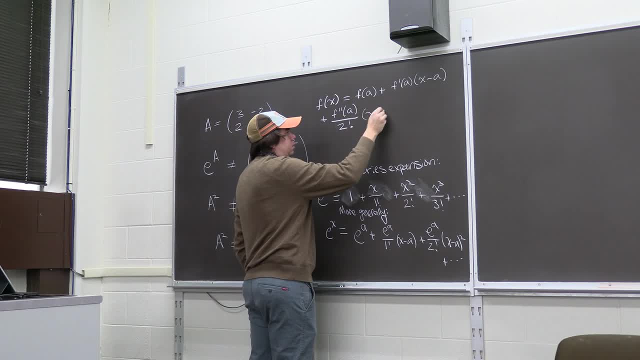 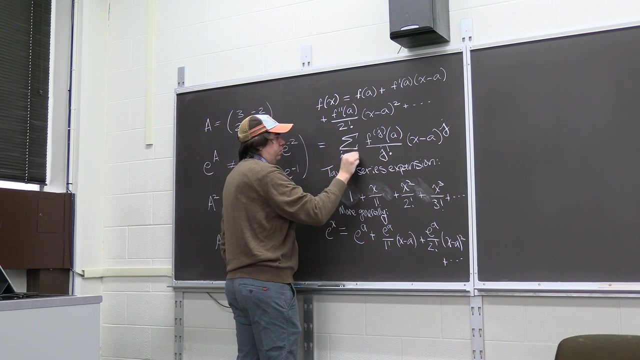 There's a zero factorial here, but that's just zero times x minus a squared and so on. Right That is. you can write this as just the sum of the jth derivative of f at a divided by j factorial Times x minus a to the j where j goes from zero off to infinity. 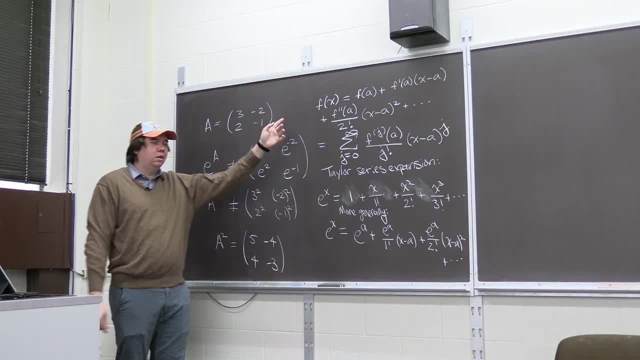 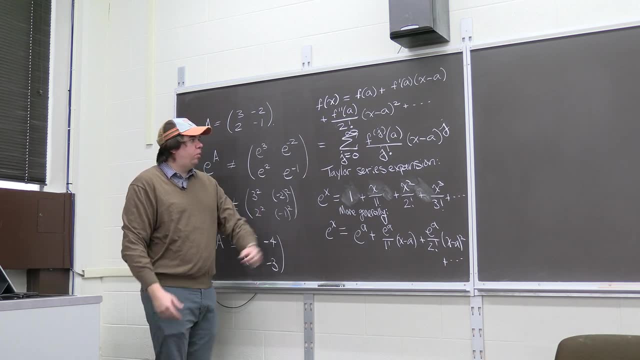 That's our Taylor series. Okay, Taylor, expansion of a function. Now, a big portion of calculus two is thinking about like: oh, when does the Taylor series actually converge to your function, Right? So? So maybe a word that you may have heard before or maybe not, is we say that this is? 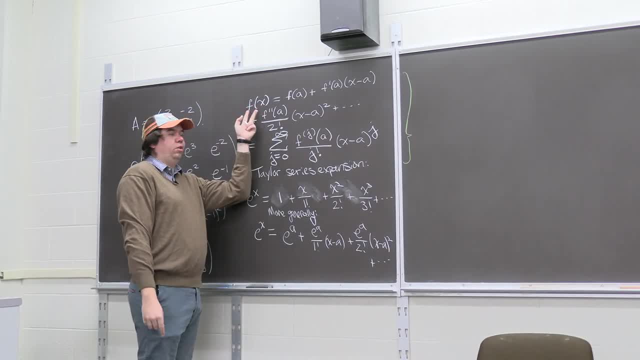 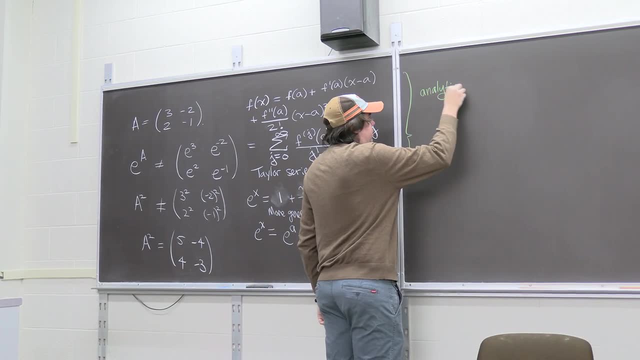 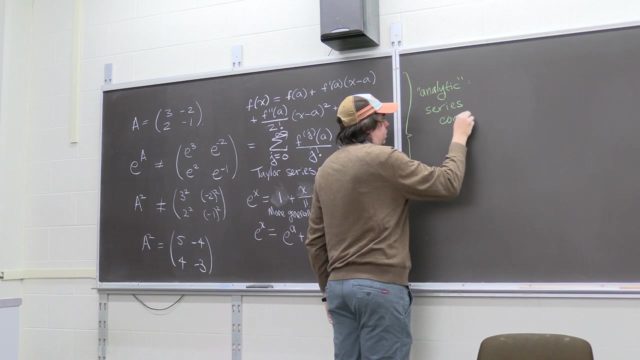 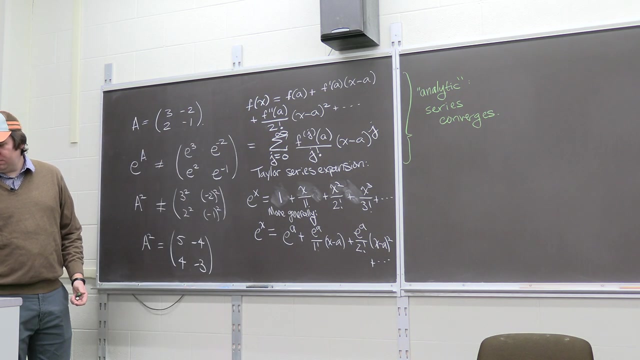 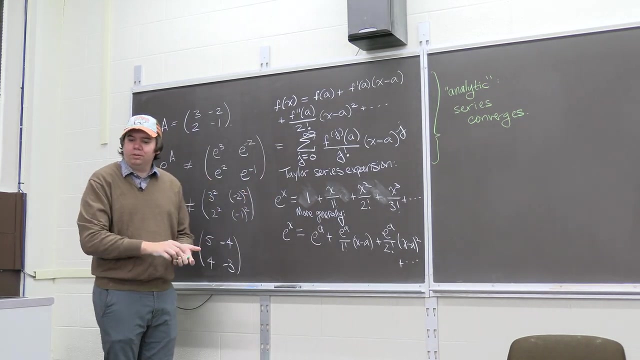 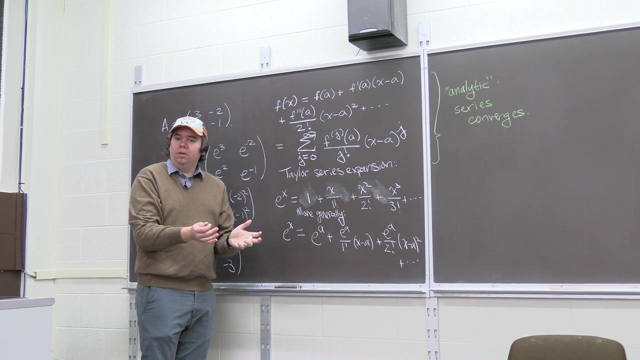 This is analytic if it converges to f of x, right? So analytic is just a word, meaning that the series converges. And then what you might remember from you know calculus two, or maybe Maybe you've seen this in some analysis course or something- is that these, these converge on like some open interval, right? 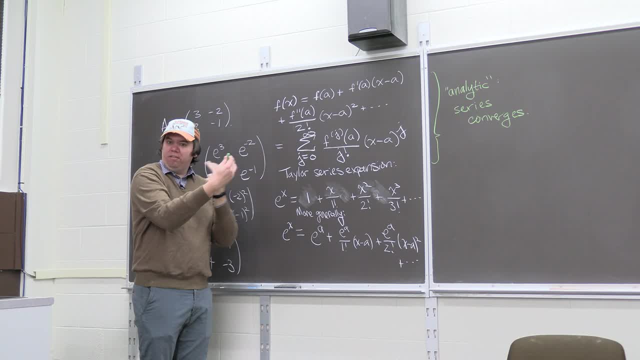 So if you're working on the reals, it's like you have some a and then you find the radius of convergence- Remember all that right- And you have some open interval, And so for some functions the radius may be infinite and it may converge for all real numbers. 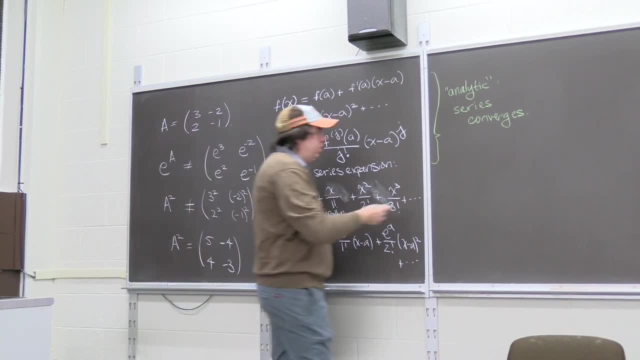 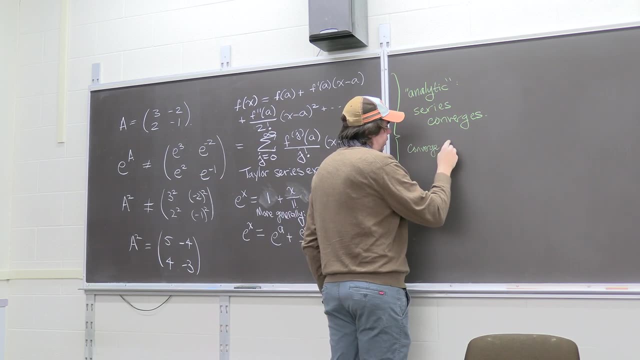 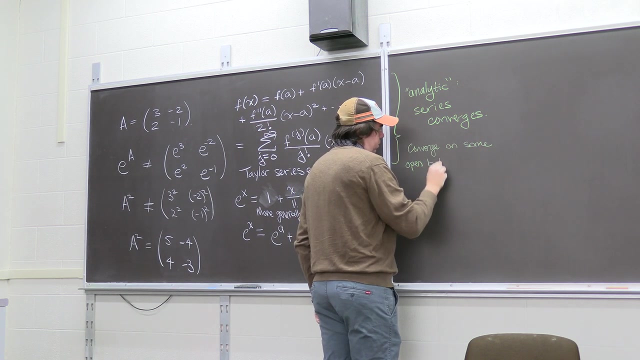 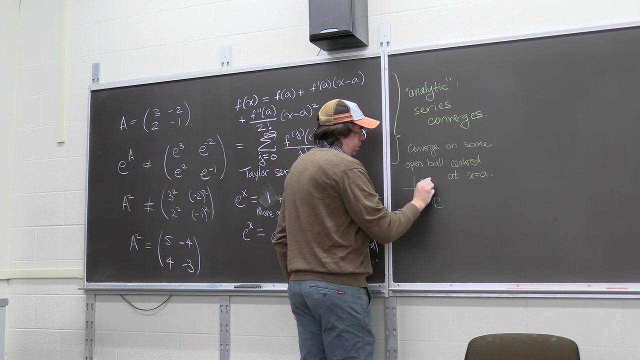 But you guys do have a complex numbers and seven open interval, You have an open ball And so, and so, in general, these, these converge, You know, on some open ball. So so converge on some open ball centered on a, centered at x equals a, and I'm saying ball just because if we're in the complex plane, then you know you're two dimensions. 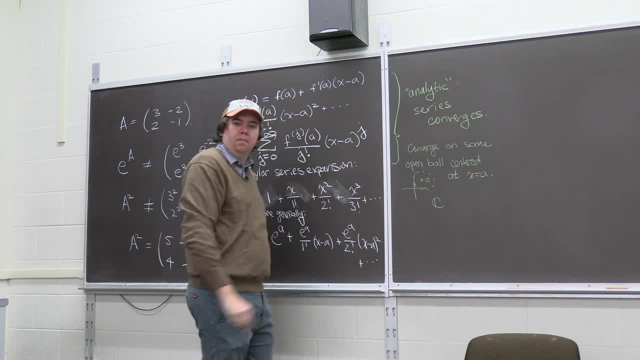 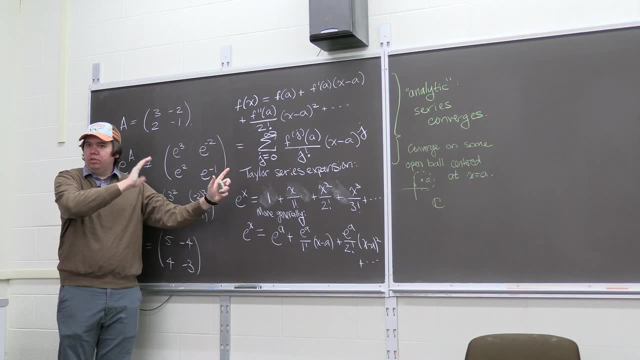 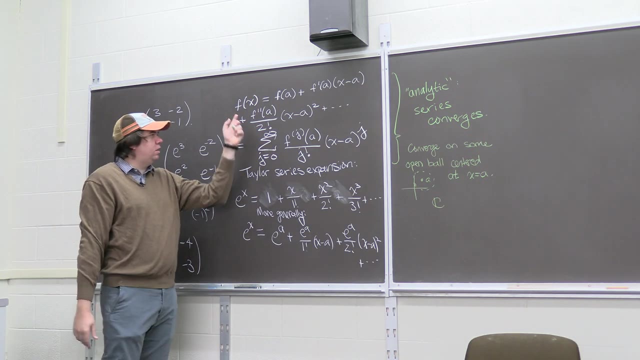 And so your ball is something like this: right, Okay, Is this familiar? We feel vaguely comfortable. Taylor series and you've talked about this and this isn't. this isn't disturbing you too much. If you ever like, forget this like one little hack you can do is you can just be like okay. 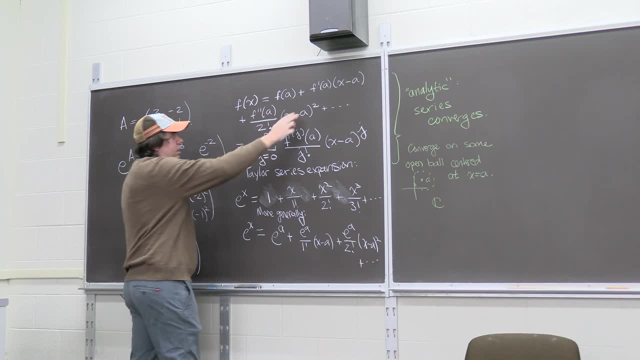 when I plug in a to left-hand side should equal the right-hand side and these all vanish, the x minus a terms all vanish, So they're equal. Or if I take a derivative and then plug in a, what happens? Taking the derivative? he vanishes and this goes away. 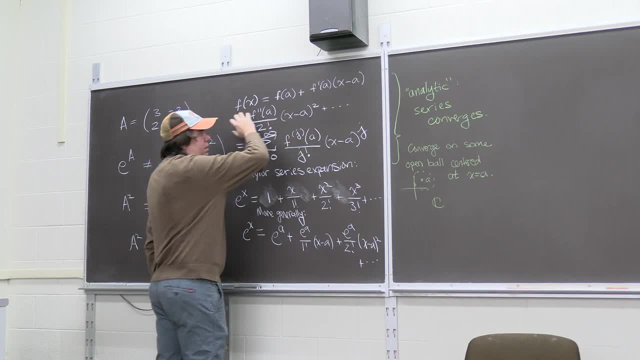 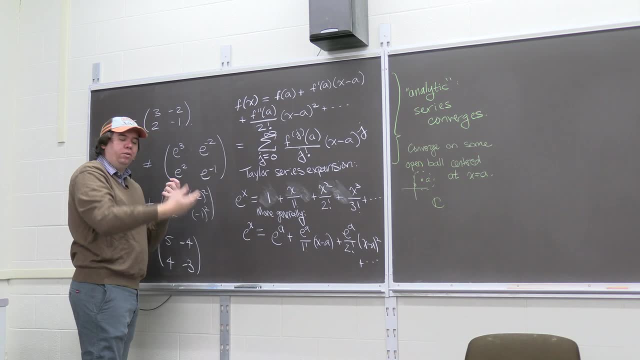 It's just one And everything else. when you plug in a, then vanishes, or you just have f prime of a which agrees, And so this is really designed so that if you plug in a or you take a few jitters and plug in a, the left-hand side equals the right-hand side. 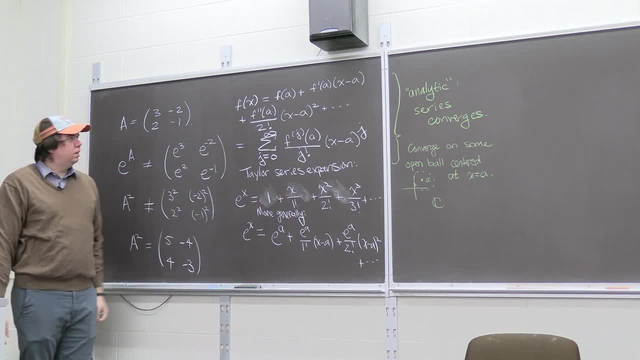 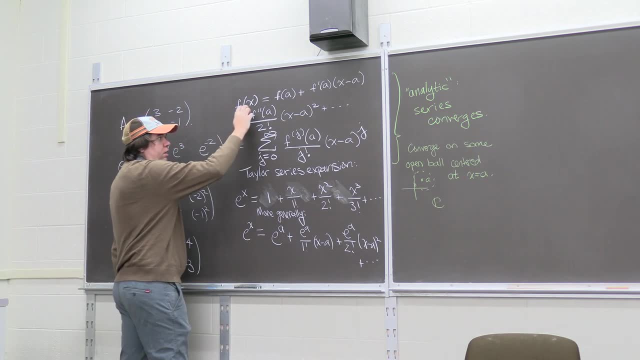 And so sometimes it's a little mnemonic you can use to try and remind yourself of how these are expanded. Anyway, the point is now that we can define functions in terms of just sums of powers of things. let's do that for something like e to a minus a. 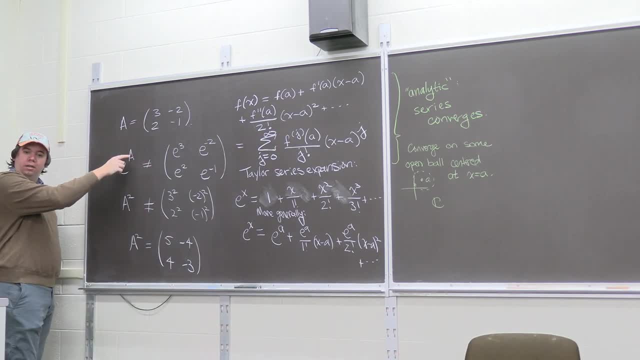 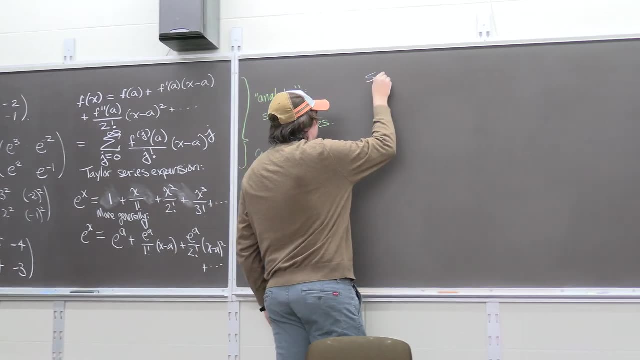 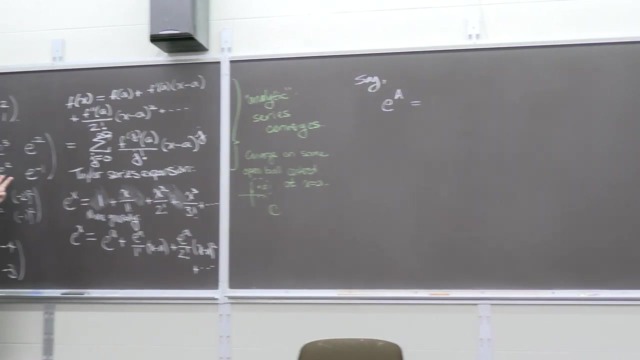 Okay, Let's do that for something like e to a matrix, a Right. What I want to do is I want to say that e to the a will just be defined as the analogous thing with matrices, right. So instead of being some x, we're now plugging in a matrix. 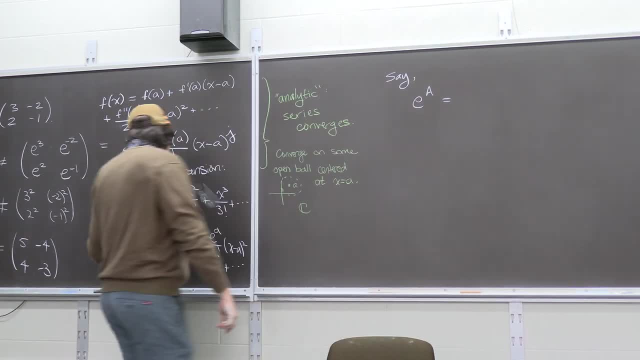 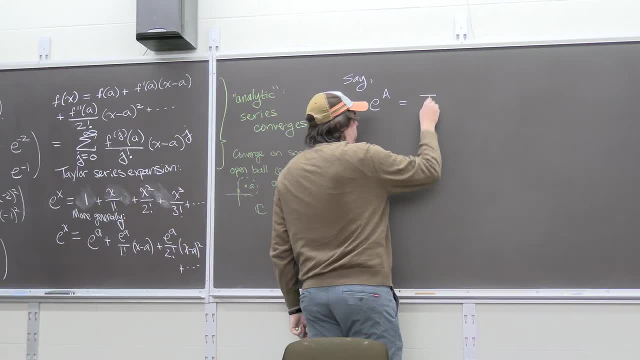 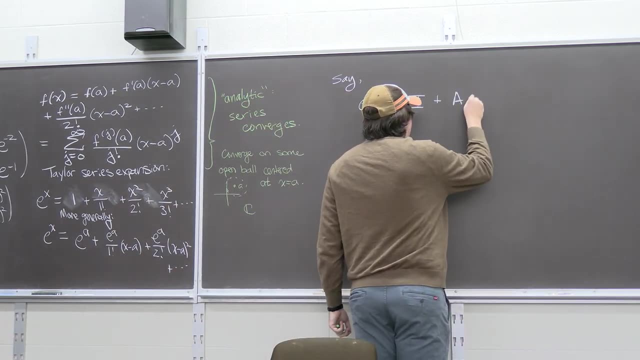 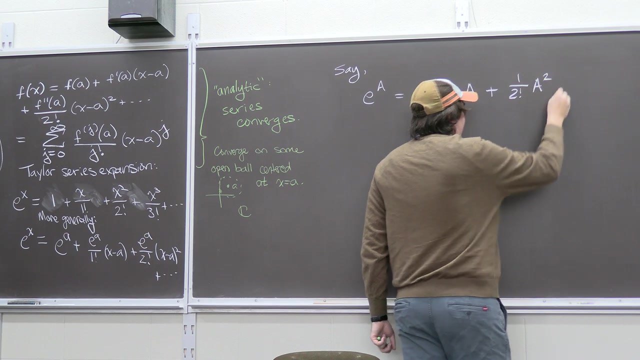 It's a matrix. It's a matrix, Identity matrix, That's right. So this should just be one identity matrix plus. and then it's like: here's an x, so that's just a copy of a plus, here's x squared, and you have a factor you're scaling by, so it's 1 over 2 factorial times a squared, plus 1 over 3 factorial times a cubed, and so on. 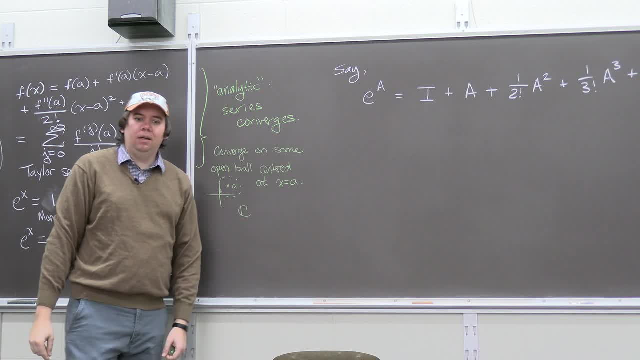 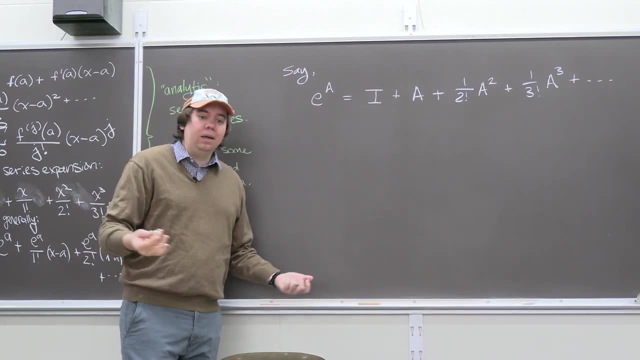 Right, That's where we want to say e to the a is, And then, analogously, we're going to be able to define other functions. And then we're going to be able to define other kinds of functions, Things like, I don't know, sine of a or cosine of a, which also have series expansions. 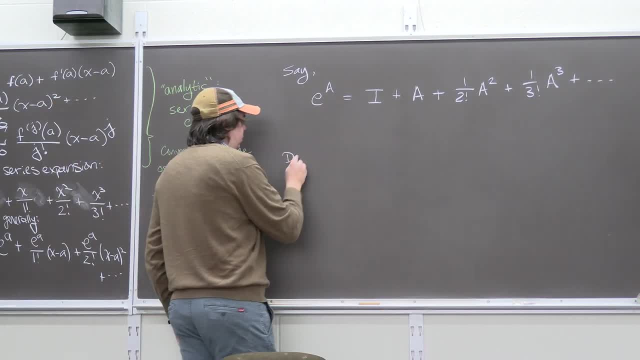 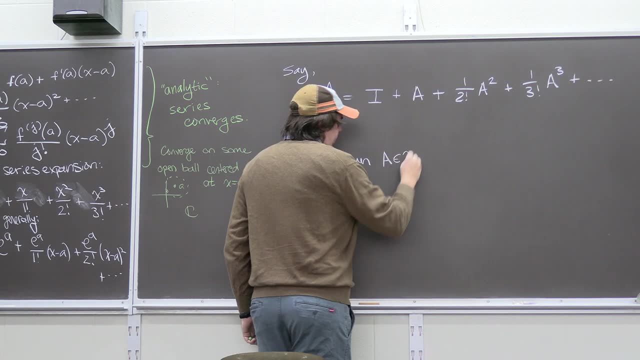 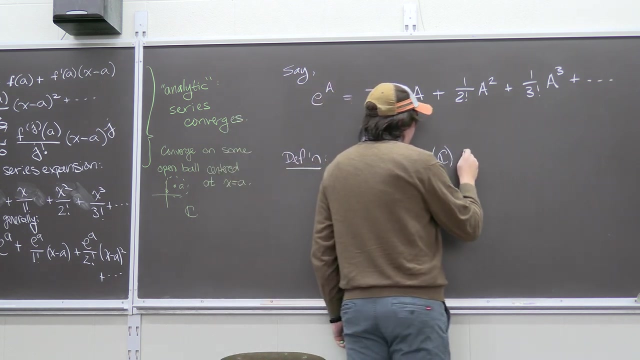 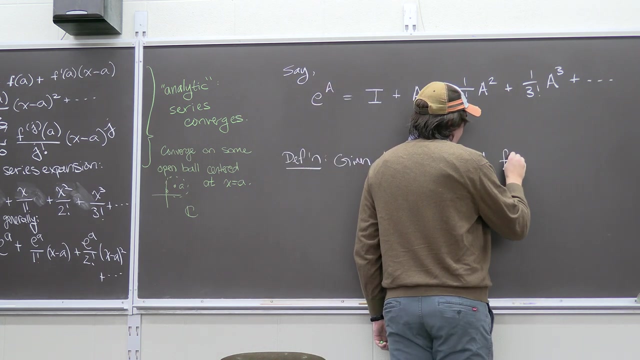 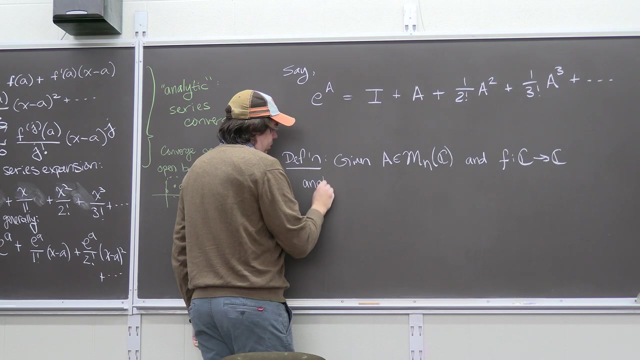 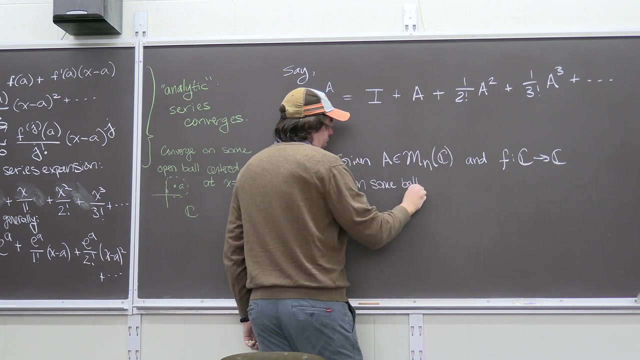 So in general we're going to define if we're given some matrix, a square matrix, And we're also given some analytic function. so some function f from complex numbers to complex numbers where the function is analytic on some ball centered at you know, whatever point you want. 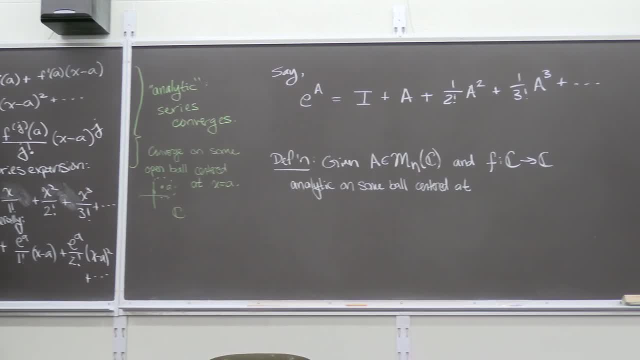 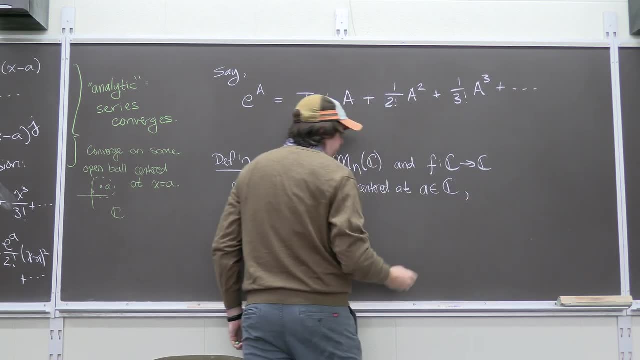 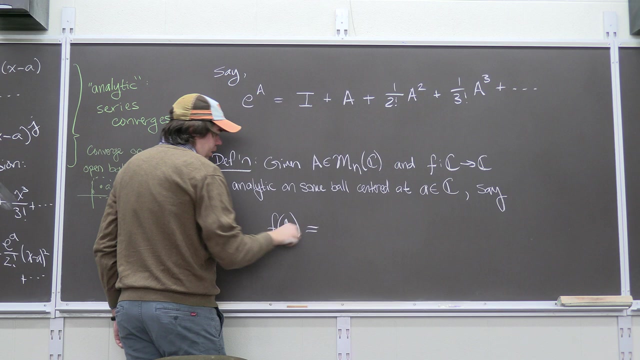 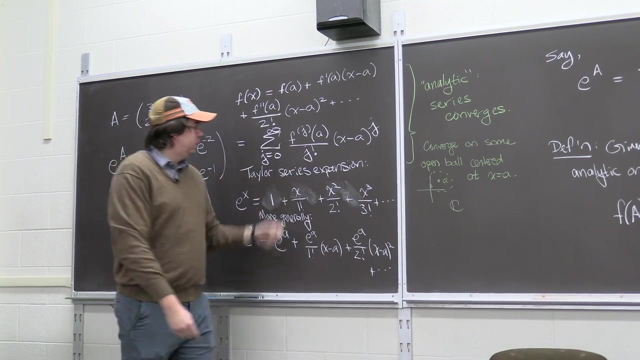 Right. So if we want at some point a, we want to say so centered. at some point a, we're going to say that f of a matrix is exactly what you get when you just plug a into this formula, the matrix a into this formula. 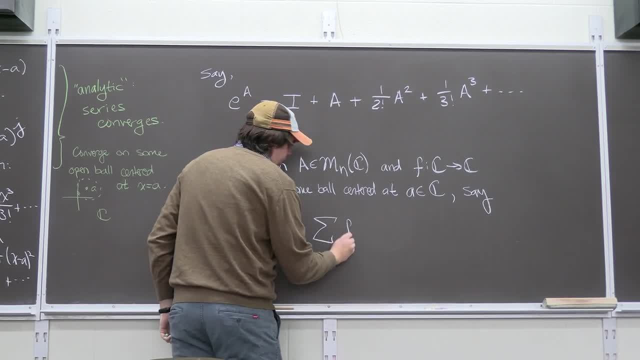 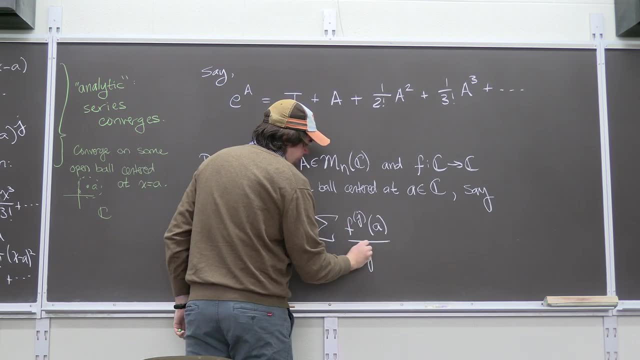 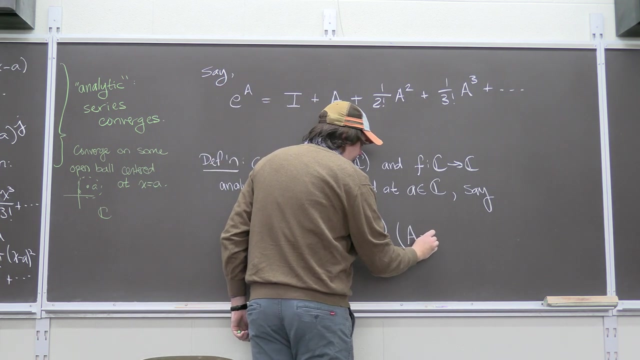 It's the sum of the jth triangle, The jth derivative of your function, determined at a divided by j factorial. This is a number, This is a scalar Times your matrix, a minus. well, we've got to be careful. It's like: how do you subtract a scalar from a matrix? 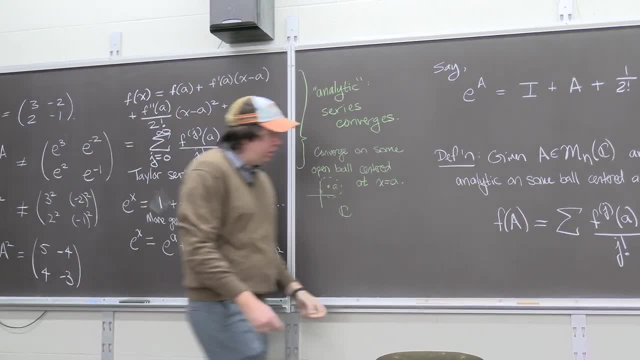 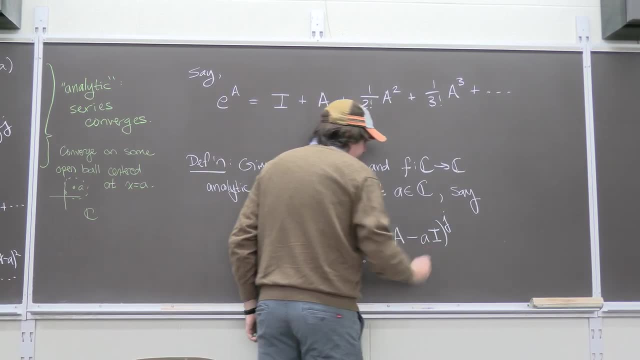 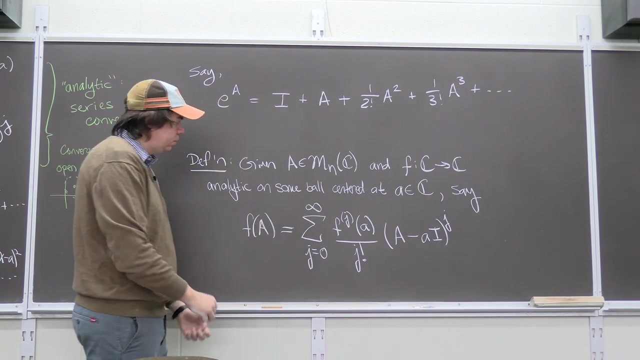 You're like. well, that's equally a times 1 or a times the density Right, A your matrix, a minus your scalar, a times the density To the jth power, Where a j is running from 0 to infinity. 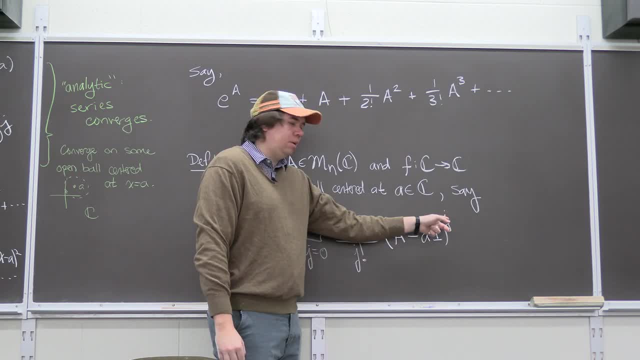 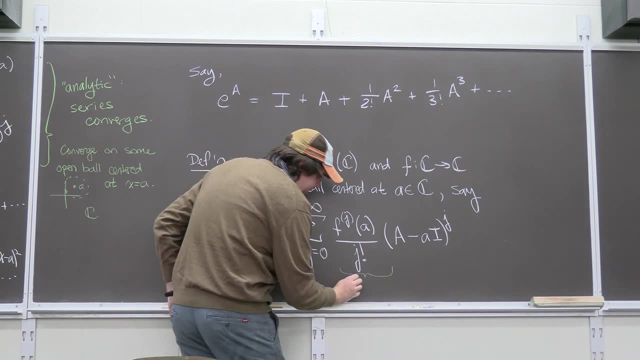 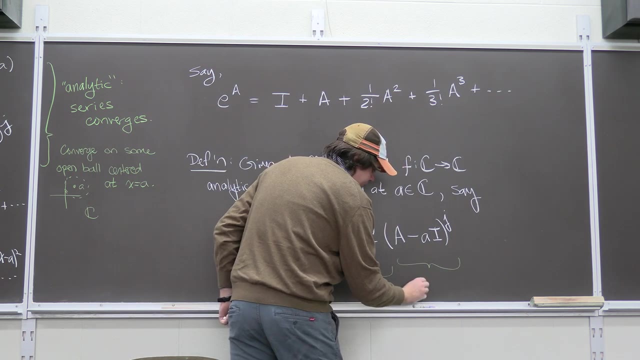 So this is just a matrix. This is a matrix to some power times by a scalar- Right. So this is just a sum of complex scalars, times, powers of matrices- Right. So this is what we're going to do, Right. 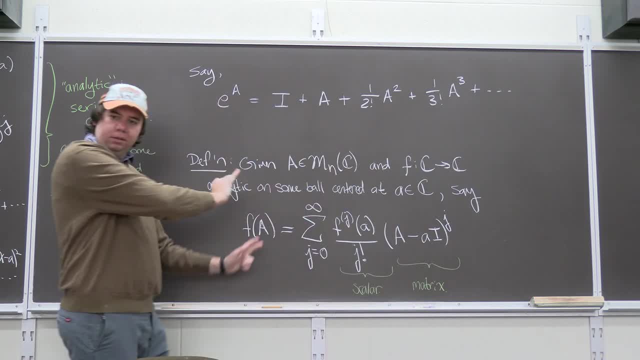 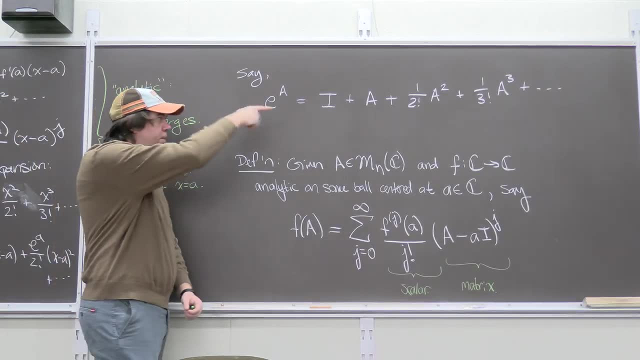 So this is what we're going to do, Right? So this is what we're going to do Right, Right, Right, Right. well-defined, This makes sense, right? Okay, Just like above, we would define e to the: 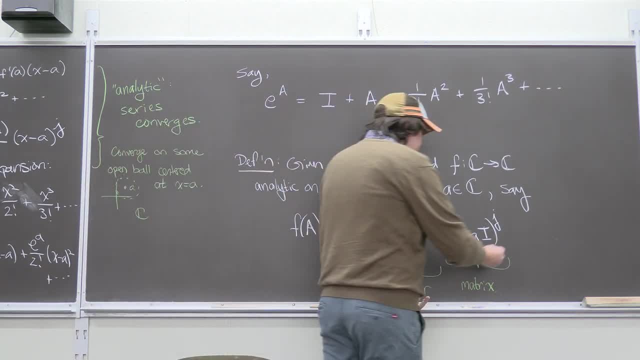 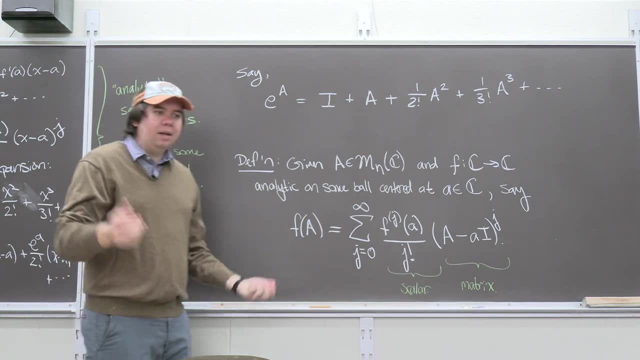 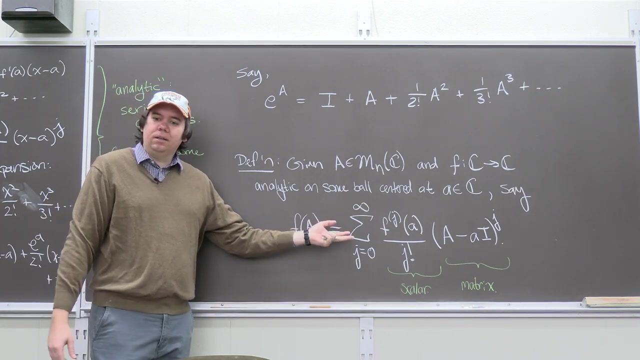 a to be this thing. Okay. when you write something like this, like you might remember from Paraclose 2 or whatever analysis class you've done, it's like the big worry you now have are worries about convergence, Like worries that this thing is well-defined And, if you like, pick. 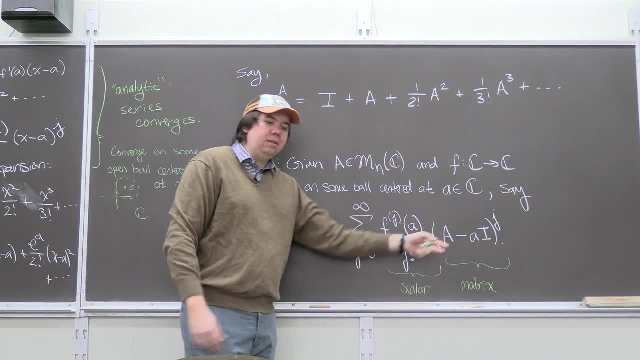 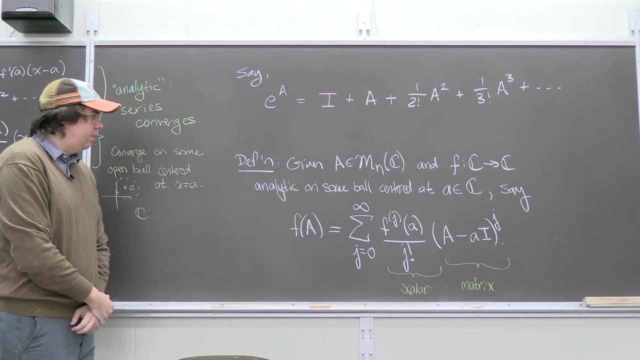 different a's, for instance different scalar a's, that they converge to the same thing, right? So these are the kinds of worries you have in an analysis course. I don't want to worry about that too much because you know there's a reason I don't teach an analysis. 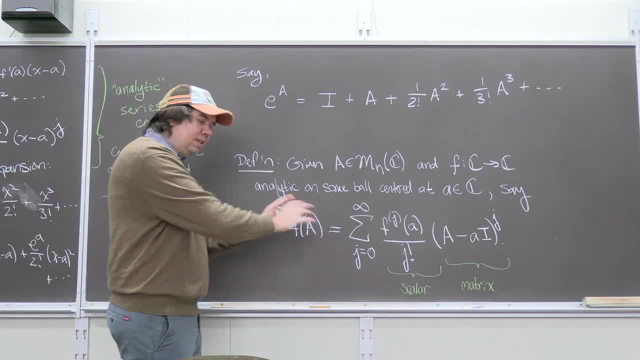 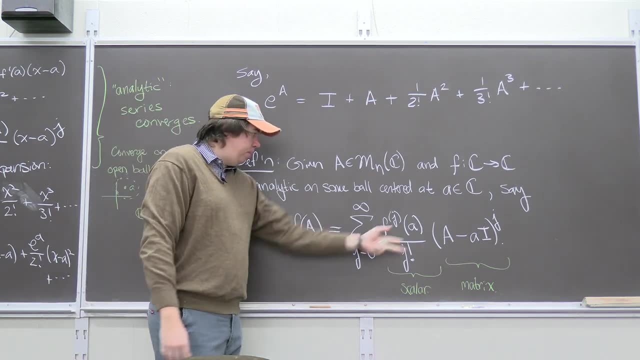 course I don't like that stuff right, But like, that is a worry you should have. And so in a couple minutes, what we're going to transition to is we're going to give some better formula for this right And we're going to see like, well, once we have a precise 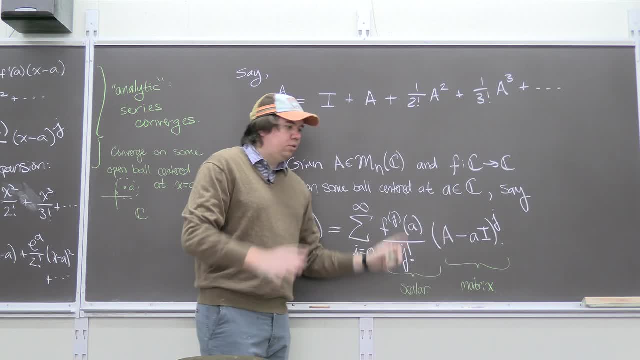 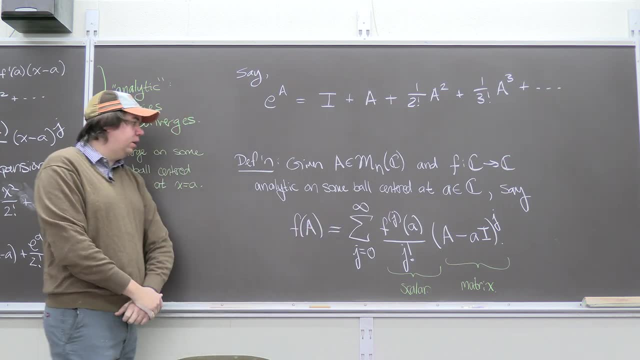 algorithm. it'll be actually independent of your choice of a. So regardless of which point you pick, as long as it converges, it will converge to the same thing, right? So we'll address that worry that you might secretly have. But we really do need to do that because, like 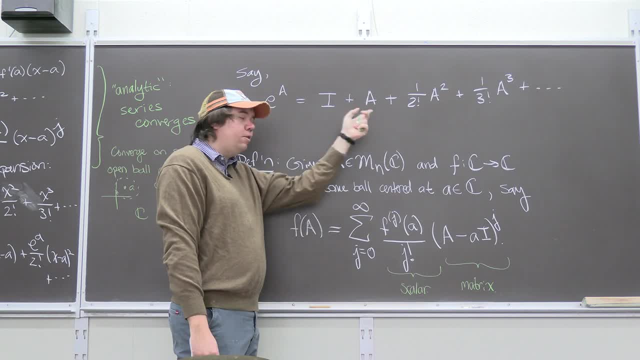 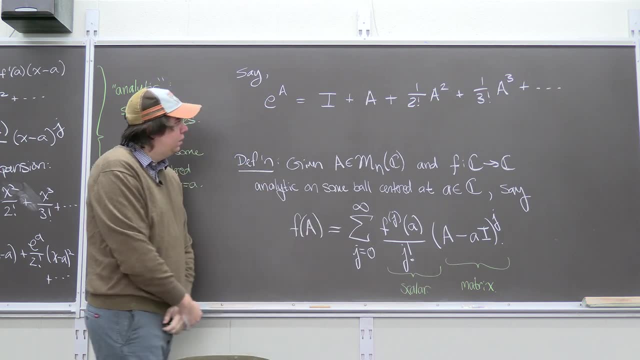 right now, although we've given like a definition for e to the a, it's like: how are you going to calculate that thing, right? Like that's a mess. So it's like: good luck, right, There's. 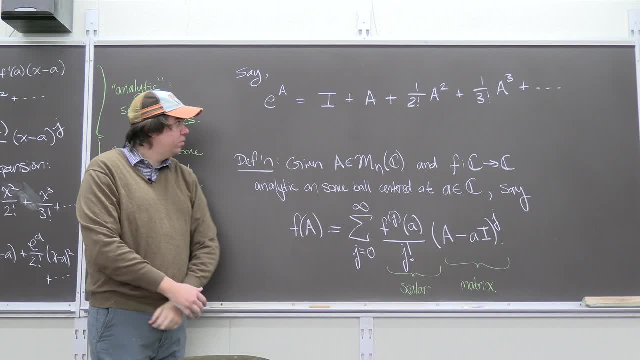 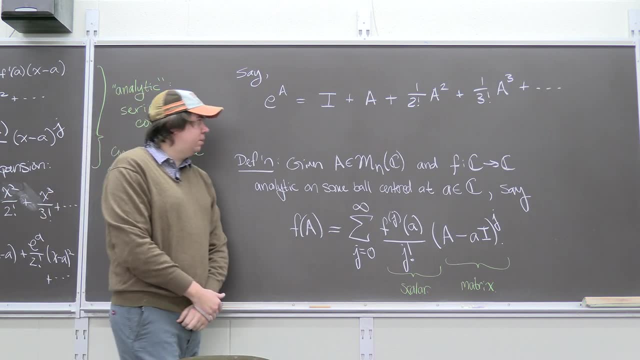 like a lot to calculate, like infinitely many terms. So so we want some better way to to like actually determine what e to the a is And, and I don't know, maybe you have some clever way of figuring out some pattern of what the like if, if, 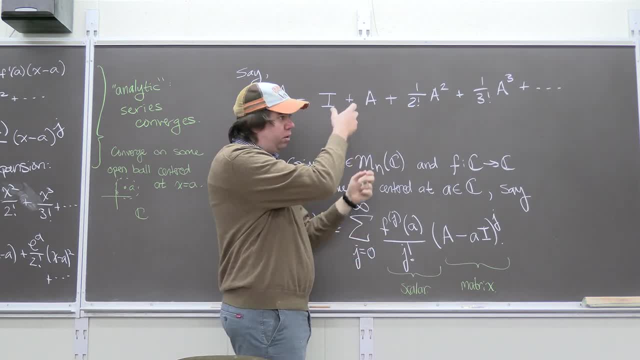 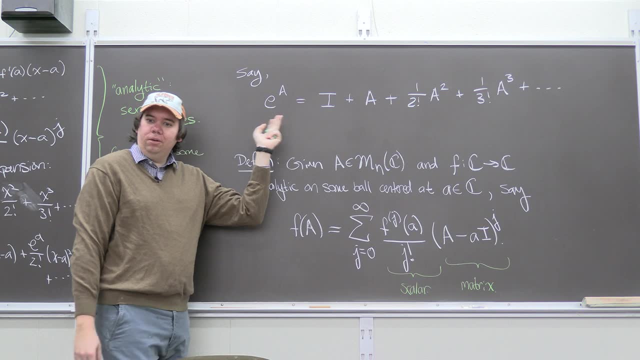 a is like a two by two matrix. maybe you can determine, like the upper left- you know some formula for the upper left value of like a to the n And maybe you could solve this like entry-wise. But in general, like this is very hard to do, right? So so we. 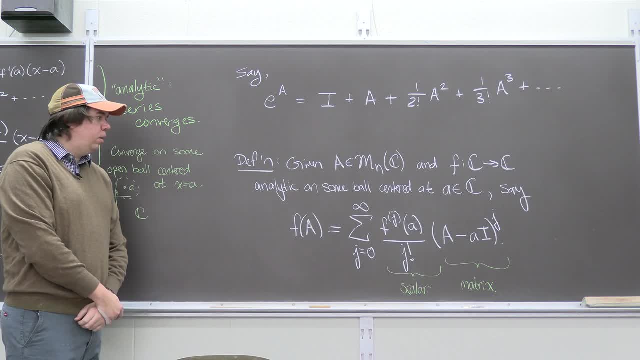 want something that's going to help us. So it's like, well, what's the thing that's going to help us? And you're like, well, what? so we're going to just like think about what we spent the last couple lectures talking. 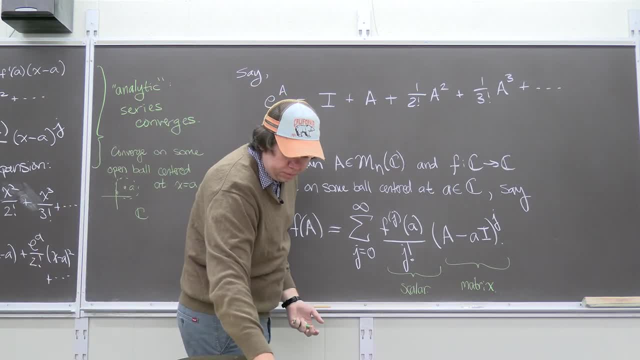 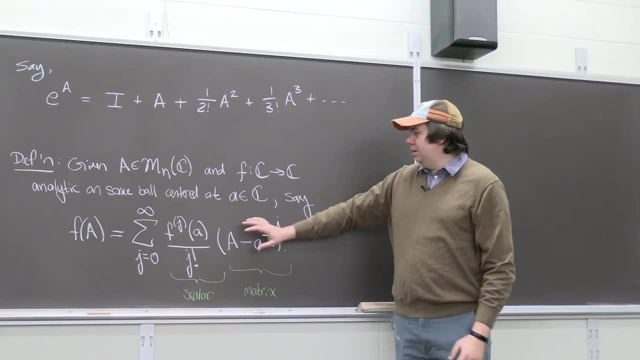 about. Maybe there's a reason we spend all this time talking about Jordan canonical forms, And so what I want us to do is see how thinking about a Jordan decomposition will actually give us a much nicer way to quickly, very quickly, determine what e to the a is with. 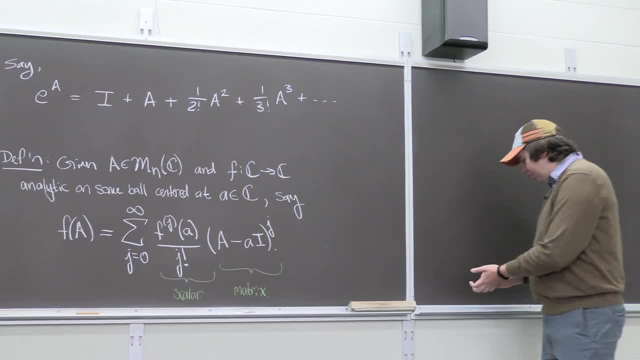 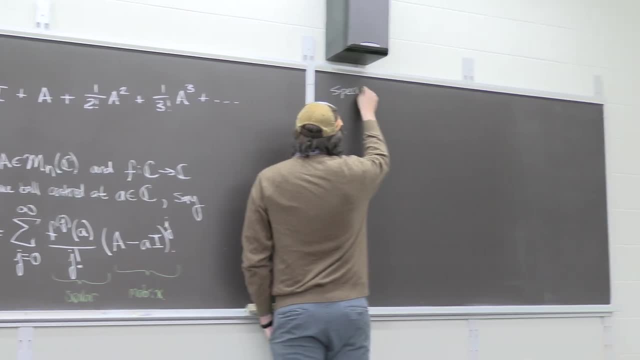 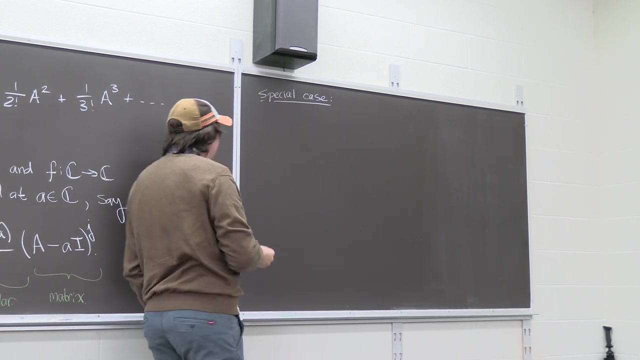 Jordan decompositions. Maybe before I do that, though, before I build up to Jordan decompositions, I want you to think about just a special case, and that's if you have a diagonal matrix. So let's say, we have some diagonal matrix D. 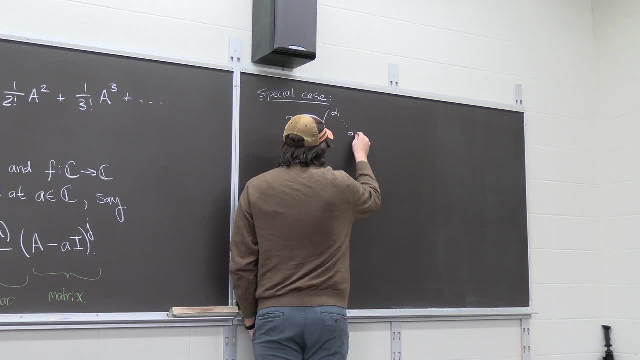 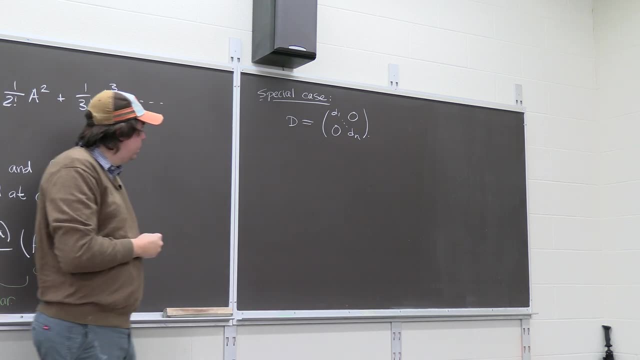 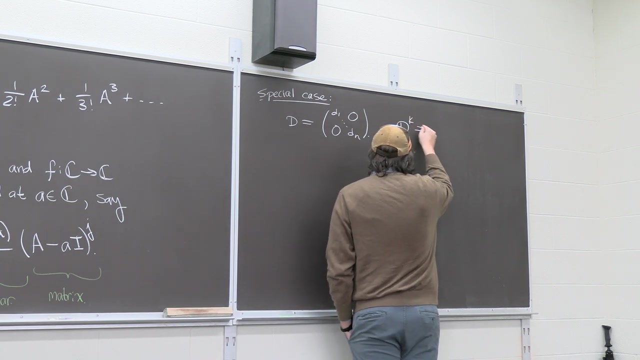 that just has diagonal entries, D1 down through, let's call it DN. Let's say we have a diagonal matrix, right? Okay? well, what are the powers of D then? The powers of D, like D to any power, just comes out to be those diagonal entries to that power. 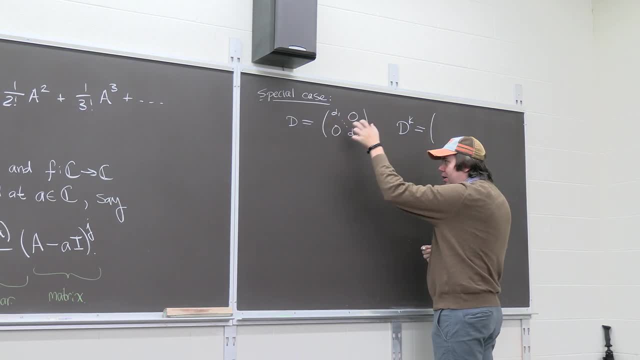 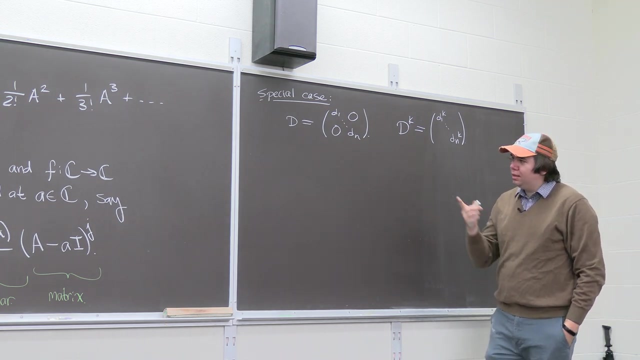 Because when you multiply them by itself, you just get the D1 times D1, the D2 times the D2, and so forth. So this is just D1 to the K, down through DN to the K, And so let's try and think about an example. 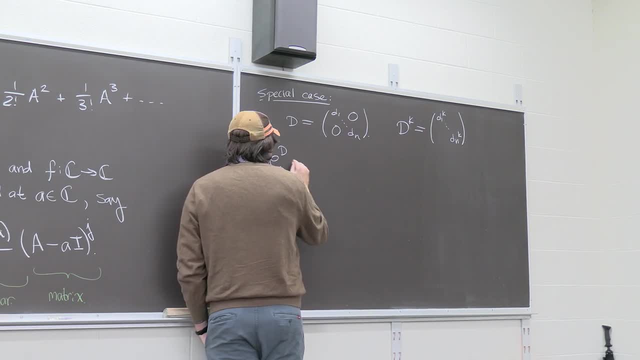 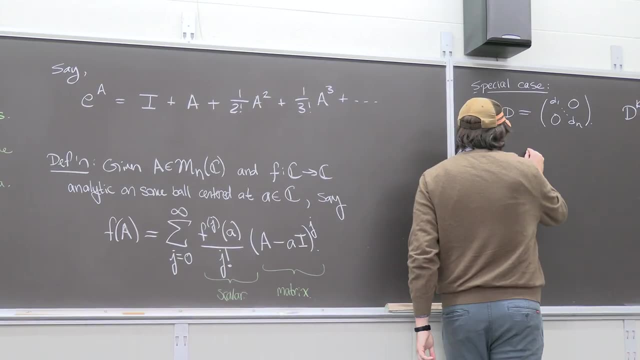 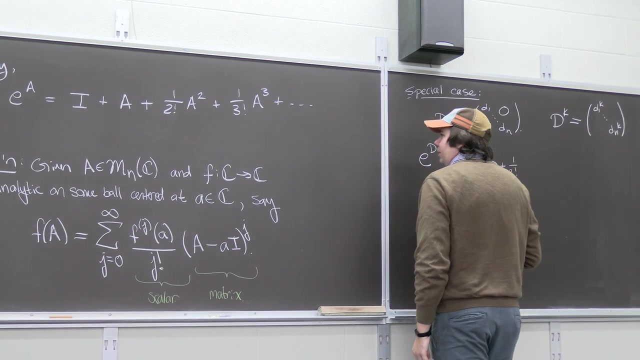 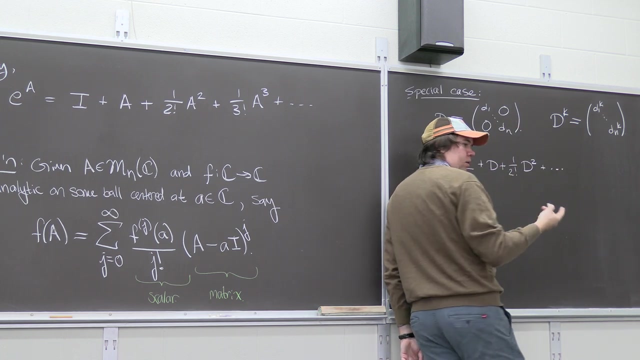 of something like: if you have E to the D, Well, you could write that out like here, where you're like: this is just identity plus D, plus one over two factorial D squared, plus one over three factorial D cubed, and so forth. 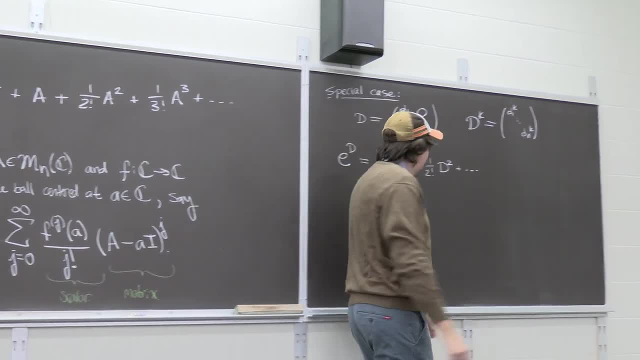 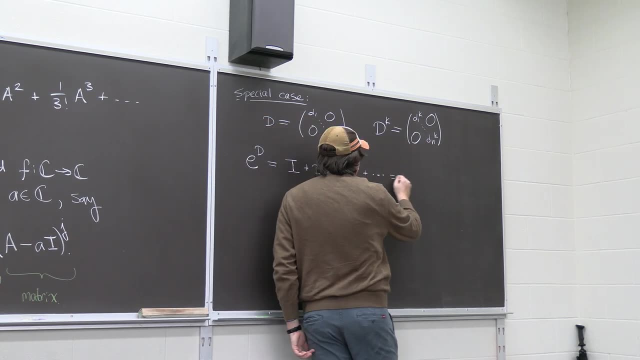 But now your powers of D are really well-behaved things. It's just your diagonal entries to whatever power. Okay, And so if we want to represent this whole thing as a single matrix, we know what's going to happen in the entries. 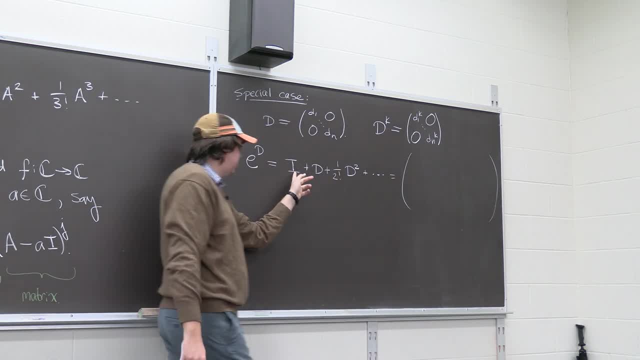 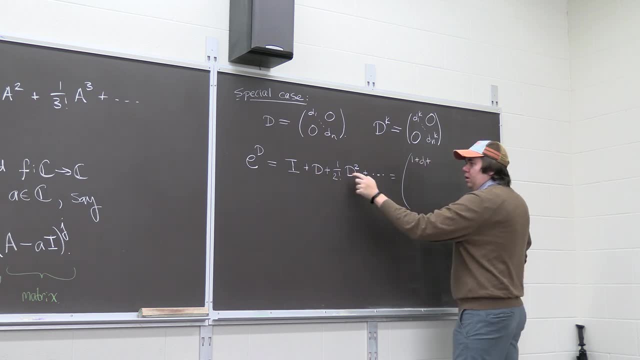 The top left entry. this time we actually can do it. Identity is just going to contribute a one. D is just going to contribute a copy of D1.. This is going to contribute a copy of one over two factorial D1 squared right. 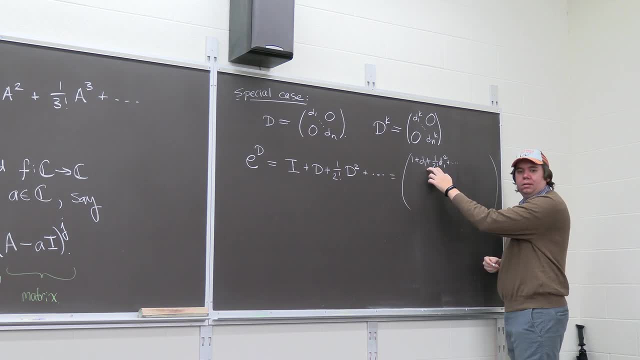 And you exactly get the series expansion with just D1 plugged in. Or if you think about the lower right entry, you'll have one from the identity, plus a copy of DN, plus one over two factorial DN squared so forth, And so your diagonal entries just become. 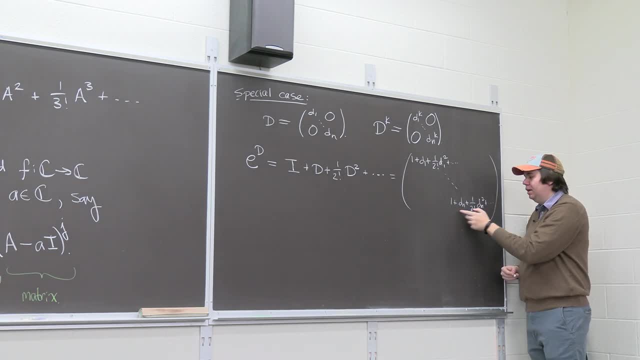 the series expansion at the DK, D1, D2, D3, down through DN and zeros everywhere else. But it's like: what is this? What is that guy right there? E to the D1? Yeah, that really is just E to the D1. 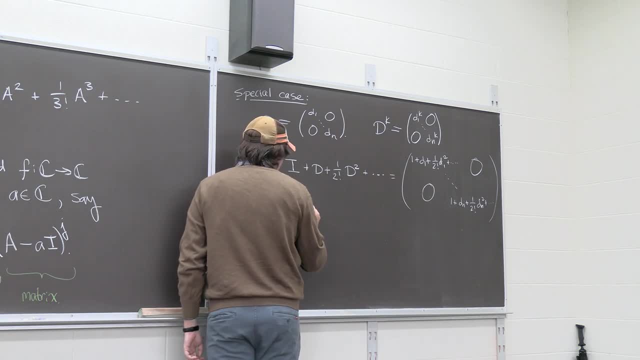 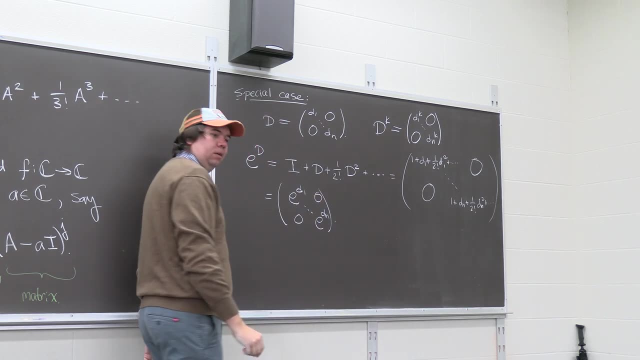 So here it really does just come out to be E to the D1 down through E to the DN on the diagonal and zeros everywhere else, And so it's like, okay, so for a diagonal matrix you really can just do E to the diagonal. 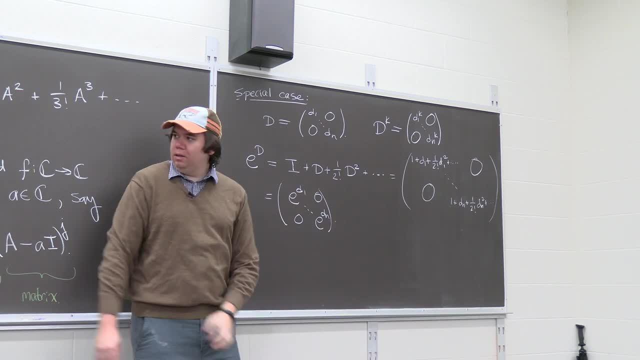 is just raising each of those values E to that value, right? It's like the thing that you want to do with a matrix be like that was too dumb. Well, it's not too dumb when it works. It's because it does work for diagonal matrices. 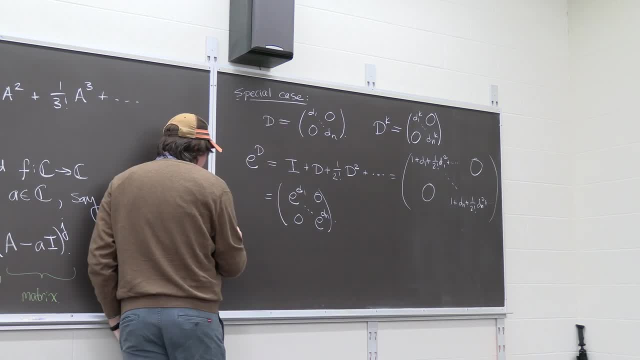 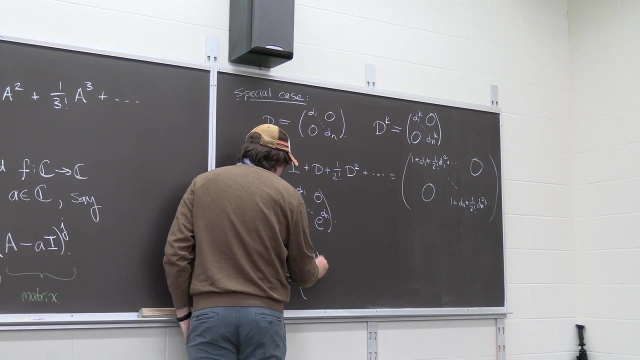 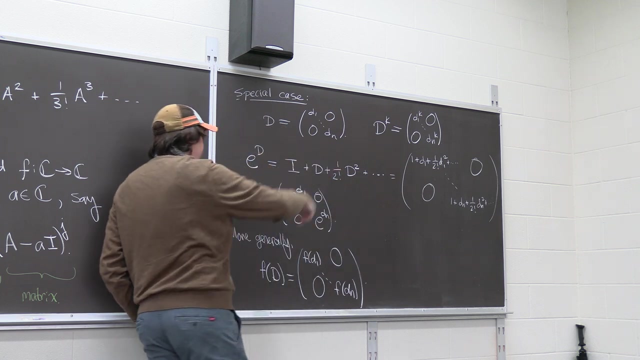 cause. that's exactly the powers of diagonal matrix work. And more generally, if you have some analytic function, F, F of D- just comes out to be F of D1, down through F of DN zeros. everywhere else It's the exact some argument. 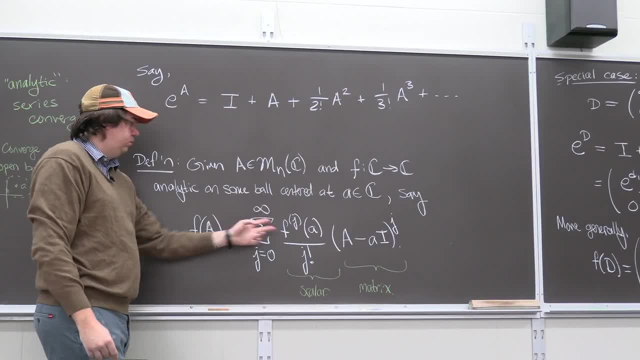 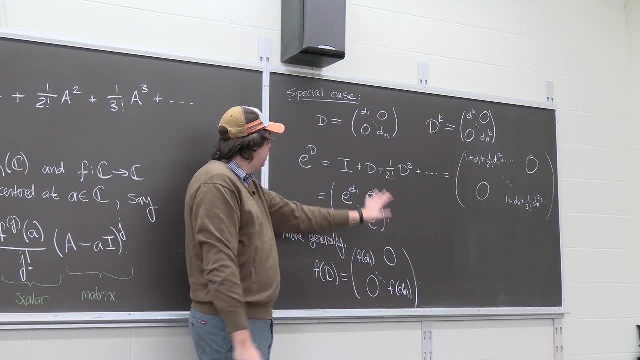 but you just do it in general with, you know, this Taylor expansion for whatever F, whatever F's Taylor expansion looks like right. So you're like okay, so diagonal matrices are really nice, Right, like those are really nice to play with. 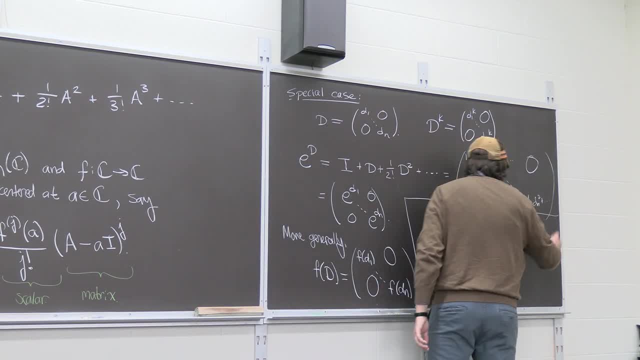 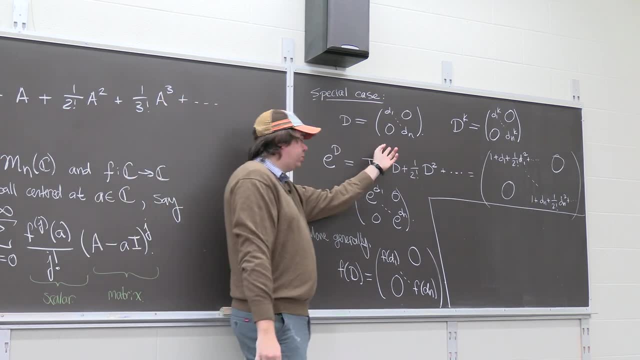 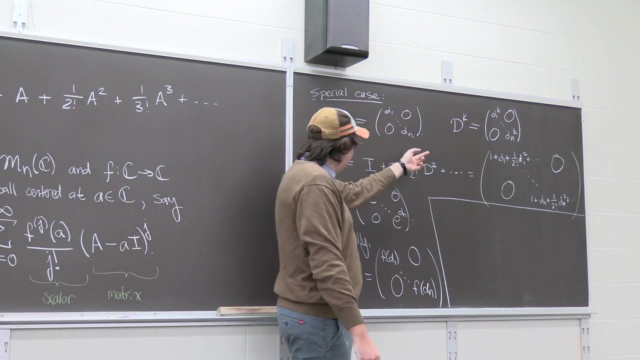 But we're interested. well, it's like the problem is not all matrices can be expressed as a diagonal matrix. Not all matrices are similar to a diagonal matrix. That's why we have this whole Jordan canonical form, where we write things that have a diagonal. 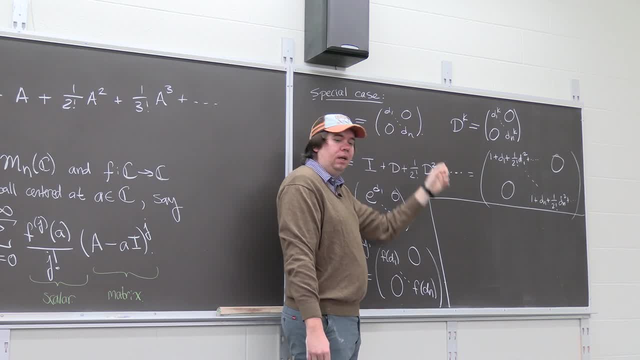 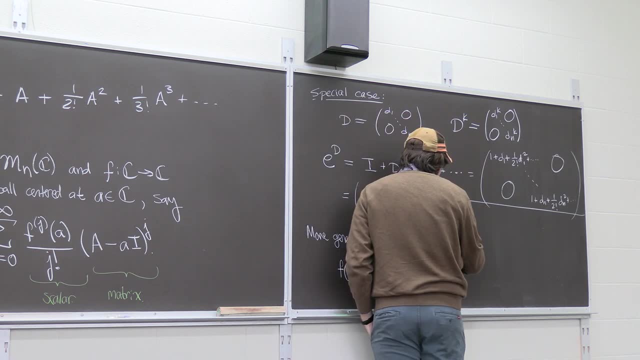 but then we also have a super diagonal with ones right, And so what I want to do is take a second to think about just what happens to these powers. what happens to these powers if you have some matrix that has a super diagonal of ones? 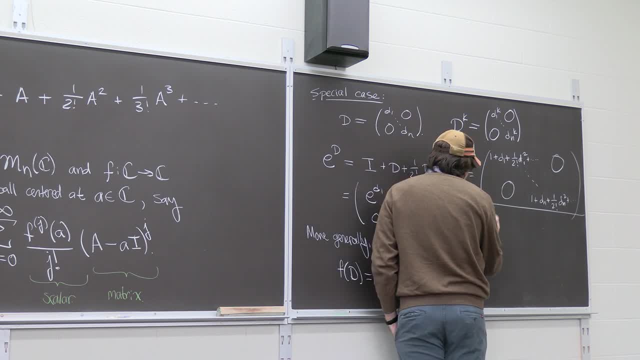 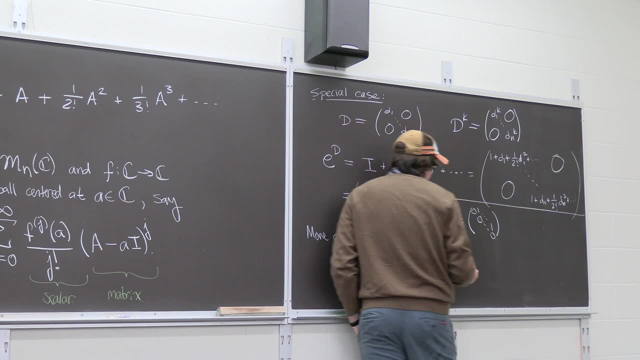 And so, for simplicity, I'm just gonna make my diagonals all zeros. This is like the simplest case we can do: the diagonal is all zeros, And then I'm gonna have your super diagonal of all ones. So here I just have ones. 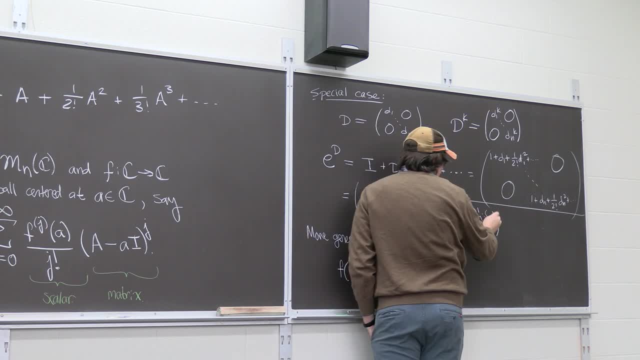 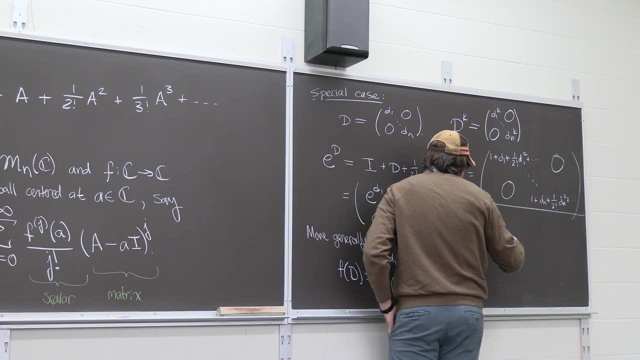 which is just one above the diagonal right And zeros everywhere else. So this is my matrix. N, Let's say. this is like a, I don't know, a K by K matrix, I'll call it, or an N by N matrix, or whatever size I want this to be. 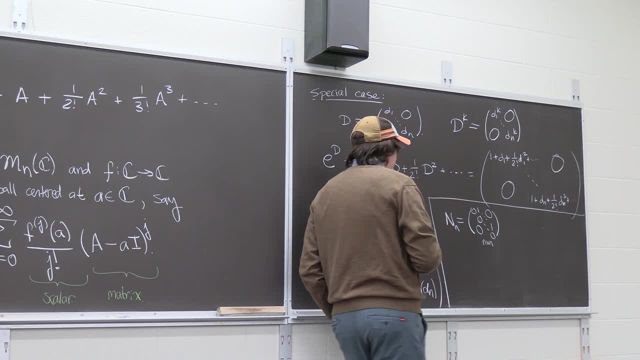 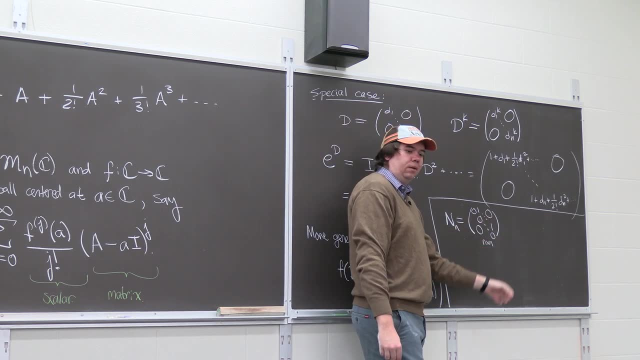 Let's call it an M by N matrix, So maybe I'll denote this like N sub N. So this is just the matrix of ones along the super diagonal. So let's just think for a moment. This is gonna get a little bit messy. 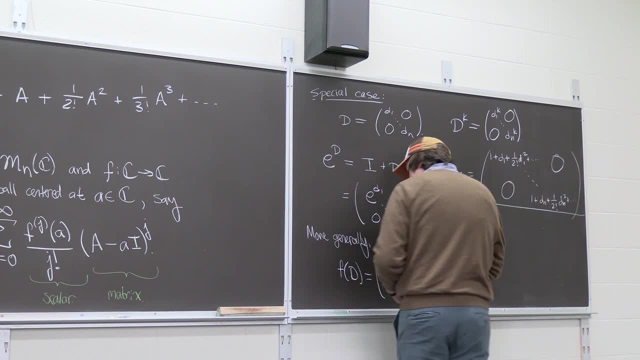 I think I should do a concrete example. Let me do N four. I think that'll let you really see what's going on here. So, like, let's do N four, Let me draw a four by four matrix that has ones on the super diagonal. 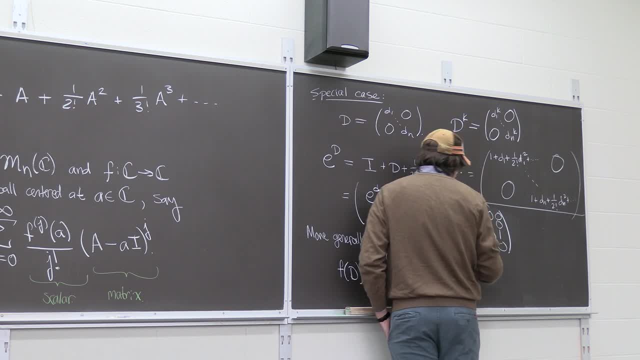 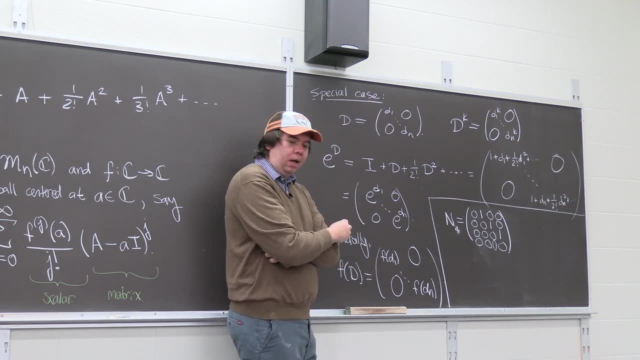 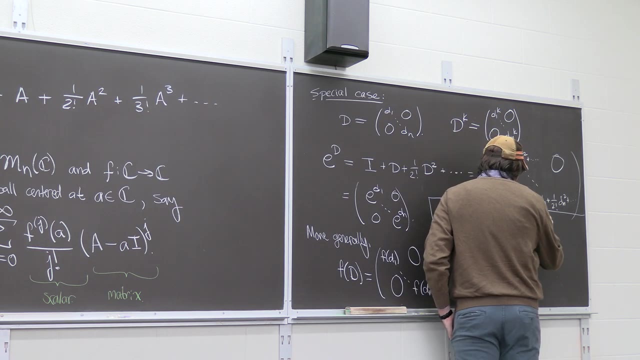 Okay, missed one. There you go. That one's kind of skinny. Okay, let's think about what happens when we square this guy. What is N four squared Right? if we get some intuition about this, maybe we can get some intuition of what happens. 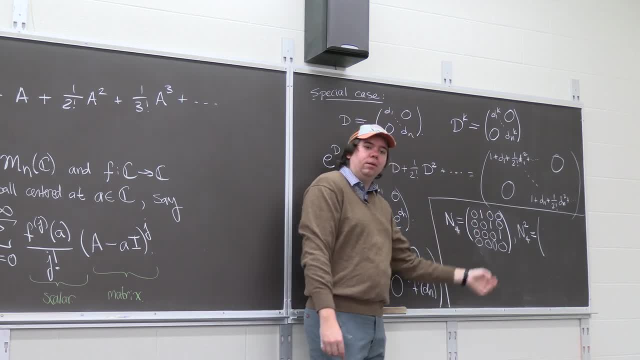 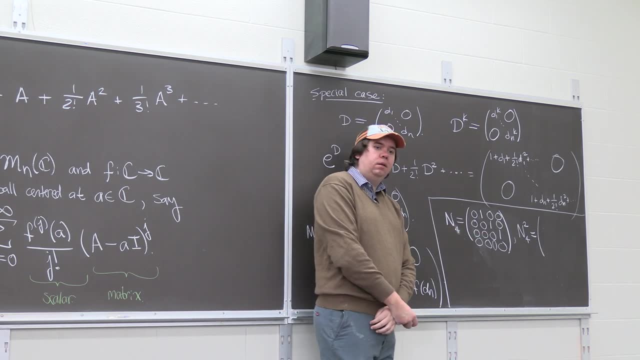 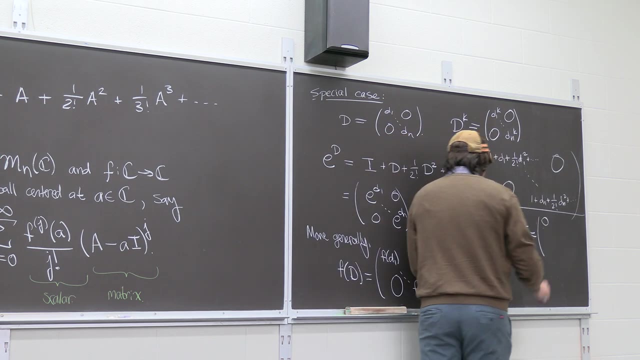 when we have a matrix that's both diagonal but has some extra stuff on the super diagonal. That's what we're trying to build up to. So help me out. What would N four squared be? It would be the opposite. It's like row times, column, that's just zero. 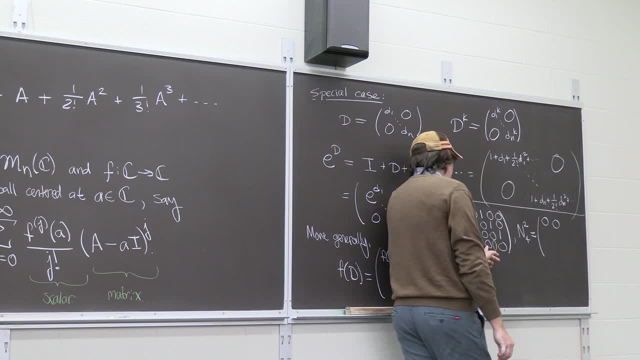 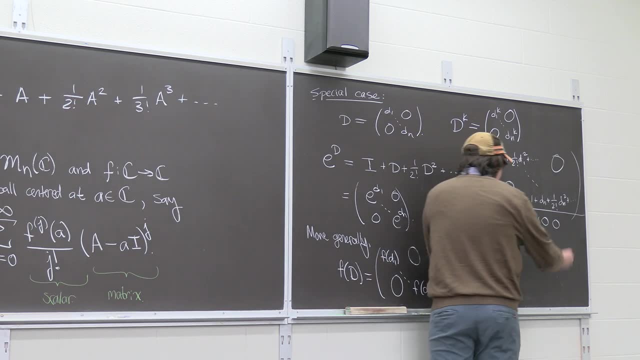 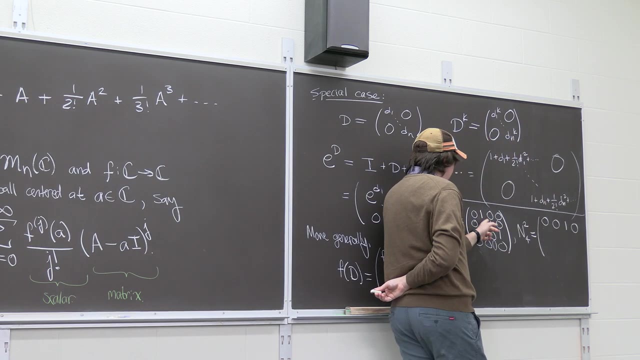 Row times, column that's just zero. But now when you do row times, the third column, you actually get a one right, Because this one and this one multiply, And then row times, the last column is zero. So it's like it's only gonna work. 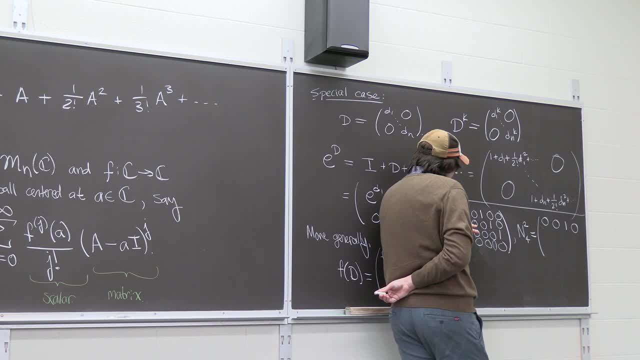 this one And then for the second one it's like: when is it going to be non-zero? Well, if you do a second row, it'll be non-zero when you times it by the last column And all the other times it gives you zeros And everything else gives you a zero right, Like. 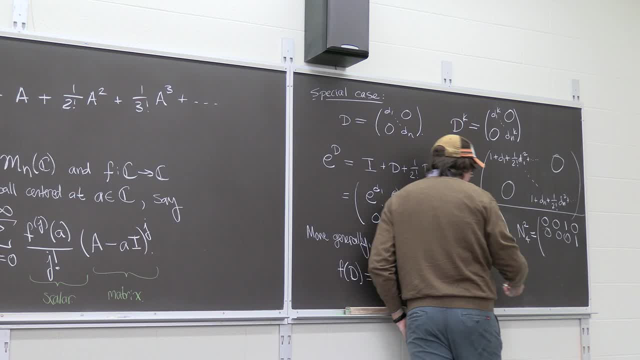 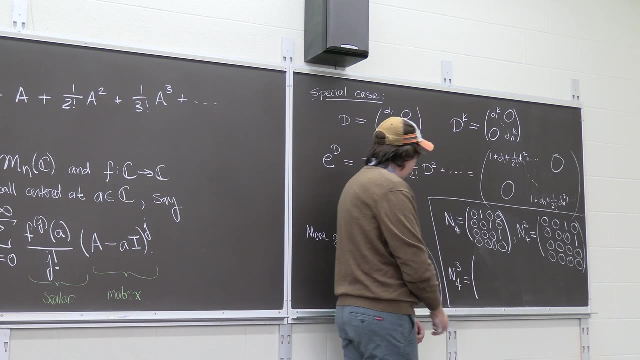 this guy. it gives you zeros in times of any column and so forth. Okay, how about we do like n4 cubed? Well, now I want to do a copy of n4 times, a copy of n4 squared. So here we go: Row times, column zero. Okay, a lot of times it gives you zeros And everything. 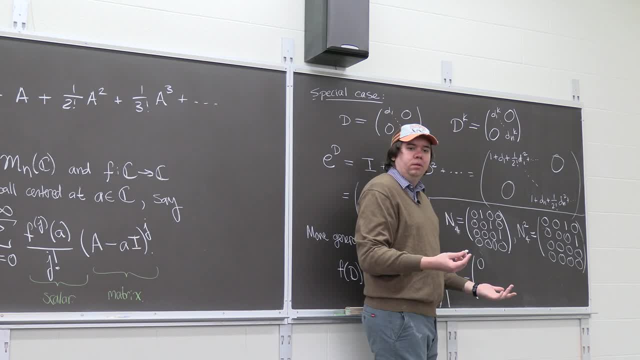 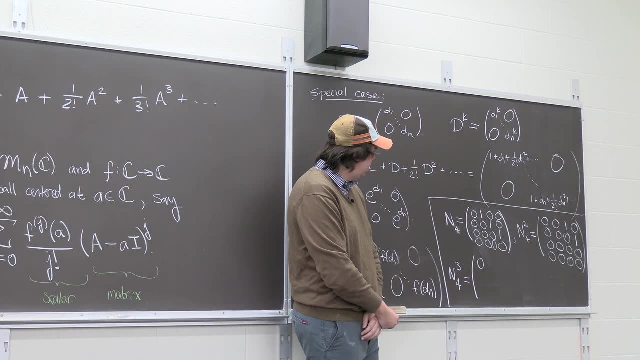 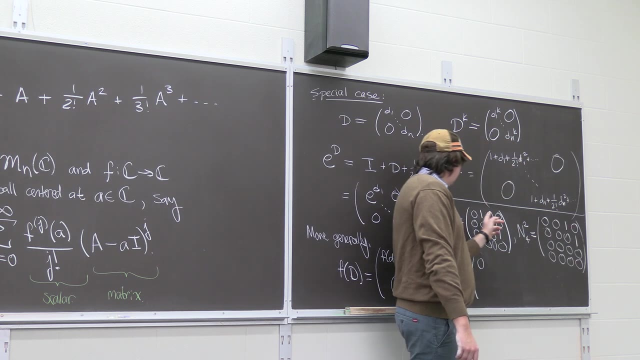 else gives you zeros. Is there any time it's not zero on the top row? Or is there any time at all when this is non-zero? When, Yeah, if you do, the very top row times the rightmost column, this one and this one line up So we get this, But anywhere else you get zero. 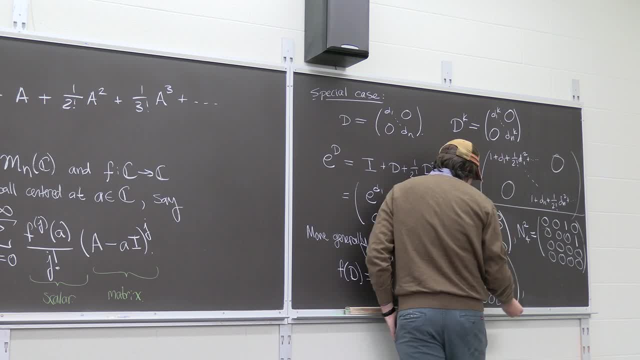 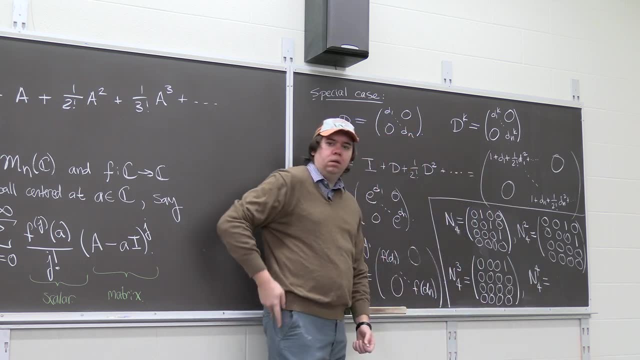 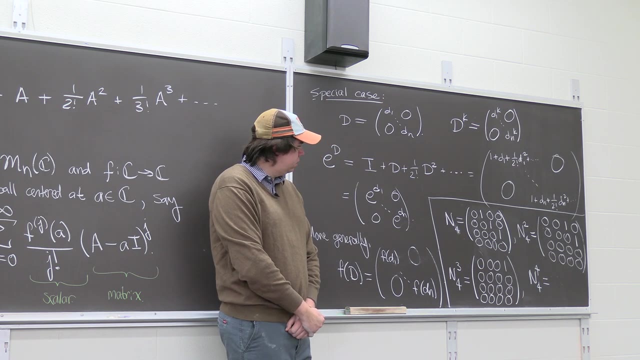 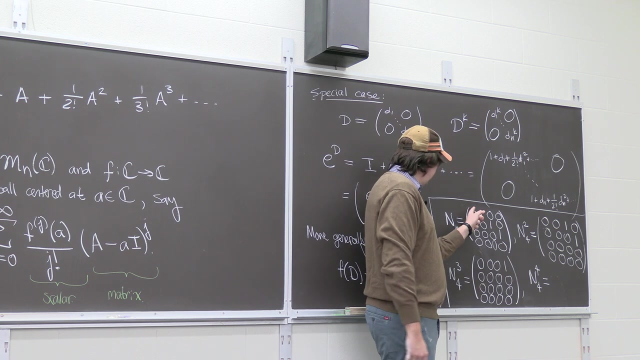 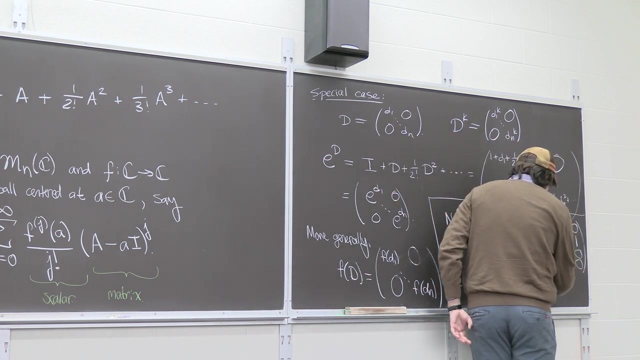 Okay, how about n4 to the fourth? Yeah, like any row times these columns gives you a zero, because it's like this first column is all zero, So there's no way anything times this one gives you a zero, So he just comes out to be zero. Okay, so what's the pattern? 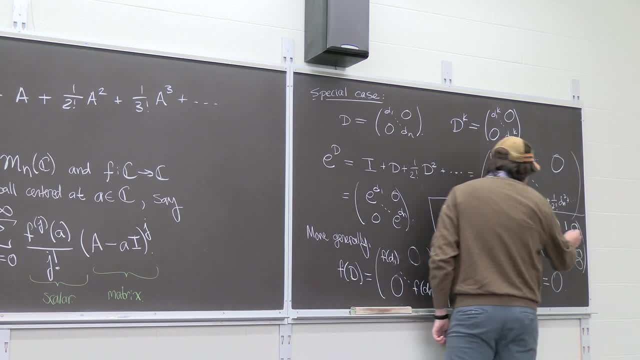 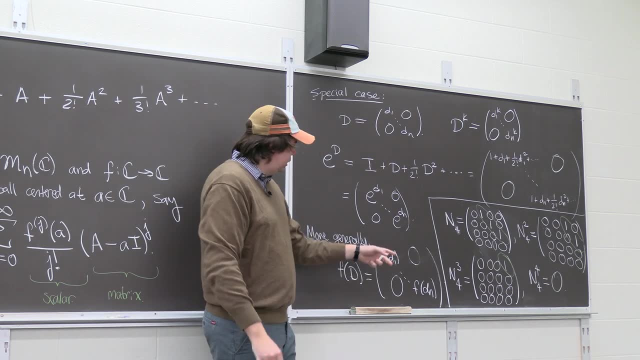 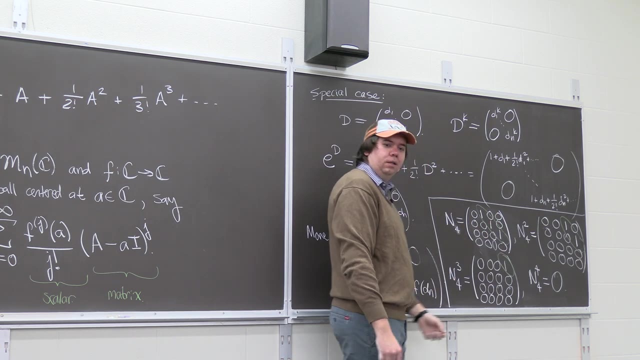 Yeah, it's just. every time you go up a power you're shifting up where this diagonal of ones are, And this holds in general. You can think about it: if you have just a k by k matrix like this, then you multiply by itself. the ones just get shifted up one right. So 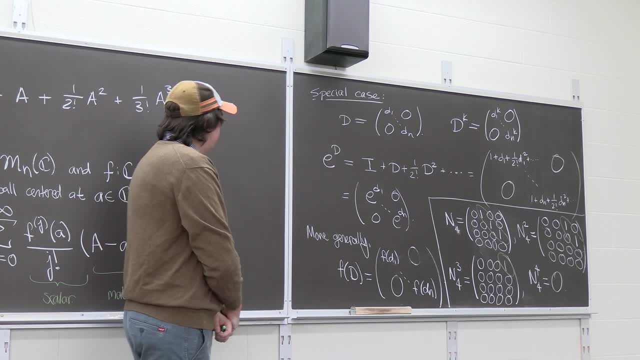 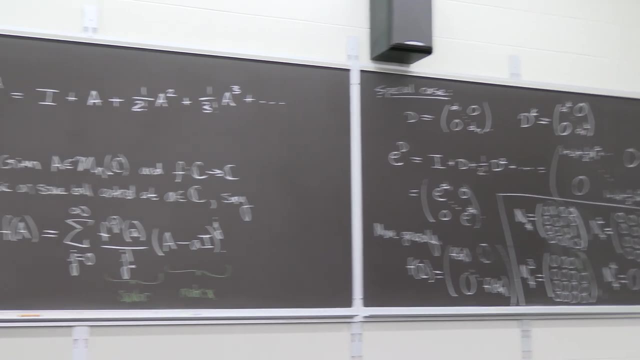 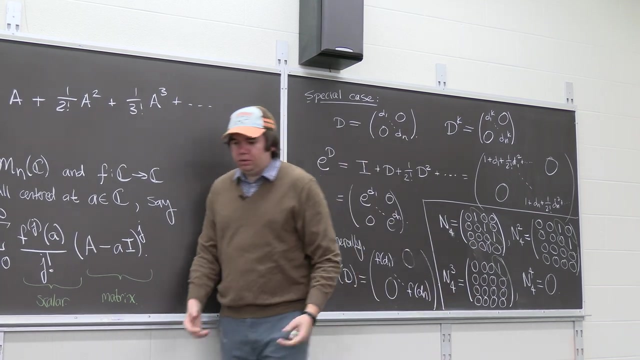 okay, Okay, maybe that's going to help us out now. So what we want to do is we want to try and think what's going on here. if I have some Jordan form, I want to try and put together a diagonal matrix with this n matrix, which is what the form of some kind of Jordan form is, And so let me just 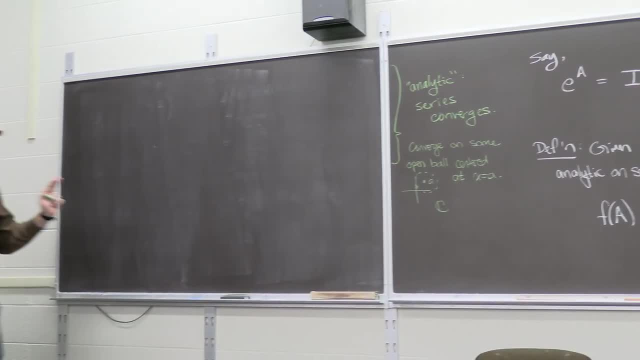 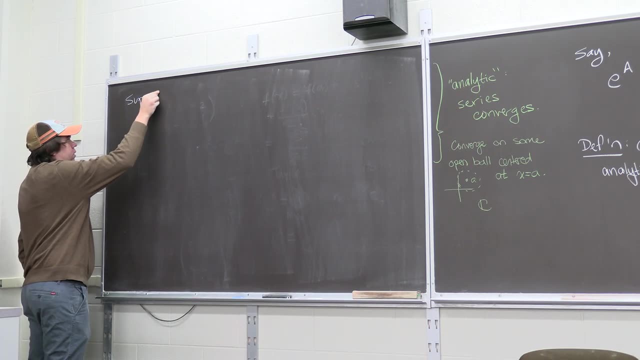 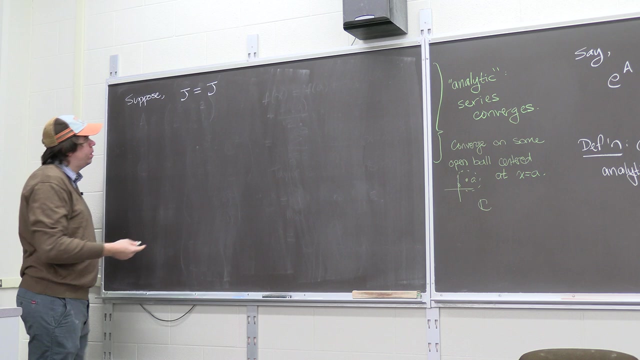 begin with a single Jordan block. A matrix in Jordan form can have many Jordan blocks, But let's just suppose you have some Jordan form. That's just a single, a single Jordan block, And so let's just say: that's j n of. 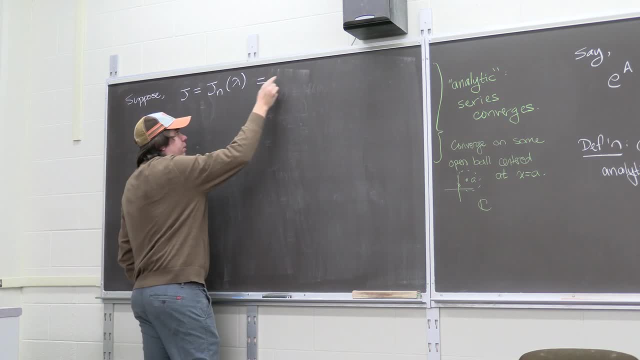 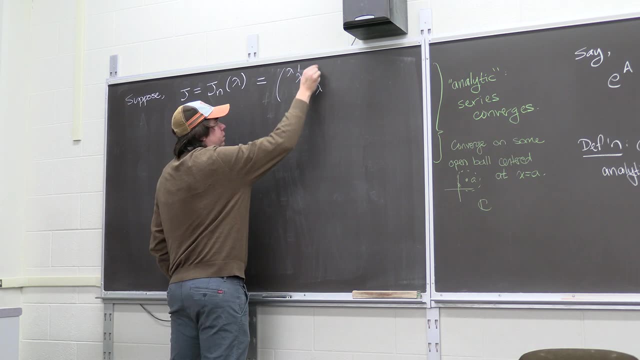 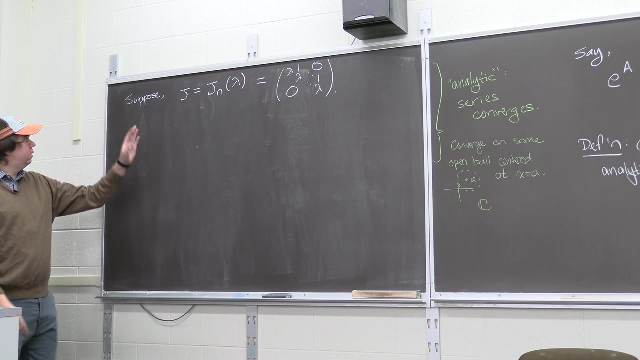 lambda, So like. if you're forgetting what this looks like, I'll just remind you: this is something that has lambdas along the diagonal and that has ones along your superdiagonal And zero, Zero's everywhere else. Okay, so we have just a single matrix of this form And I want to try and 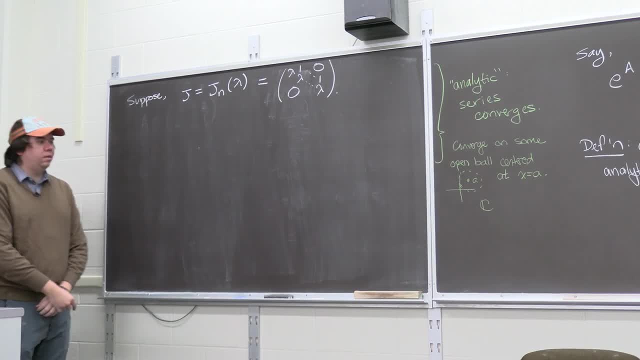 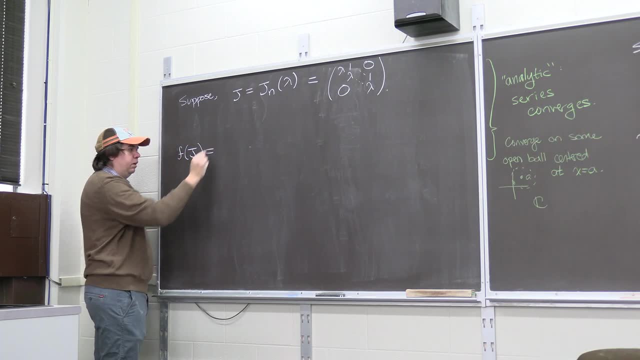 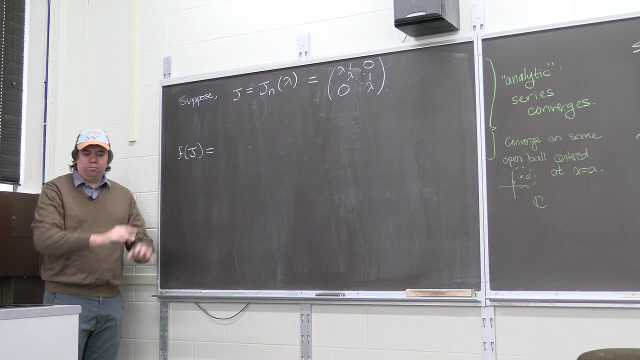 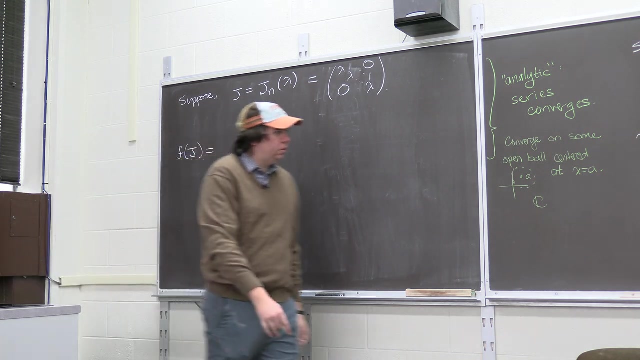 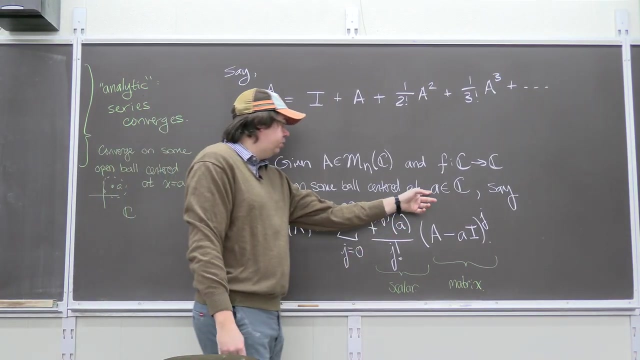 think a little bit about what the Taylor expansion of this is going to look like, And so let's try and calculate f of j where f is some analytic function- Okay, or analytic on some open ball. So it's like let's be a little bit strategic: Open ball centered at a Well like what might be a good 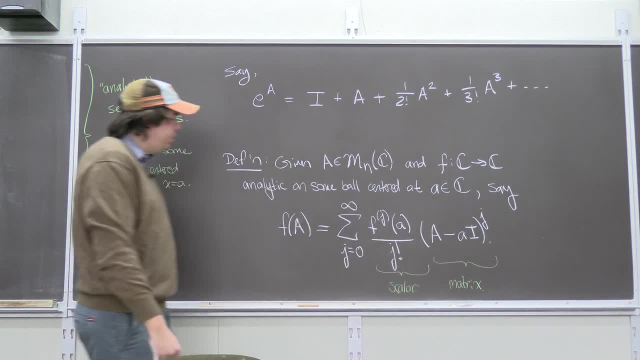 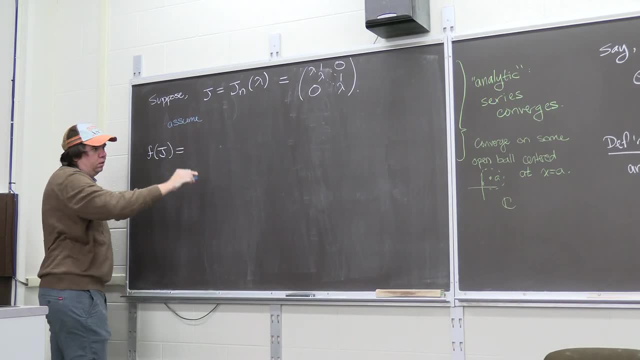 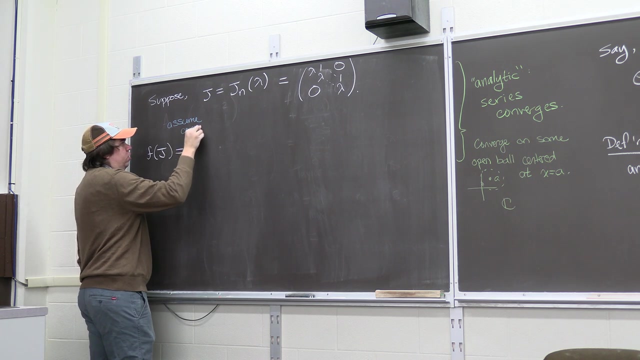 value of a for us to pick. I'm going to make the assumption, we're going to assume, that this is analytic at lambda, That is, it converges For x, equals lambda for your value, lambda in the complex numbers. Because if we pick out a to be, 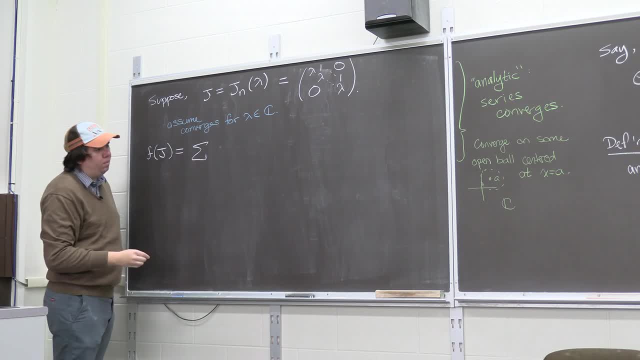 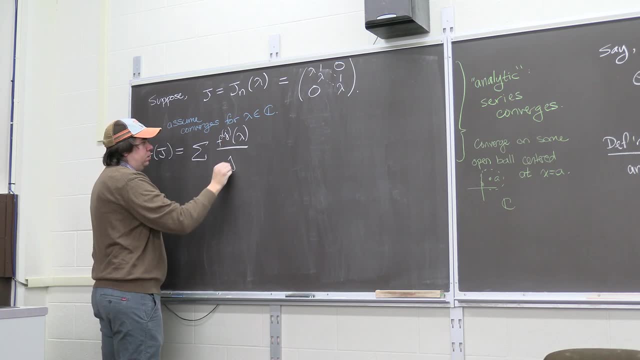 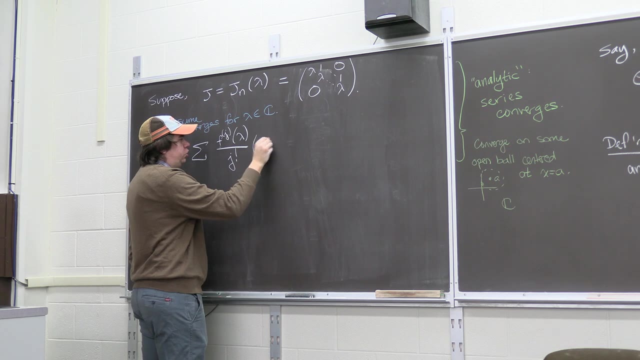 lambda things will simplify quite nicely for us. We'll have the sum of the jth derivative of f at lambda divided by j factorial times, whatever your matrix a is, Which is for us j minus lambda times, the identity to the jth power Where little j is running from. 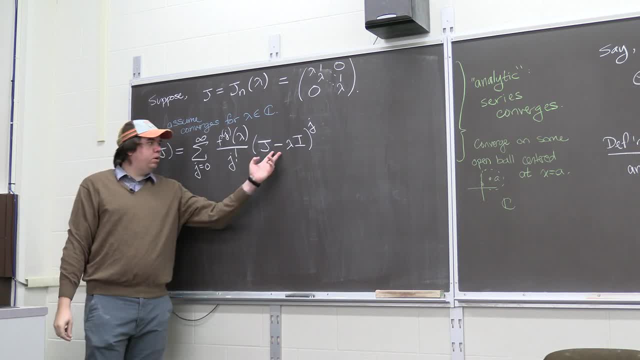 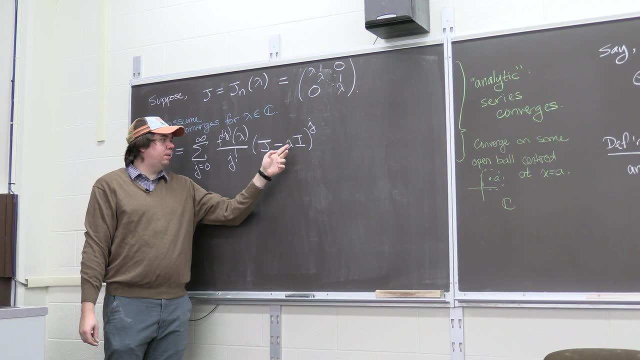 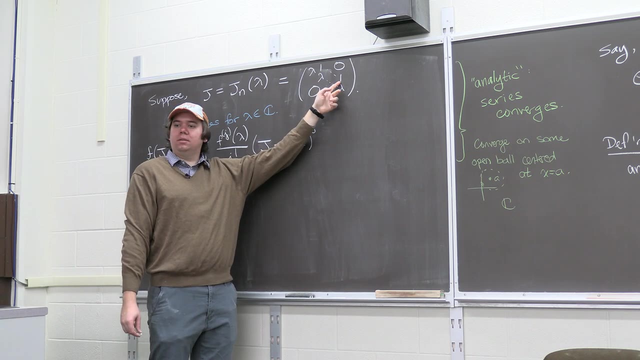 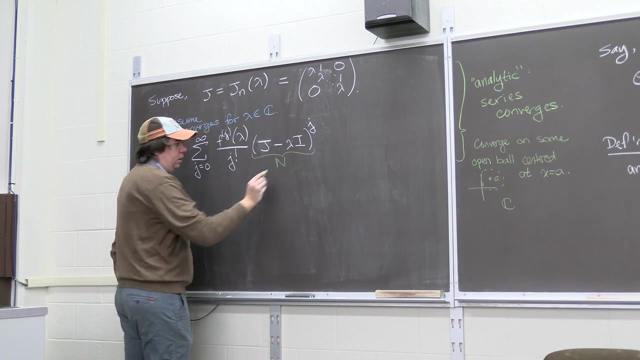 zero to infinity. But notice what happens here: When you do lambda minus j minus lambda times the identity, we're just going to be killing off these lambdas, And so we're left with just a superdiagonal of ones. So what results? here is just some matrix n, An n by n matrix n, just like we had seen And we've already. 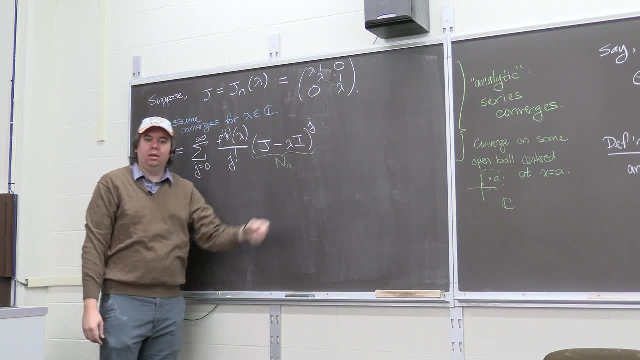 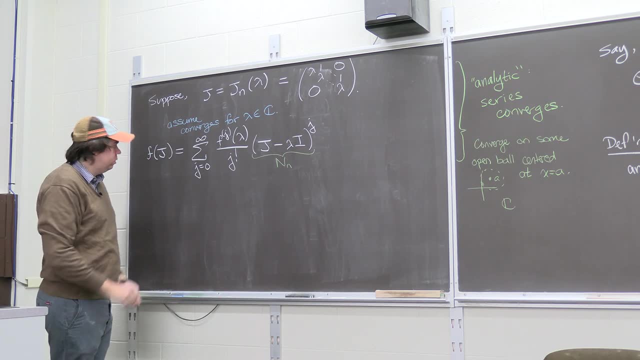 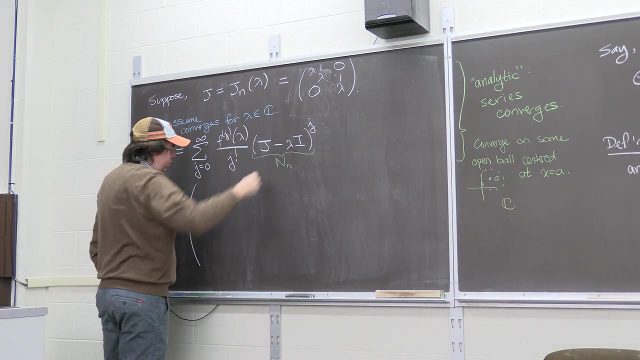 talked about what happens when you raise this to the jth power. You just end up with your diagonal of ones moving higher and higher and higher Right. So let's just like draw a picture of what this is going to end up being. We now have zeros along the main diagonal. 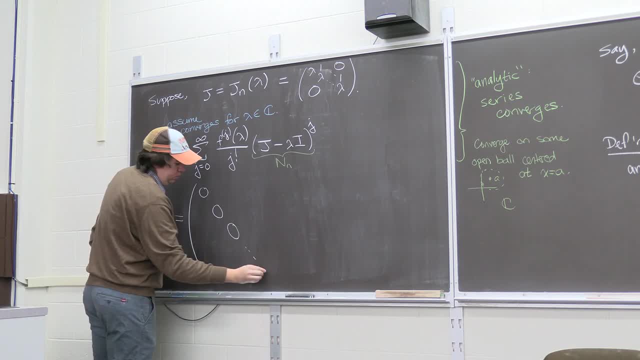 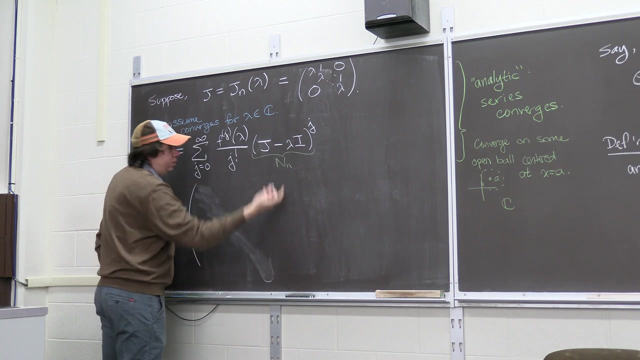 And I have ones on my superdiagonal. So when j equals zero, ah, actually, when j equals zero, what happens When j equals zero? this collapses down to identity. So when j equals zero, I have identity, so that gives me. 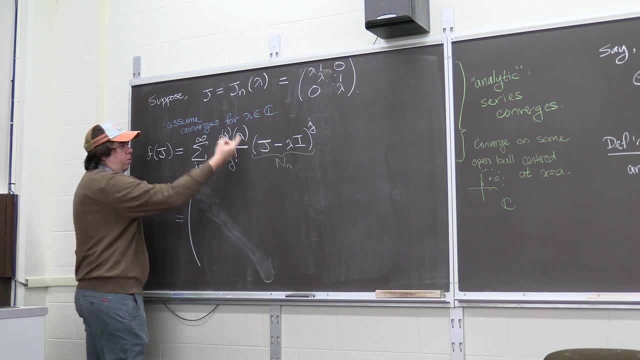 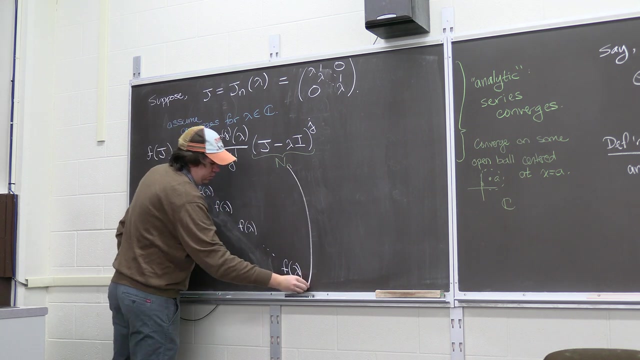 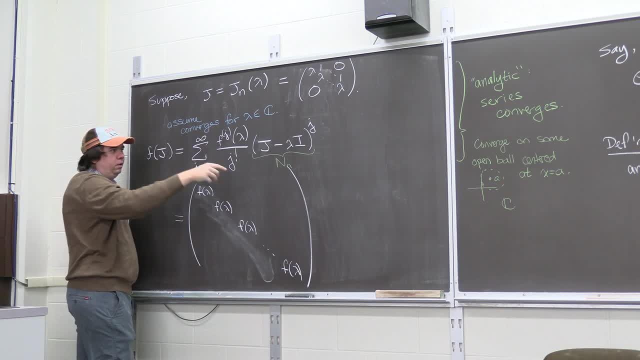 But now let's let j equal one. So what happens when j equals one? Now, this is just ones on the superdiagonal, And those ones on the superdiagonal are getting multiplied by the first derivative of f of lambda, So f, prime of lambda, ends up being on your superdiagonal. 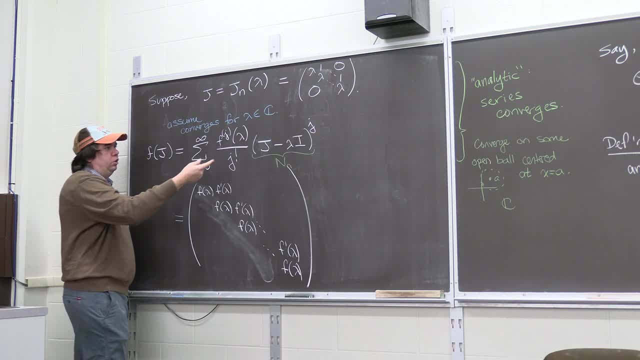 And then it's like: okay, what happens if you have? j equals two, This is squared. so we just set a superdiagonal that moves up one And j is two, so you're doing the second derivative divided by two factorial. 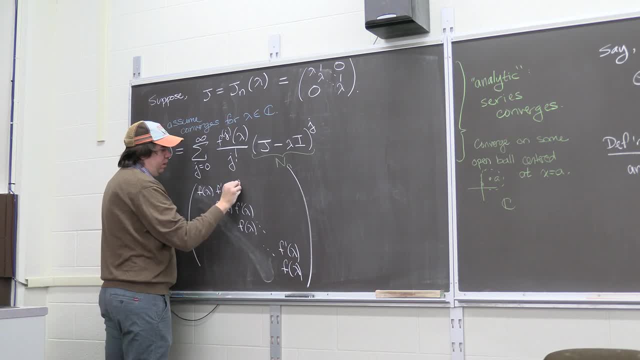 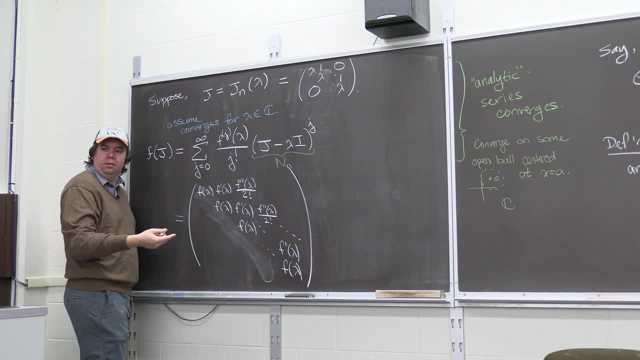 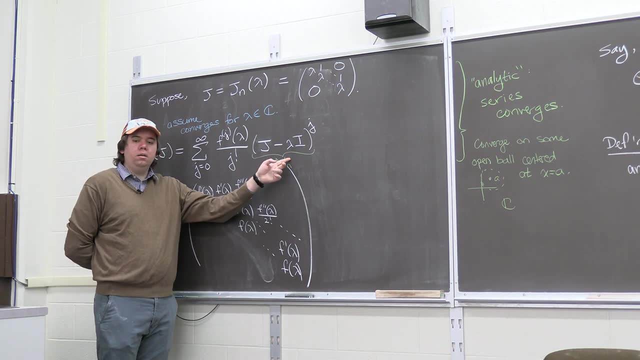 So on the next higher diagonal, you have the second derivative, divided by two factorial, And you just continue this way right Until you fill up your matrix, however big your matrix is, Because at some point, when you get to n. 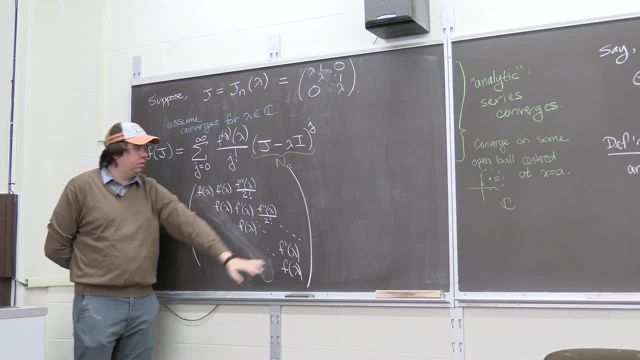 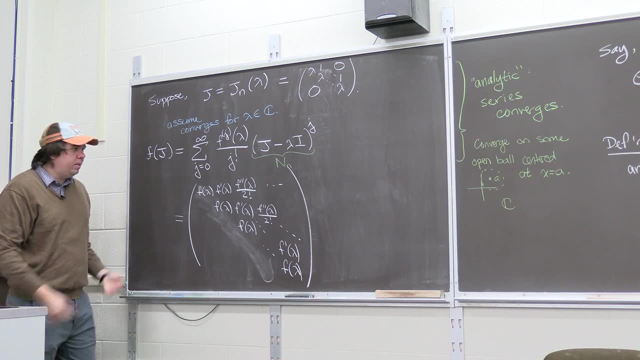 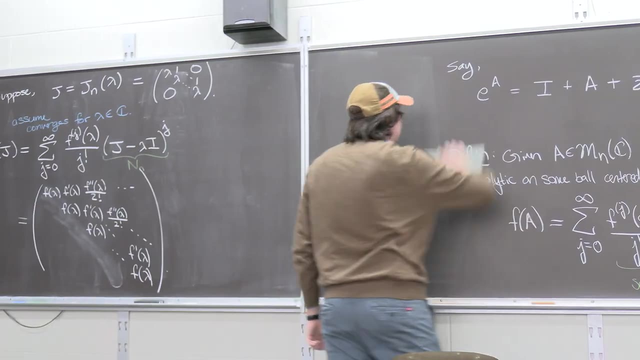 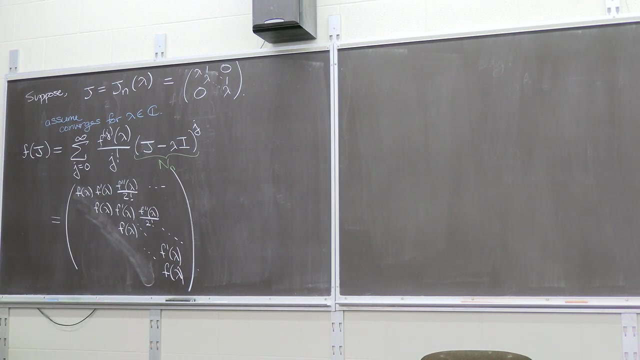 this becomes zero, and then you stop. You're not changing your matrix by anything, and so you just continue this, however large your matrix is. So maybe this warrants an example. So let's pick something for it to be our matrix. J, I don't know. 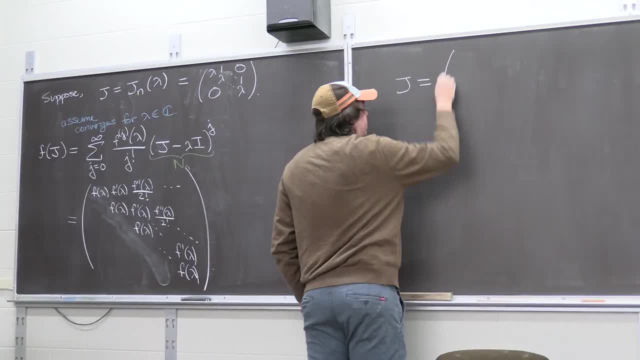 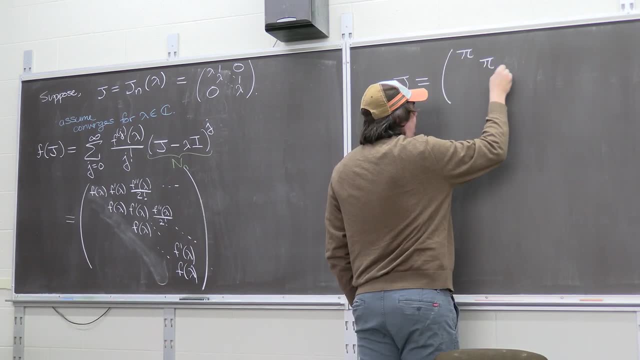 Let's make our matrix J be something like the matrix Let's get pi's, Let's do sine and cosine. That'd be kind of fun. Pi, pi, pi, pi. A four, Four by four, And we'll have some superdiagonal. 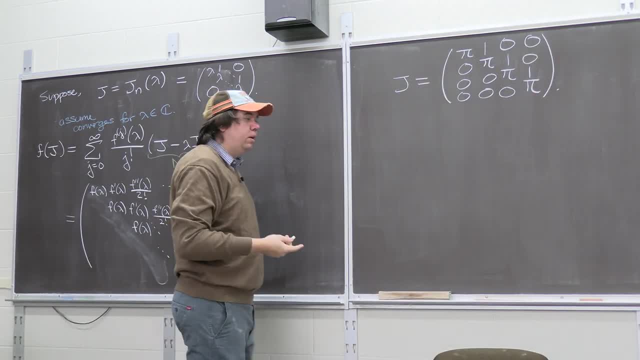 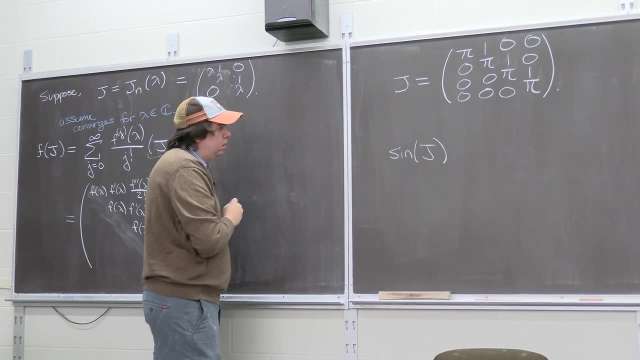 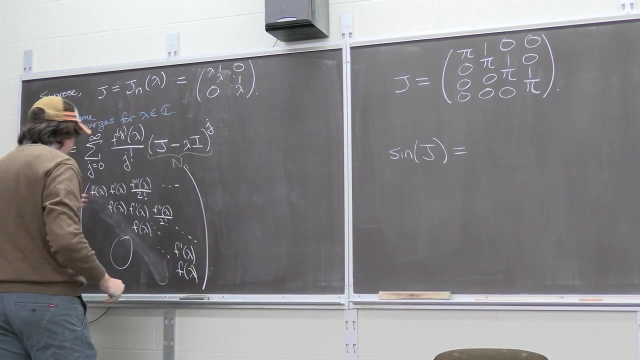 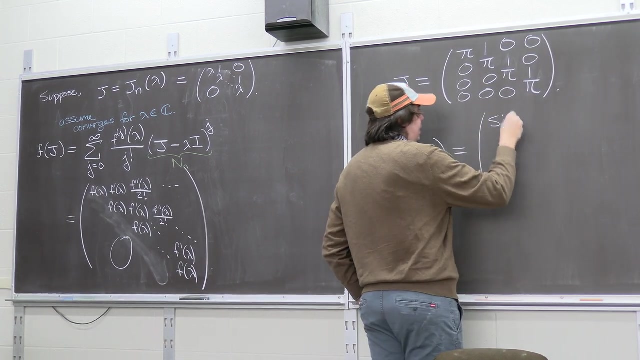 So let's suppose we have some matrix like this And suppose I want to calculate what is sine of J. So we have instructions now: Zero, zero or else. Well, this will come out to be. It's just going to be along the diagonal. 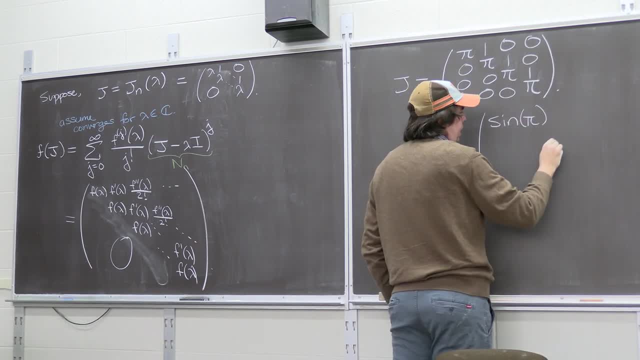 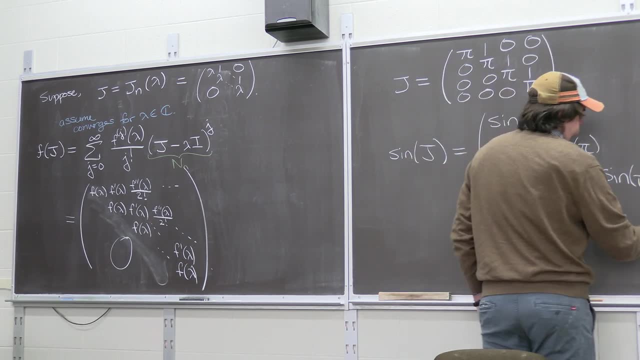 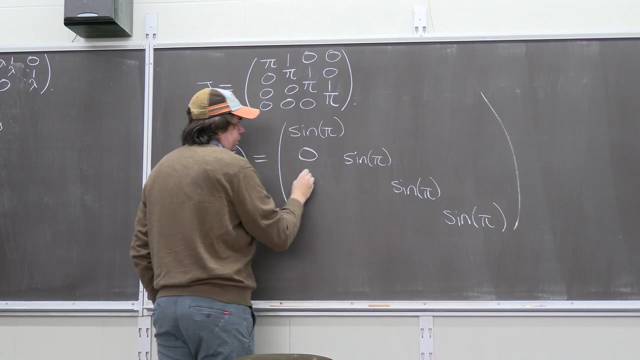 sine of your lambda Sine of pi. So on your diagonal this is just sine of pi. OK, help me out. What is it going to be? the next diagonal up? Zero is everywhere else. Zero is down here in the lower triangular portion. 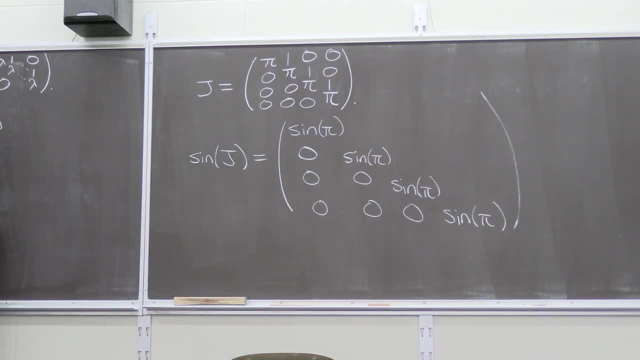 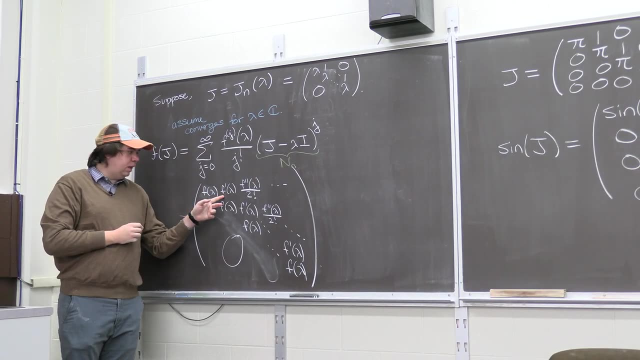 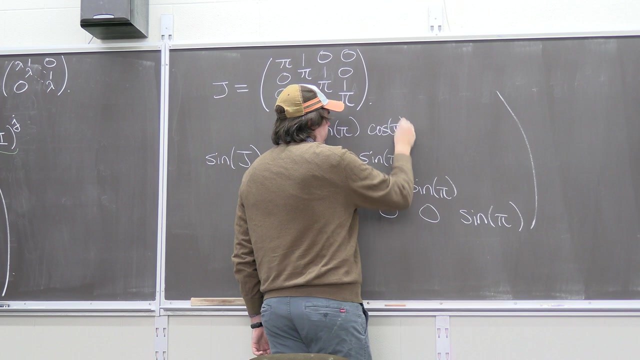 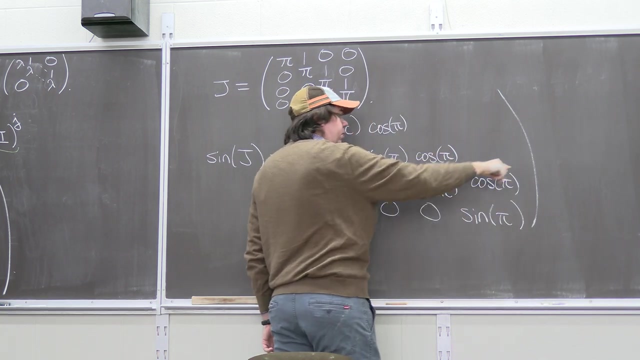 What's going to be on the superdiagonal Zero? So we have sine over pi, Sine, No, Sine over pi, Cosine, Yeah, cosine of still pi. So here we'll have cosine of pi, OK, and then, if we move up a diagonal, what do we have? 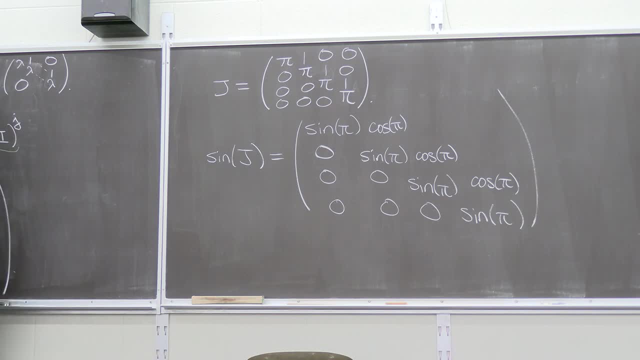 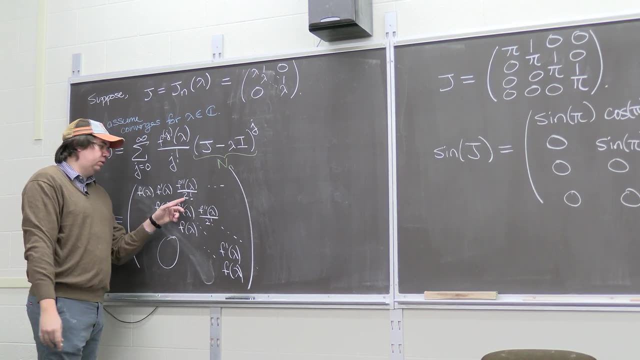 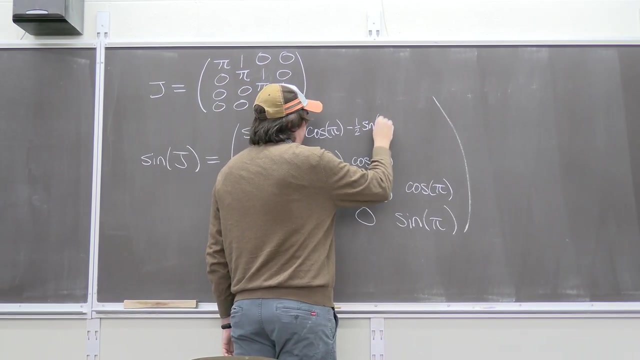 Derivative of cosine. Stop What. Diagonal, Diagonal, Diagonal, Diagonal Cosine is negative sine. but we also have to scale by this two factorial. So it's minus one half sine. So we have minus one half sine of pi. 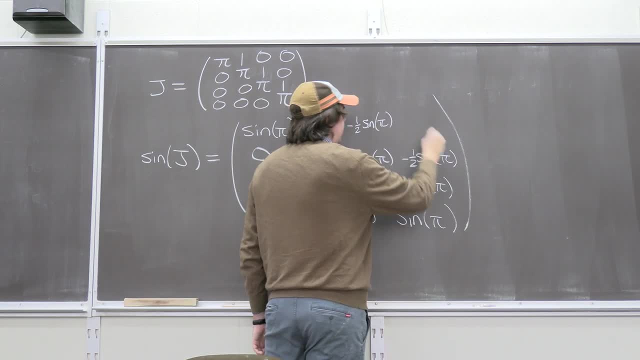 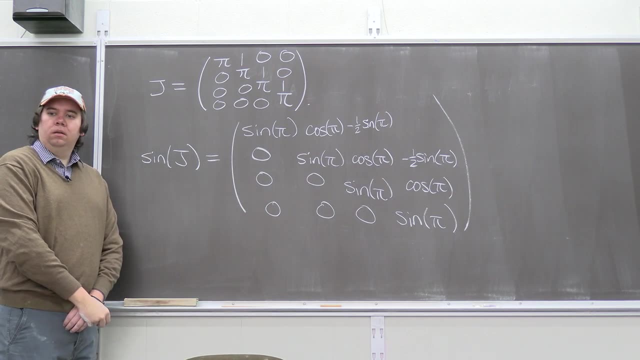 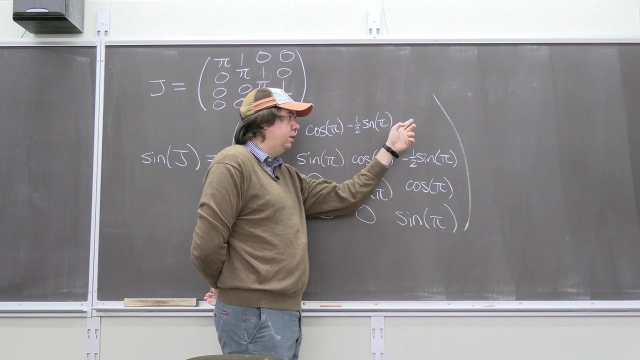 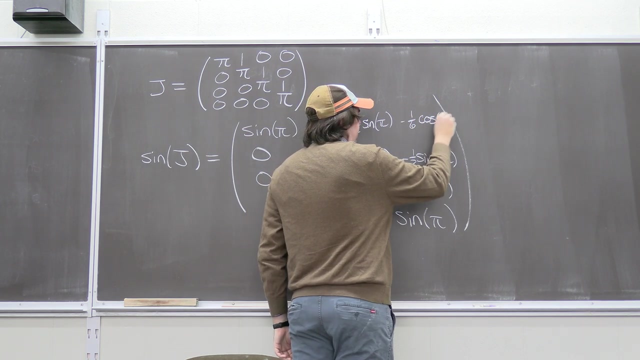 We have minus one half sine of pi. And what's gonna be up here? Well, yeah, the derivative of sine is cosine, so it's minus cosine. but now it's three factorials, so it's a six. So it's minus one sixth, minus one sixth cosine of pi. 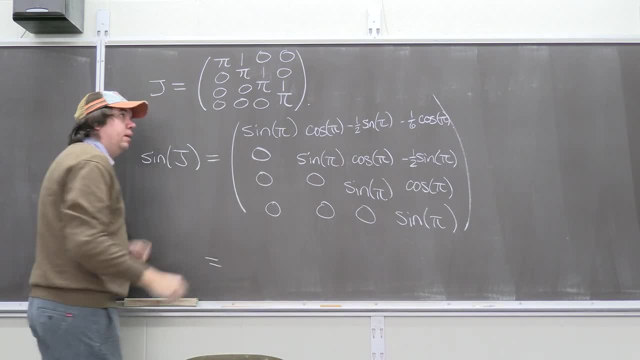 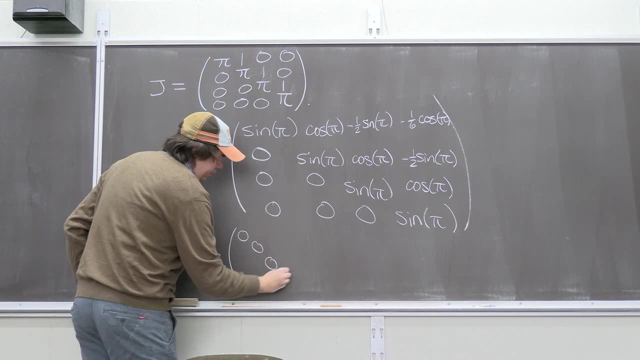 That's what this is telling us. And then you can just simplify this: At pi your sine is zero and at pi your cosine is negative one. So we just have zeros along this diagonal and we have negative ones on the super diagonal. 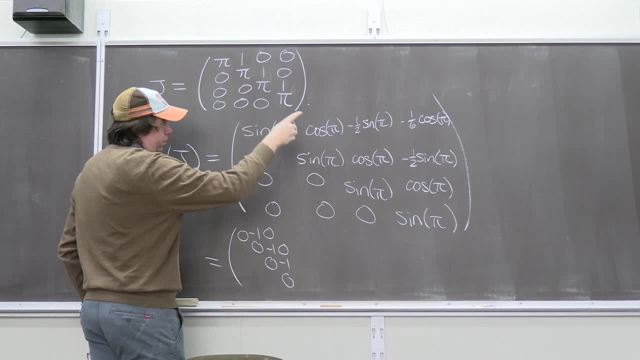 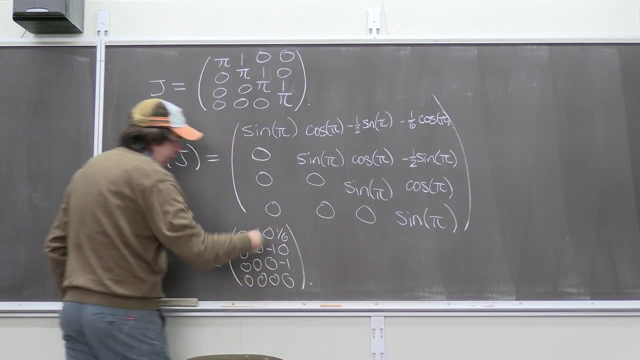 and then zeros again, And then cosine is negative one, but it's negative negative one. Then we have a one One, sixth. So here is what sine of j comes out to be, And it's like I don't know. maybe you wouldn't have expected that. 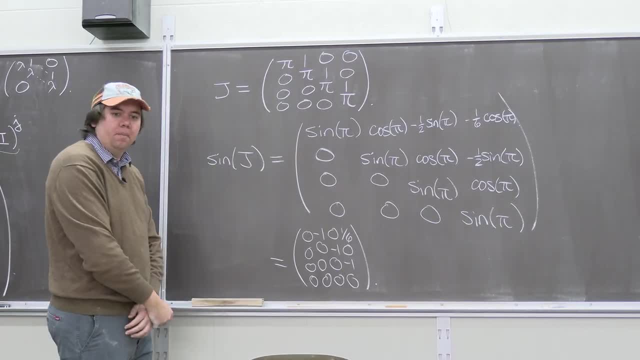 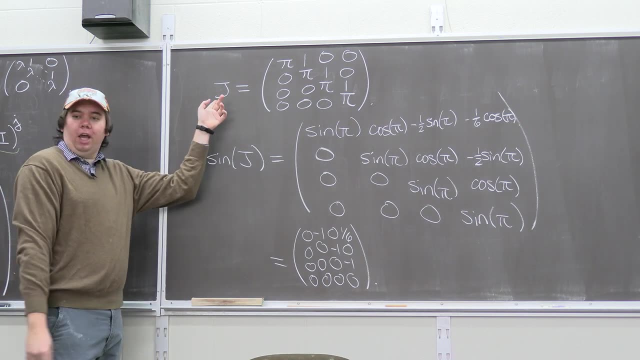 Like, how do you get from there to there? But this is what we just showed. Okay, are we happy with that? The problem is like: not every matrix, though looks like j right, Like I have a matrix we started with. 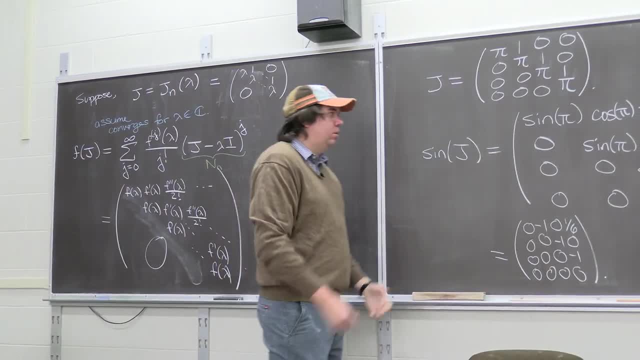 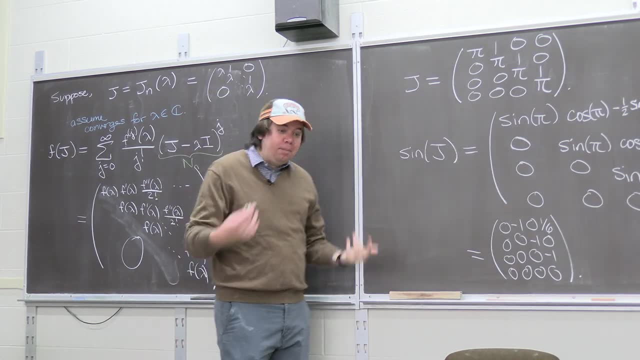 or I erased it now like three minus two, two minus one. So what we want to do now is we want to extend this more generally. It's like: well, not every matrix looks like j, but every matrix is similar to something. 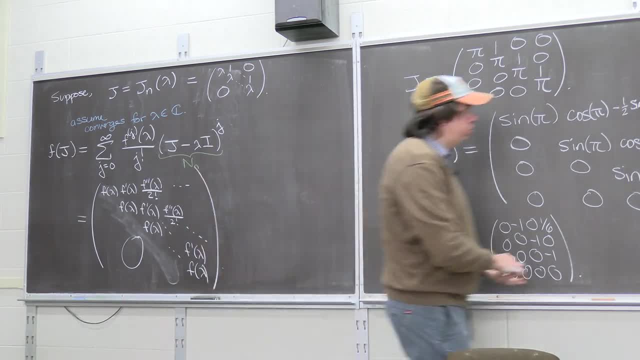 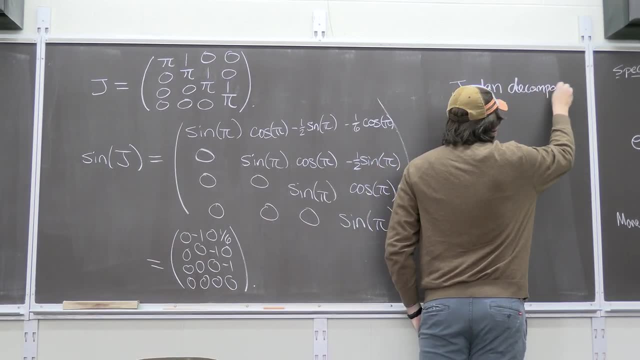 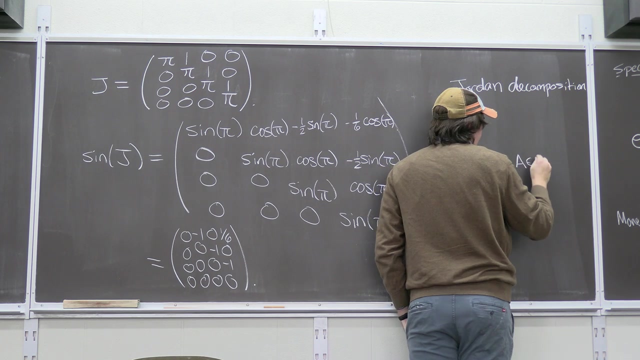 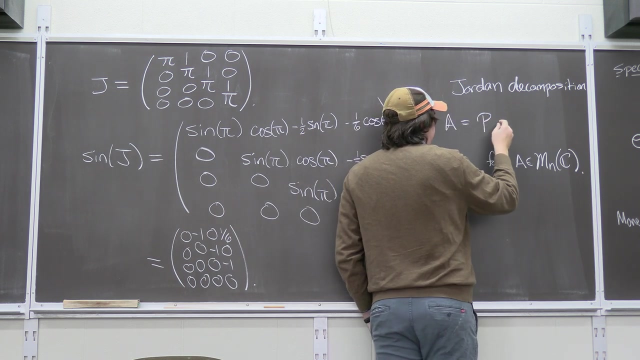 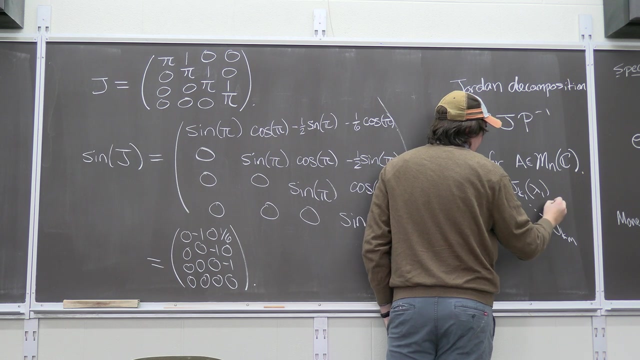 that looks like things built up of j's. So our Jordan decomposition that we discussed the last two lectures tells us that for any A square matrix complex entries, you can write a up to some change of basis as j, where your j is made up of these jordan blocks, j k 1 through j k m, with some, you know, lambda 1. 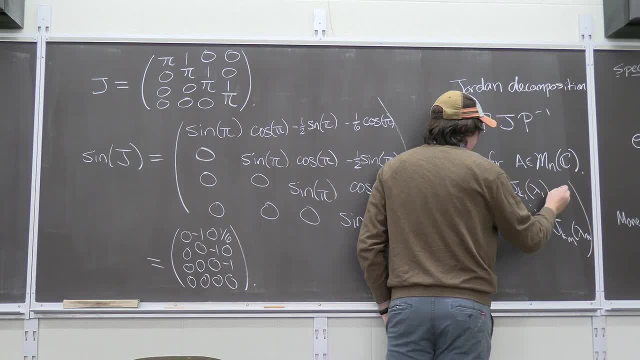 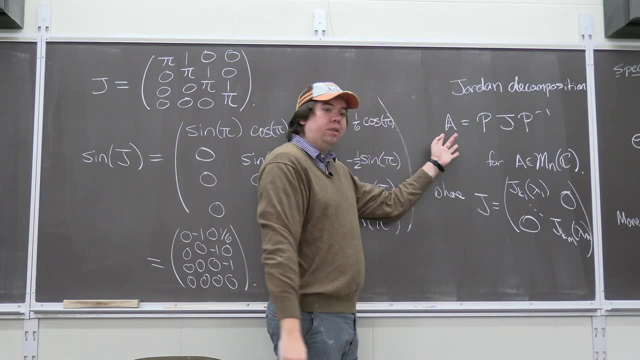 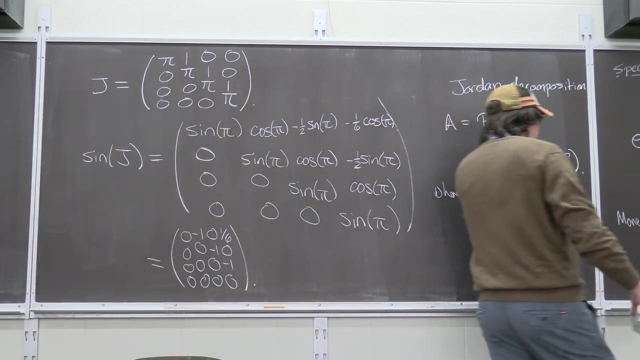 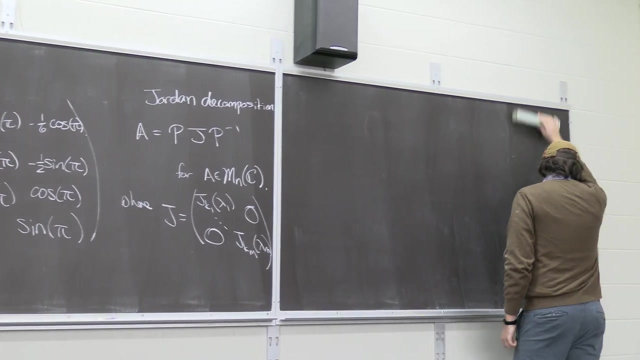 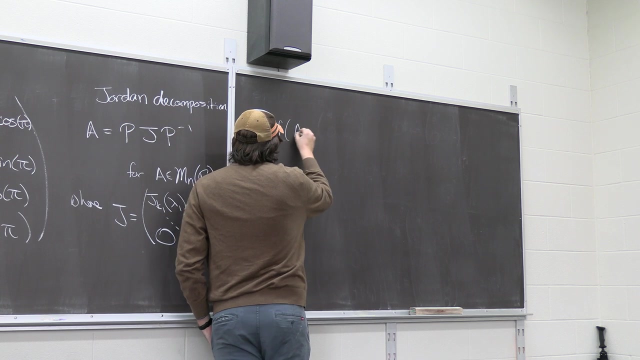 through some lambda m zero is ever else right. so let's use this to now try and think about what the analytic expansion would be if we, if we use this decomposition. so i'm trying to figure out what is f of a, but we're going to say f of a is just f of p j. 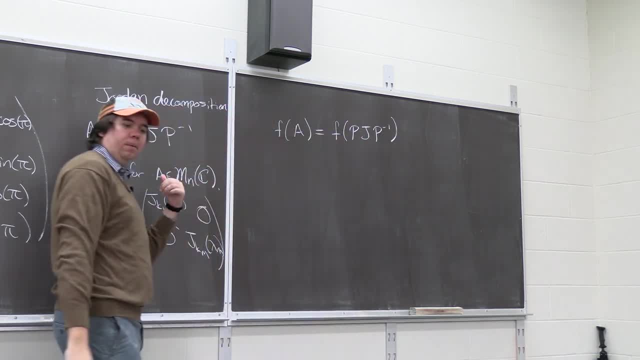 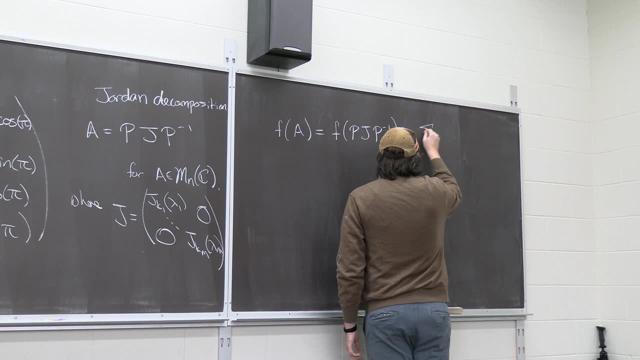 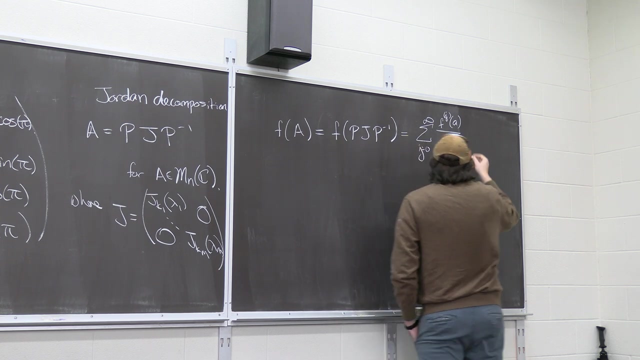 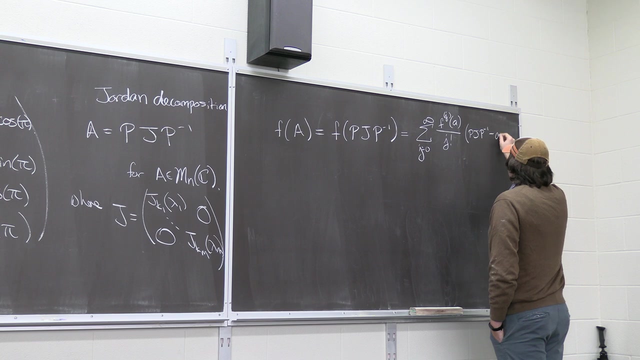 a p inverse using our jordan decomposition, and then this will just come out to be: the sum from j equals zero to infinity, of the jth derivative f at some point, a all over j factorial times, p, j, p, a p inverse minus a times the identity to the jth power. 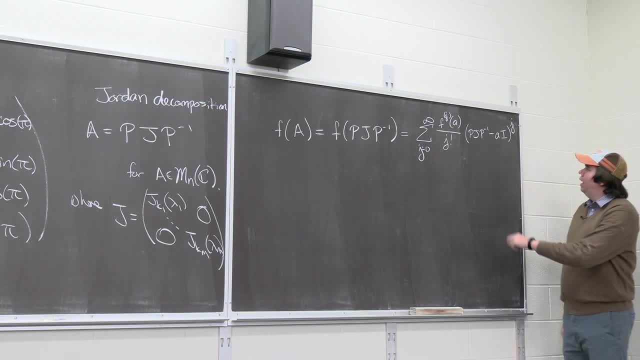 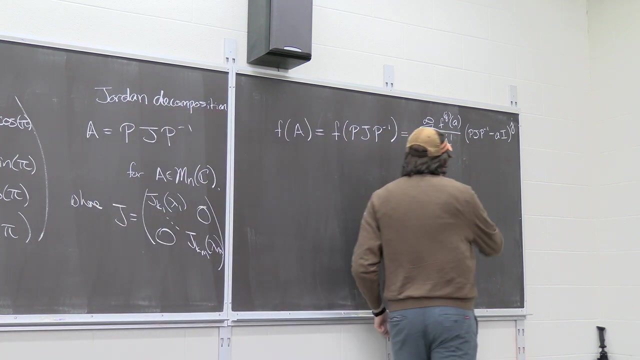 And now we want to think a little bit. It's like, okay, how can we simplify our lives? Well, here I want to pull out a p and a p inverse. So the first move is going to be to recognize this here is the same thing as p times j minus ai. 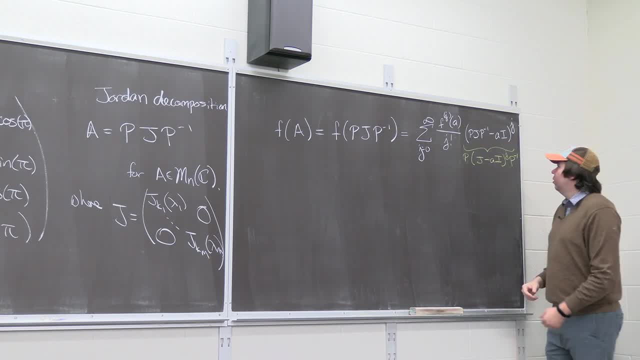 to the j times p inverse Why? Well, you know, just think about, like, when you multiply him by a copy of himself, you can well, on the inside, you can first do this on the inside. This inside of this guy is just. 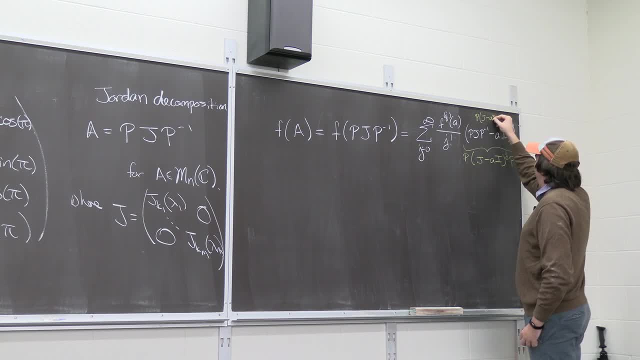 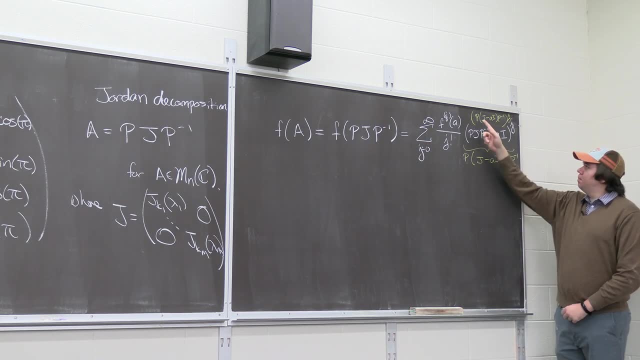 p times j minus ai times p inverse- All to the jth power, right? Because that p and the p inverse times ai is still ai, And then when you raise this to the jth power, you're just stringing these next to each other. 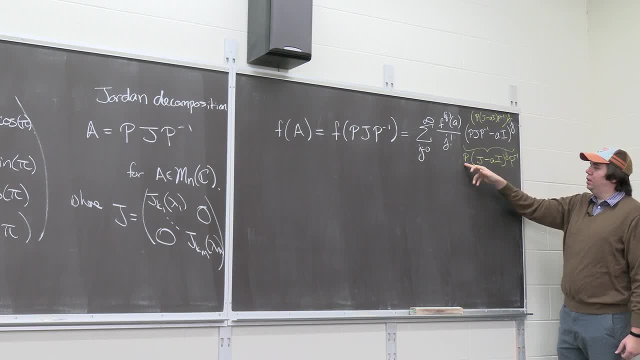 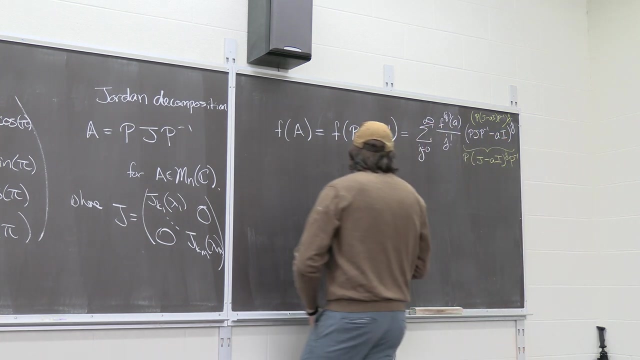 So the p and p inverses cancel in the middle and you're just left with one p at the beginning and one p inverse at the end And j copies of the center piece. And then this is just a scalar, So I can rewrite this as p times. 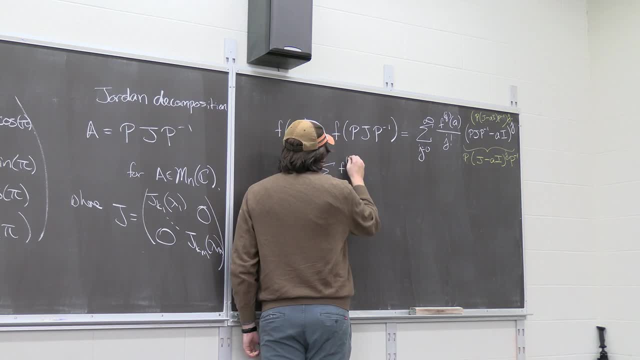 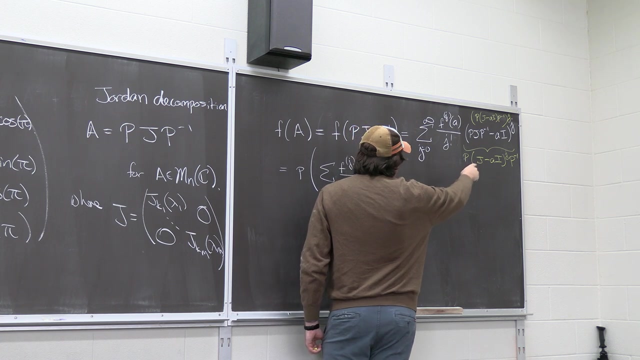 bring the scalars inside: the sum of the jth derivative of f evaluated at a divided by j factorial times. this matrix j minus ai, which let me write that as a matrix j minus ai, would be your first block up here, minus a copy of ai down through, your last block down here. 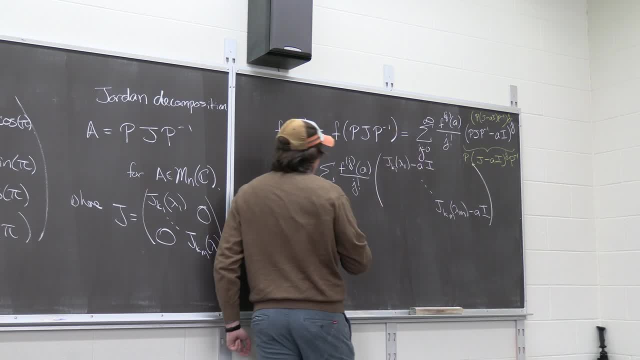 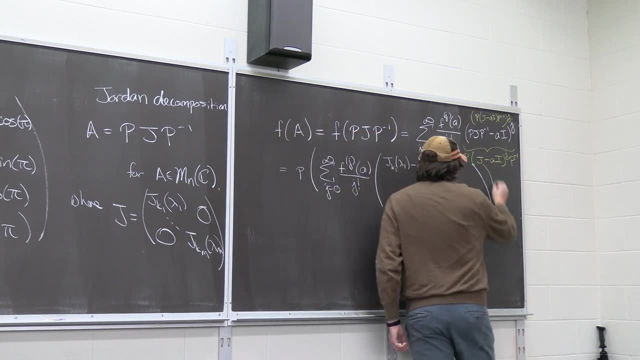 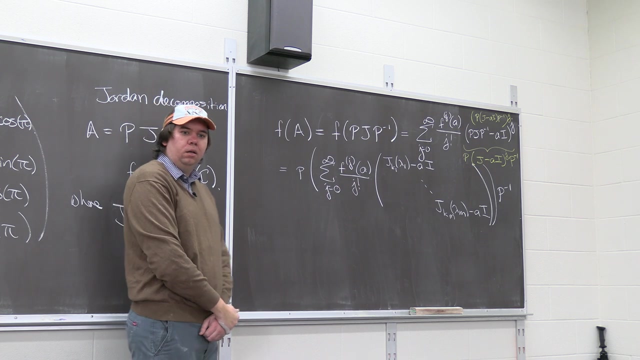 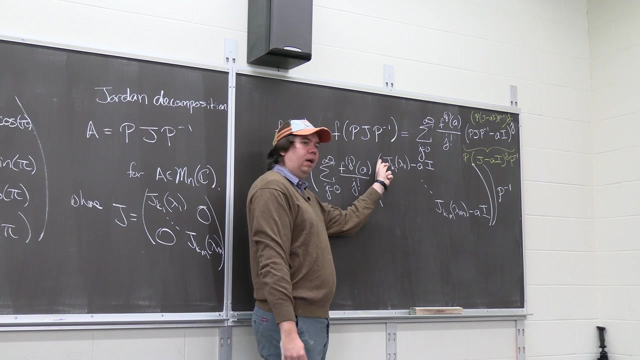 times a copy of ai where j goes from zero to infinity, And then that whole thing times p inverse. But now here's just the sum of scalars, times matrices, and you can bring the scalars inside, move the sum inside, just adding it component wise. 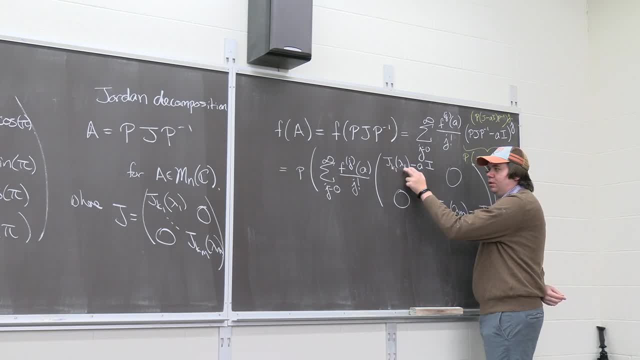 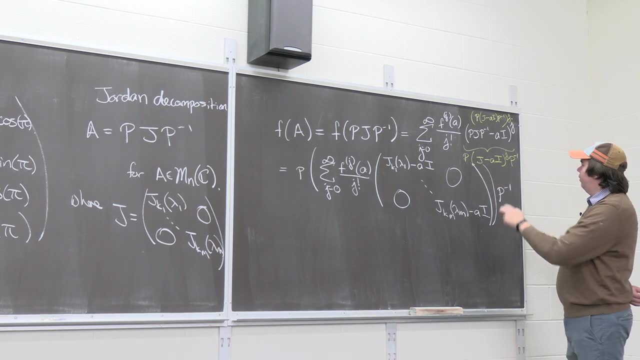 And so we're just summing this expression right here. Just the sum of the scalars times this All the way down to this. oh, oh, did I forget? I forgot to do powers. This is to the jth power. 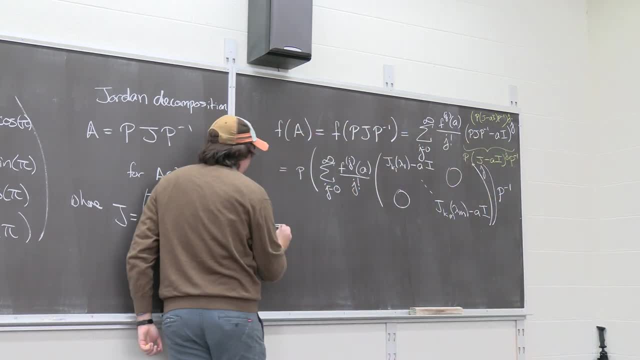 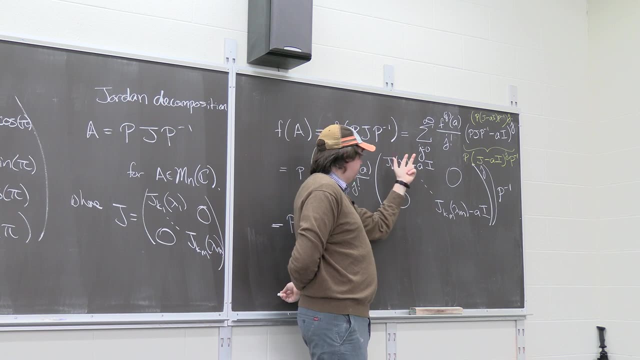 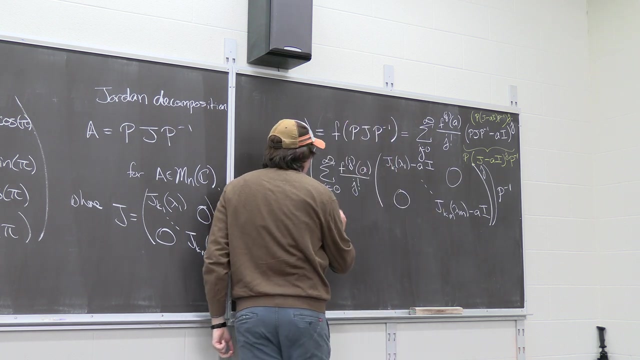 Okay, maybe I should write this as one more step. So this is just p times. this is a block diagonal. I have these matrices forming these blocks along the diagonal, And so this to the jth power would just be whatever he is to the jth power. 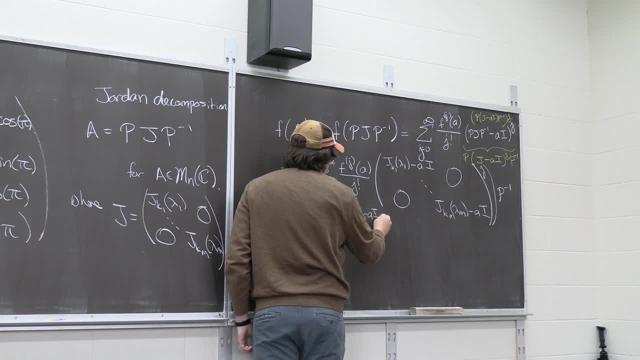 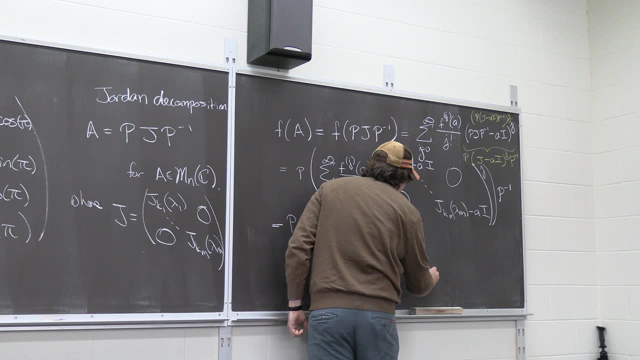 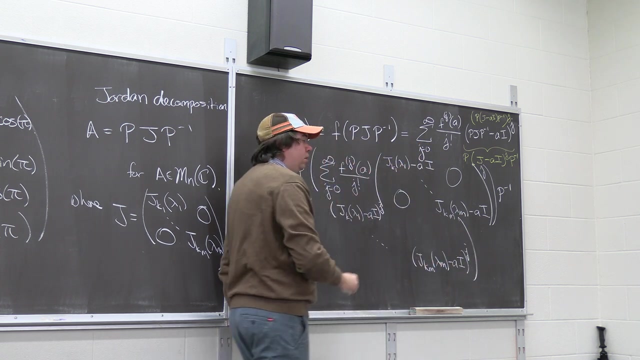 jk1 lambda one minus ai to the jth power, Down through whatever this guy is down here- to the jth power. jkm lambda m minus ai to the jth power. And then I'm going to move inside the scalars and the sum. 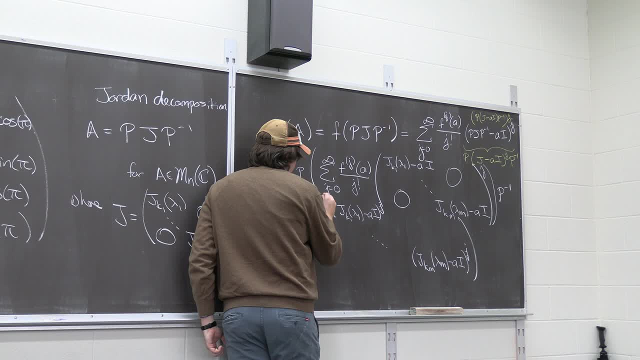 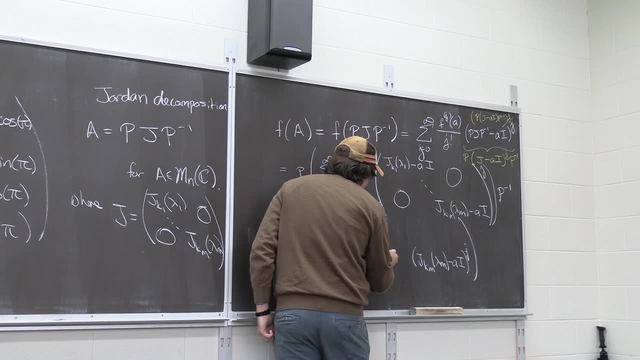 So times a sum of the jth derivative of f evaluated at a over j factorial, all the way down here to the sum of the jth derivative of f evaluated at a all over j factorial, And then finally, at the end, I have a p inverse. 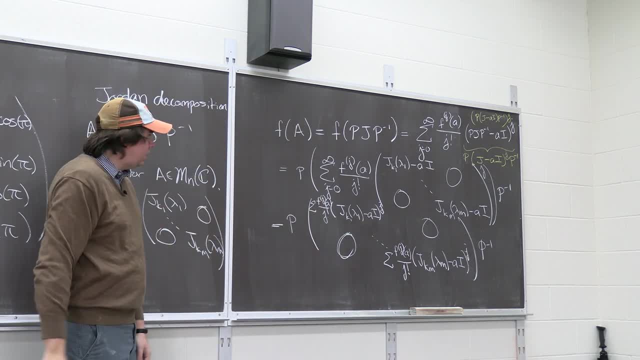 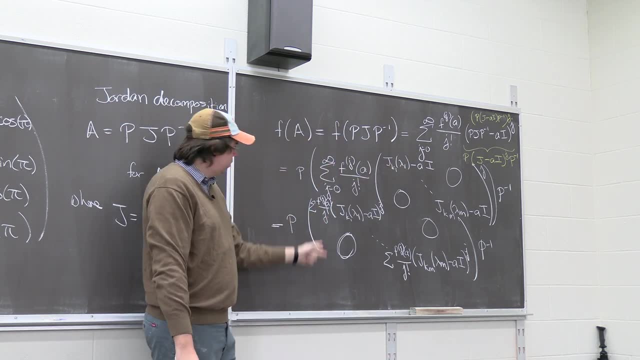 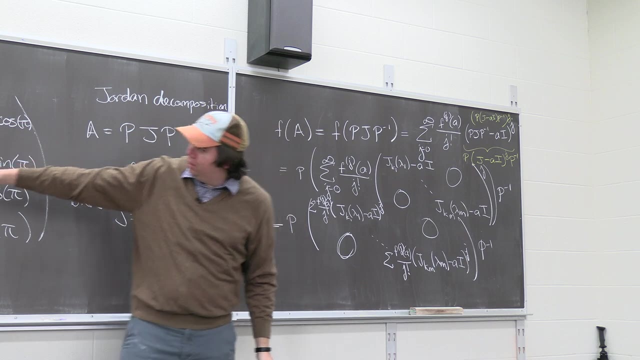 Woo, Okay, That is just to say, since this is just block diagonals, it plays very nicely with powers and sums, Right? So you just end up with: well, what is this? Well, I've already said this is this expression we had over there. 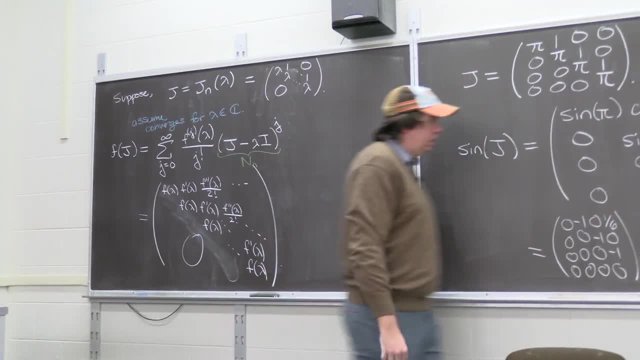 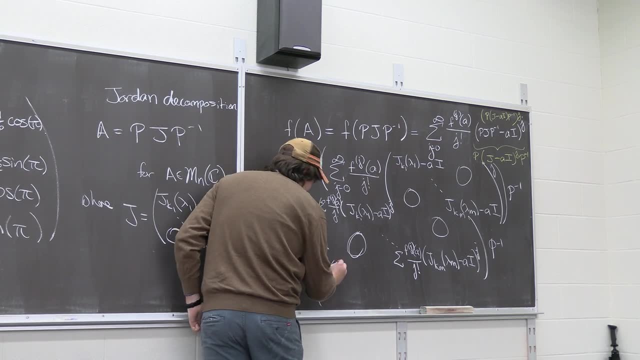 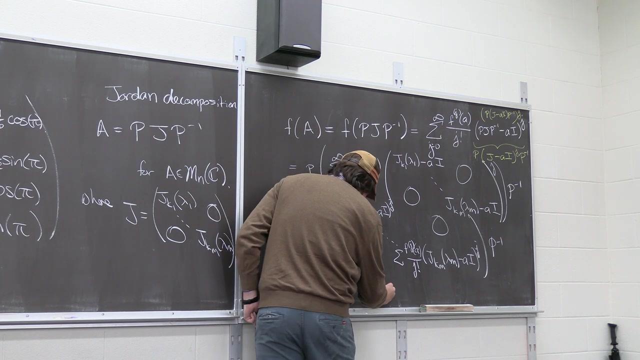 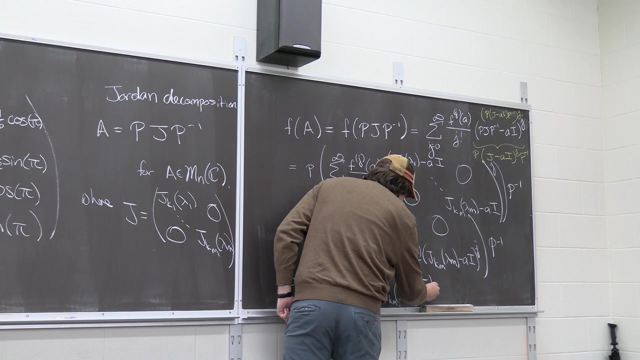 That was exactly our definition of just f of j, And we know how to calculate f of j. This just comes out to be p times f of your jk1, lambda one down through f of your jkm lambda, m times p inverse. 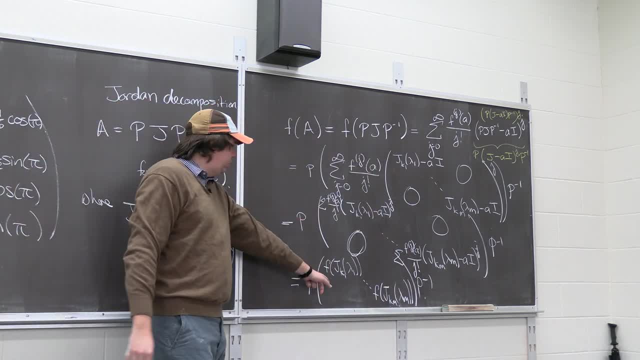 And so, like all this is saying is, if you want to- and we're going to go through all the steps next, but I'm not saying that we don't have to do anything- want to calculate? F of A? write its Jordan decomposition. 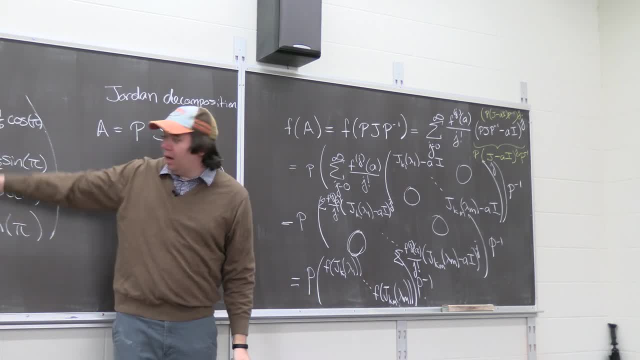 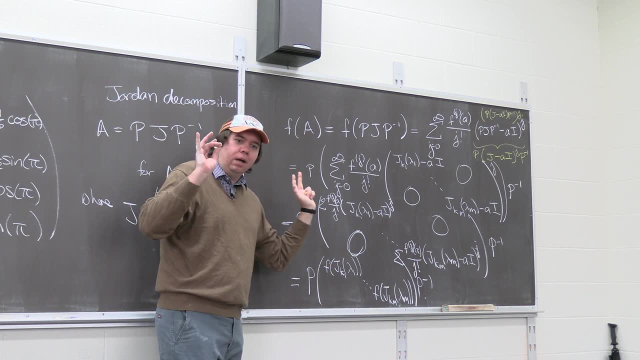 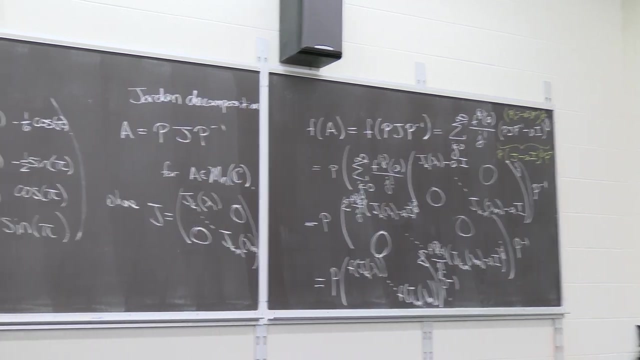 and then, for each block, just do like we did to this block. You should do block by block and then you can multiply it out and you're done. So let me just show you this. show you this in practice. So we're still gonna be following this rule here. 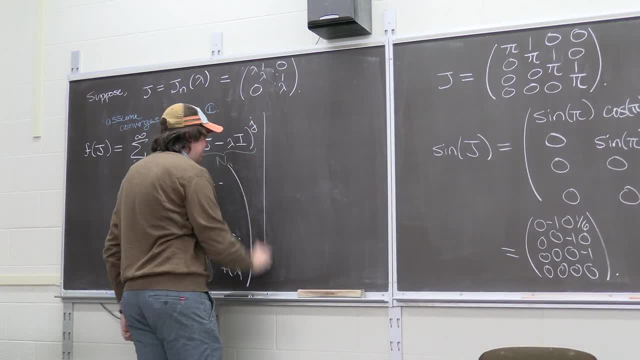 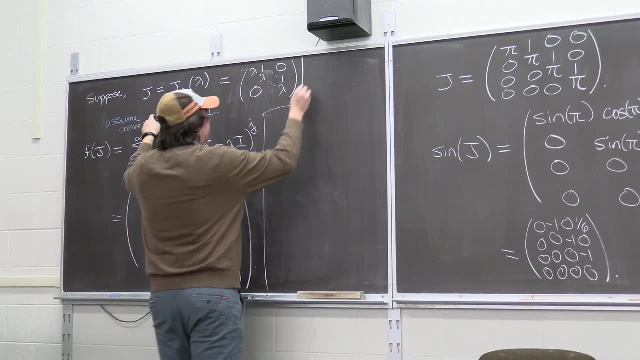 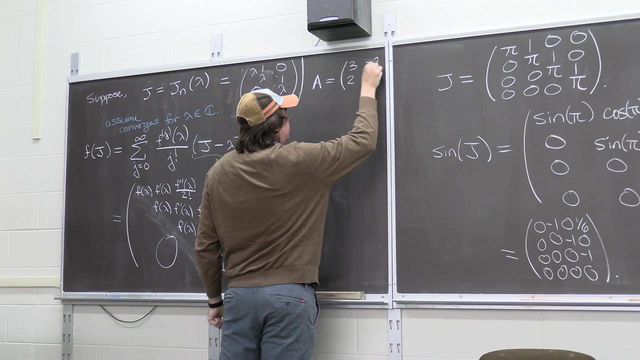 for our blocks. but you know, let's think of like a concrete example. So the example we opened class with today is: I had A equals. there's still like a remnant of it. A equals three, two minus two minus one. 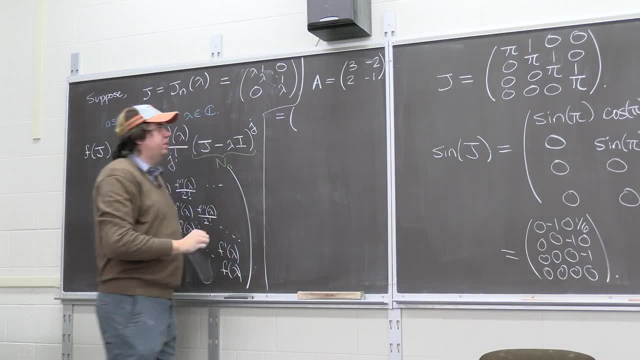 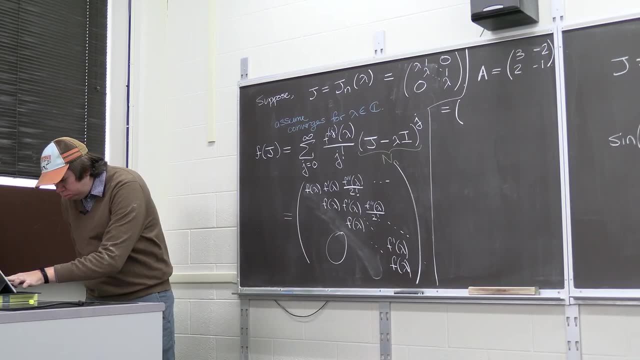 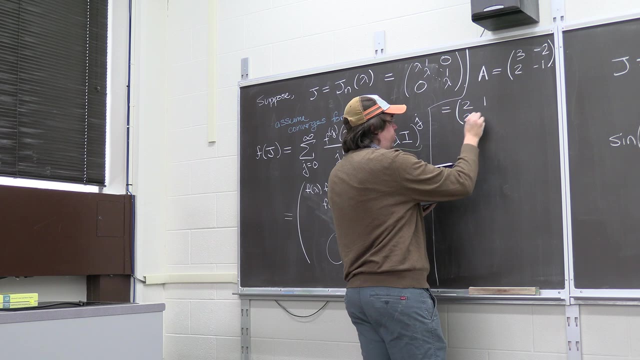 And if we find the Jordan decomposition? for that the Jordan decomposition just comes out to be- let me find it, I did it out the other night- Doo, doo, doo, doo, Here we go. It just comes out to be two, one, two, zero. 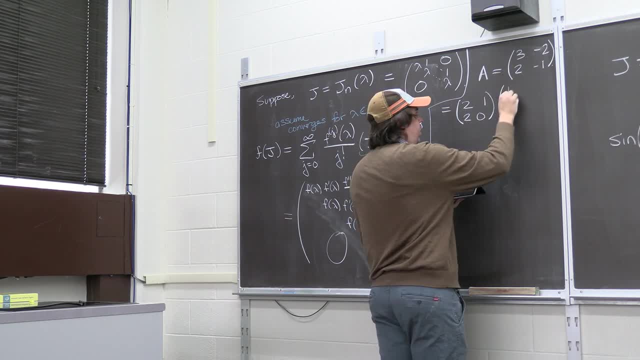 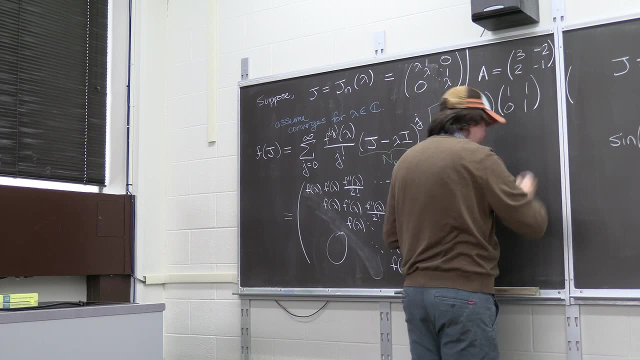 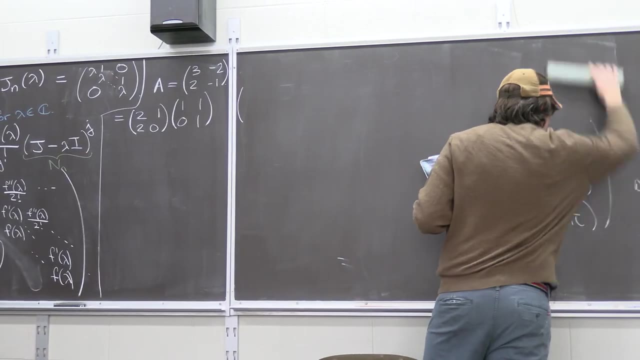 That's my P. My J just was one, one zero one, So it's a single Jordan block, with lambda being one, and then P inverse, which here we don't need all this anymore- And then P inverse, which is just the inverse of this guy. 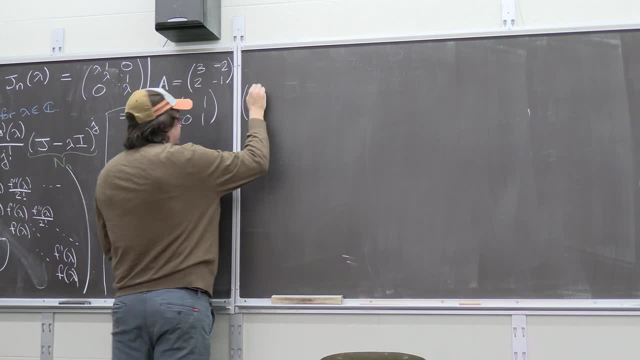 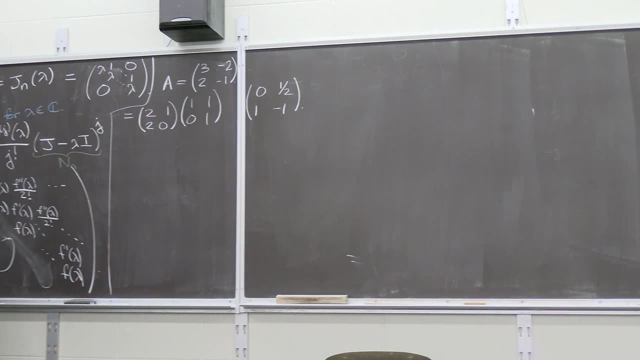 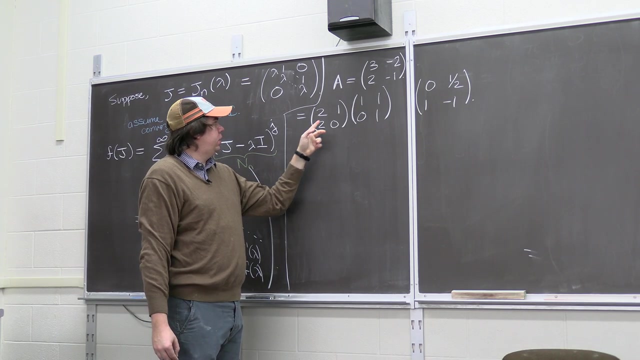 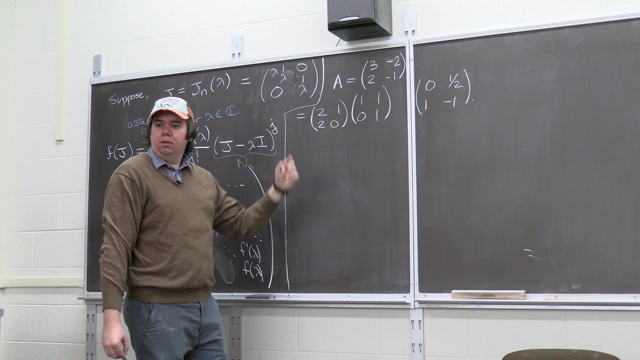 So times by one over the derivative. So it comes out being this: I believe That. look right, These switch place, these change signs. but then you have to divide it all by negative two. I think that's good, right. Negative two, so negative, yeah, that's good. 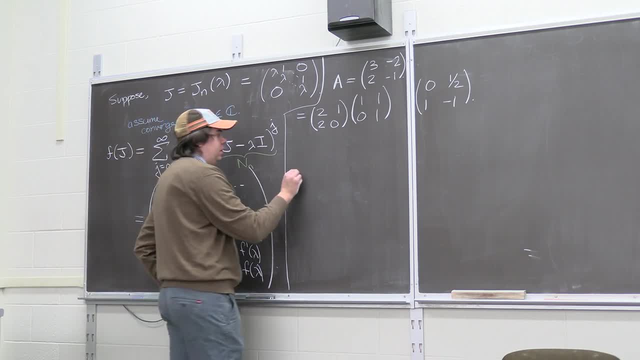 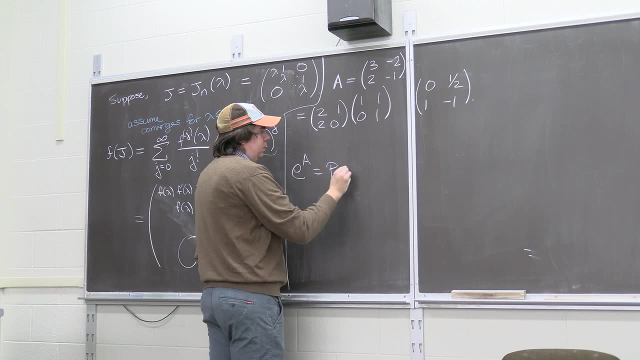 Okay, so how do we do this, Like, how do we calculate E to the A? What this is telling us is all you need to do is instead do this P times E to this J times P inverse. That's what the theorem says. 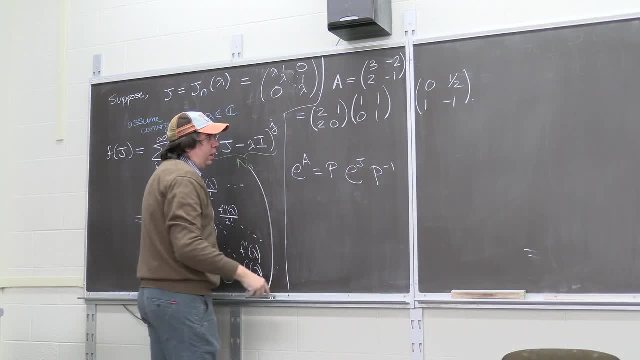 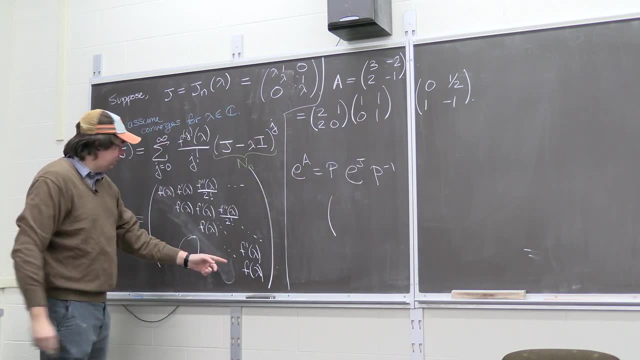 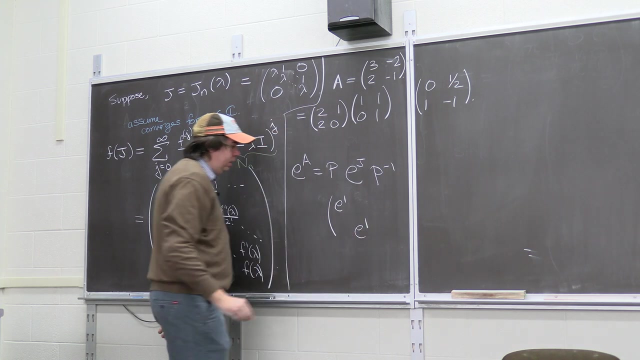 That's what our result says, And we know how to do E to the J. When you have something like this, E to the J is just, it's like you follow your directions. You do E of your lambda values. So it's like E to the one, E to the one. 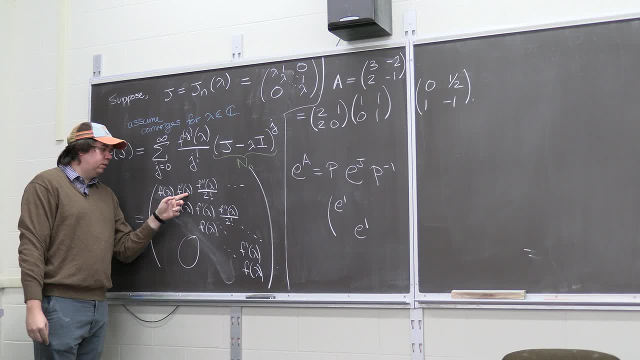 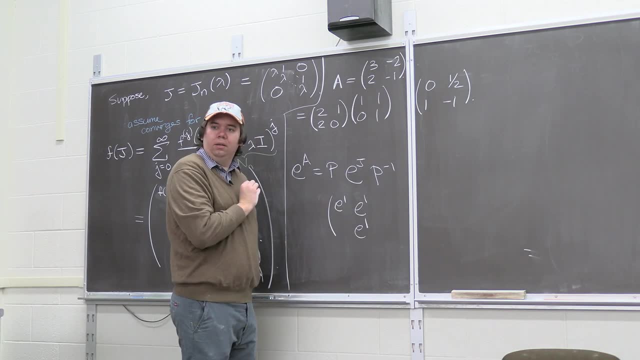 And then one diagonal up. it's the derivative of E to the X. with your lambda value, The derivative of E to the X is still E to the X. so it's still E to the one up here. So it's still E to the one. 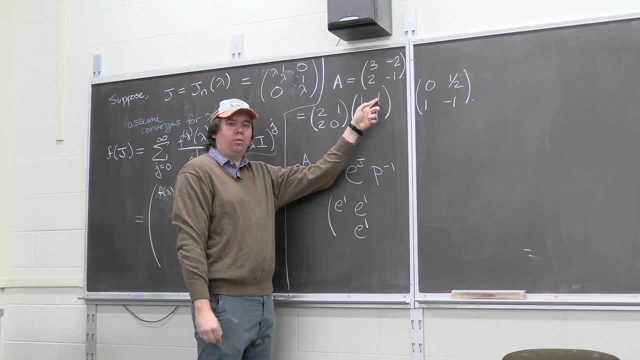 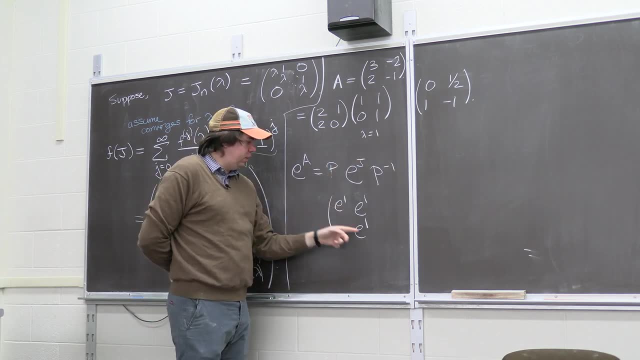 If these had been twos, that would still be an E to the two. This one is not coming from this one right. This one is from the fact that my lambda- here, my lambda, equals one, And so I'm plugging in one to E to the X. 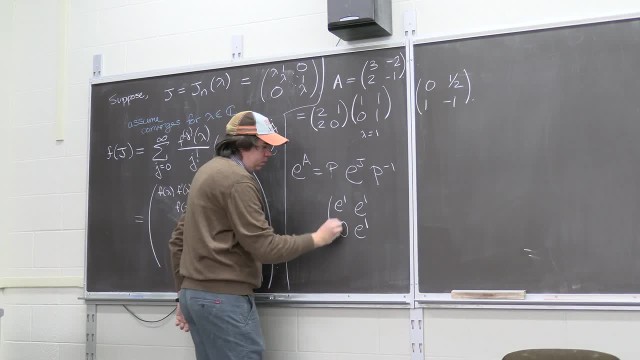 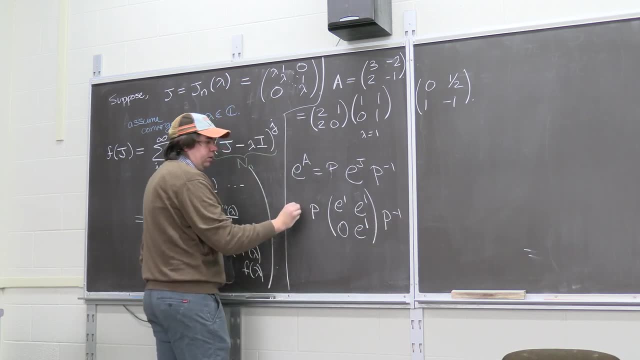 and to the derivative of E, to the X, And then you're just timesing that by your P and your P inverse And you can just do that out. But you look at this and you're like what just happened? Well, in this particular case, 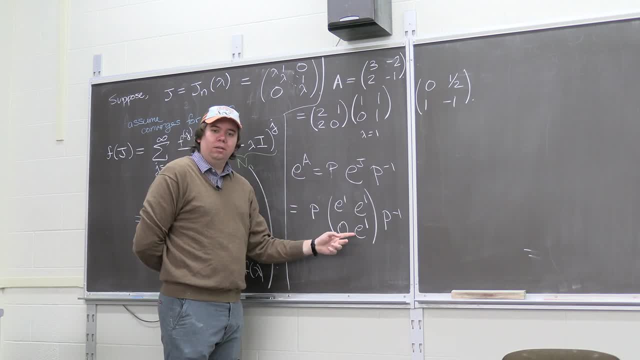 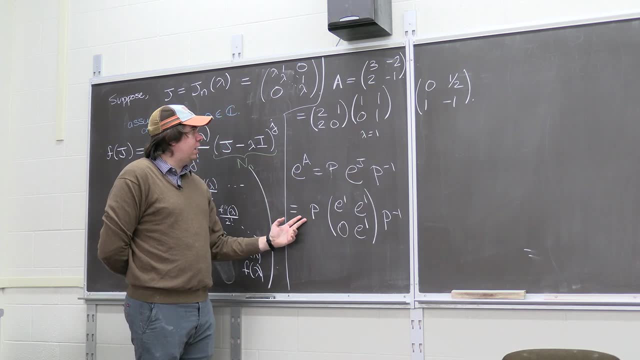 I just scaled this matrix by a copy of E. Just E's here, So if you just pull out that scalar E you're back to the original matrix J that you had, And so you just picked up a scalar copy of E. So you really just ended up with E times A. 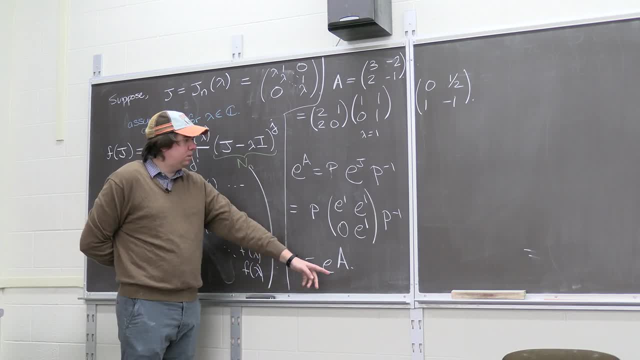 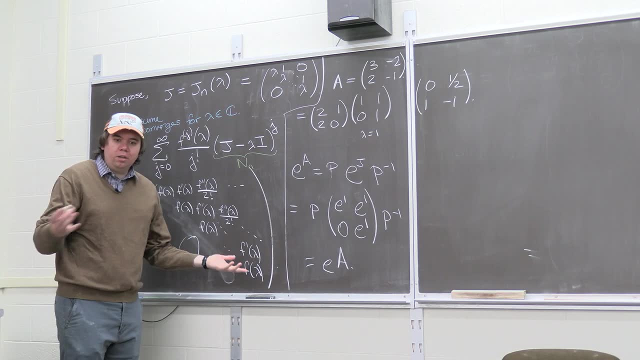 This doesn't usually happen. This is kind of a weird case, right, But that's what this comes out to be is just, you pick up a scalar multiple of E from doing this, But you can do other things too, right, Like what, if you want to calculate, say, 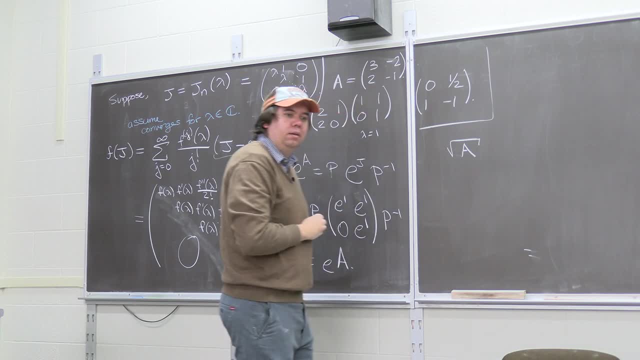 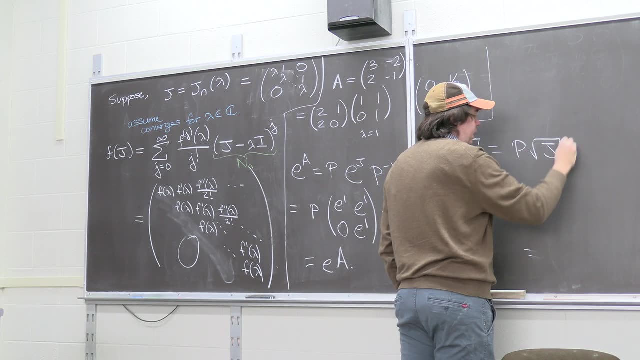 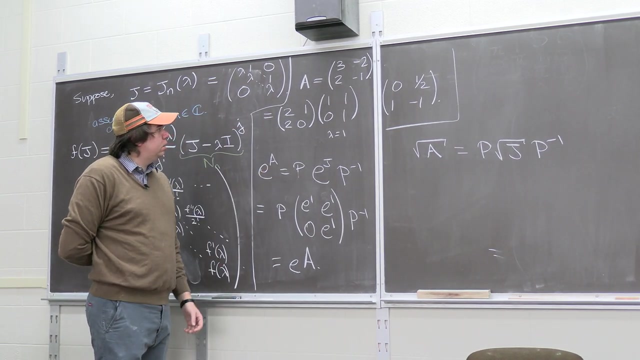 the square root of A. Well, this formula's telling us: you just do P times the square root of J, times P inverse. So let's think about what is the square root of J here. Well, what we do according to this: 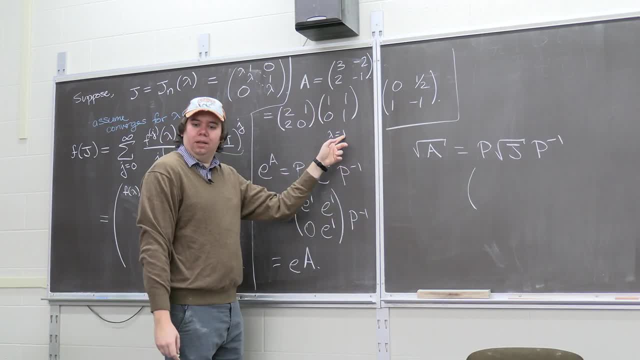 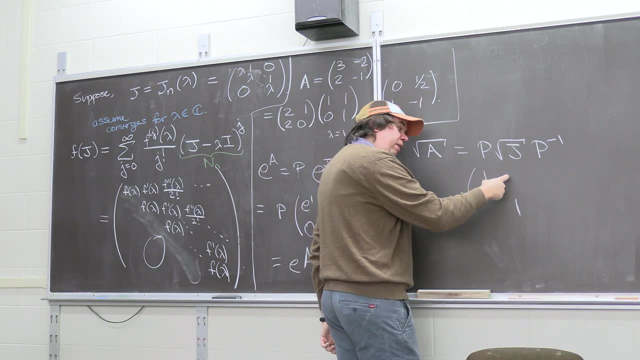 is, we do the square root function with one plugged in. lambda equals one on the diagonal. So plug in one two square root, you just get one. Then what goes here? Well, the derivative of the square root function, that's one over two root X. 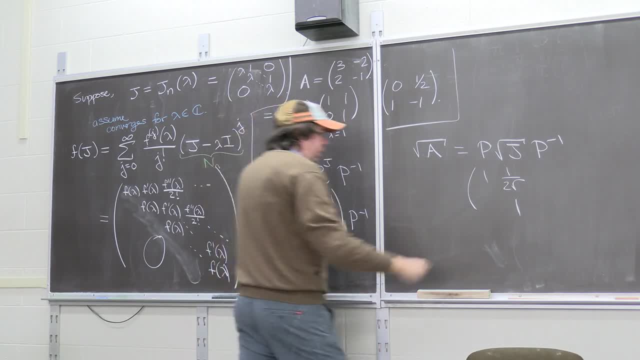 One over two square roots of X, But my X here is my lambda. Lambda equals one, So what I end up with is one half in that corner. So I do this Good, And if it was a bigger matrix you would just do more derivatives. 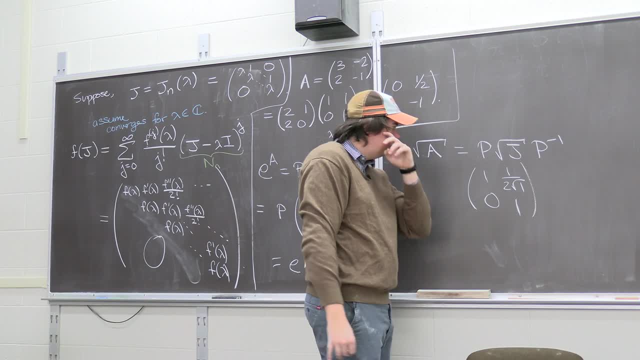 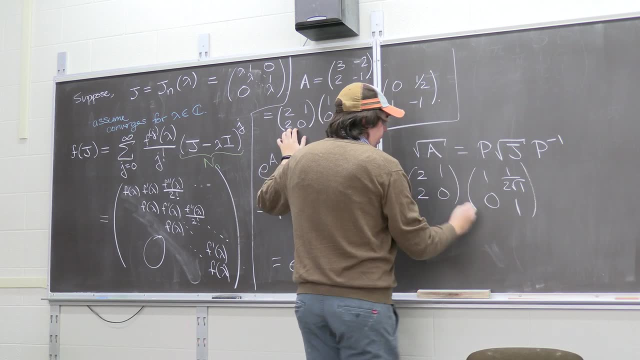 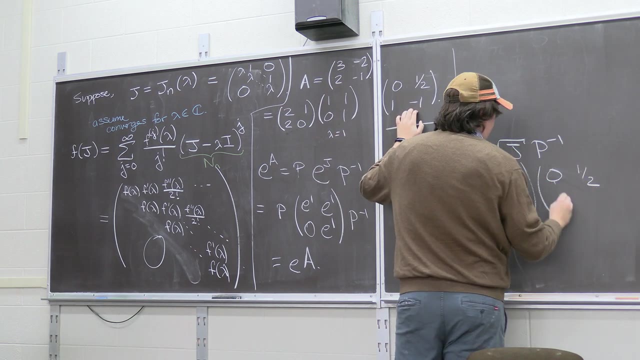 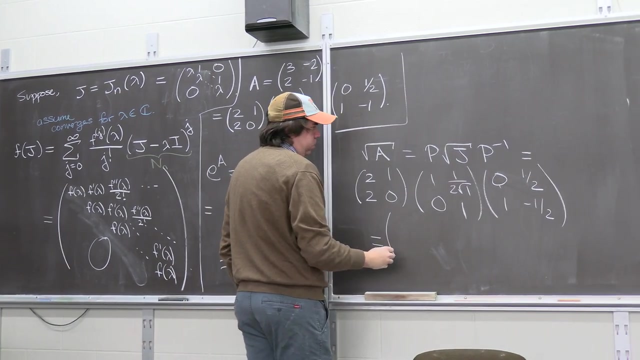 And if there were several blocks, you would do it for each block separately, And then my P is still two, two, one zero, And my P inverse is still zero, one half, one minus one half. And so I end up with: oh you know, multiply these out, What do you get? I'll just give you the spoiler. 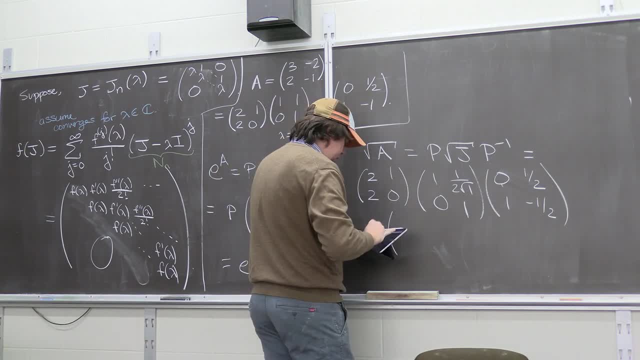 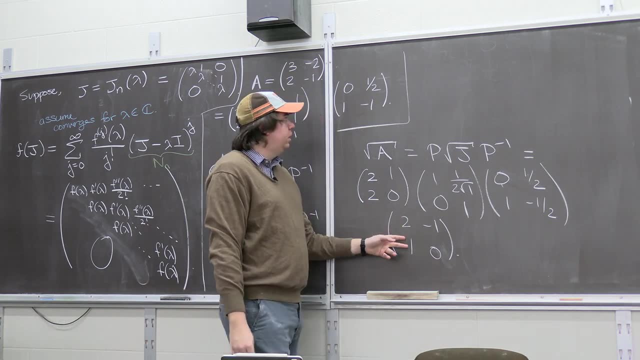 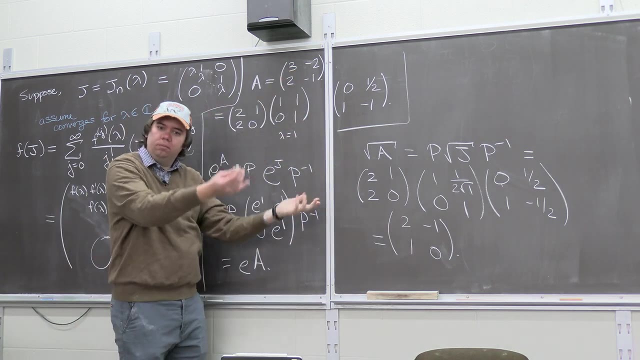 I did last night, It's. it just comes out to be 2 minus 1, 1, 0 Can multiply those out and you should check that if you square this thing, you get back to your original a. you do right. Like this row times, this column is 4 minus 1. that gives you the 3 and so forth. 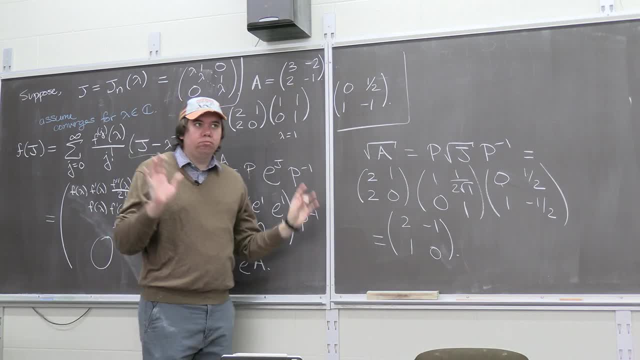 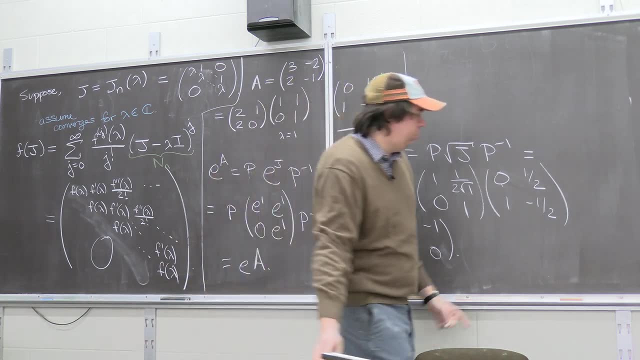 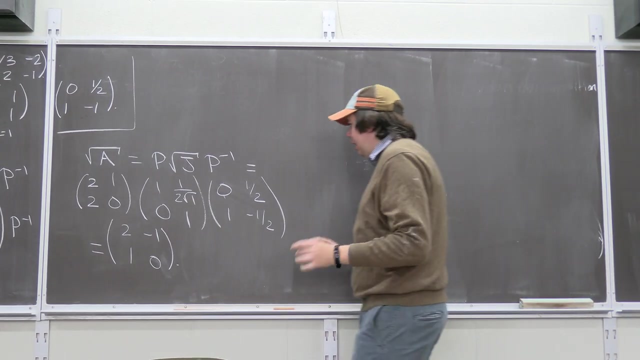 Okay, so we now know how to calculate. you know just about whatever you want. I guess I should end by giving you a little bit of a warning, Like warning. things don't always end so like: go go so nicely. like what, if I want to find the square root of B? 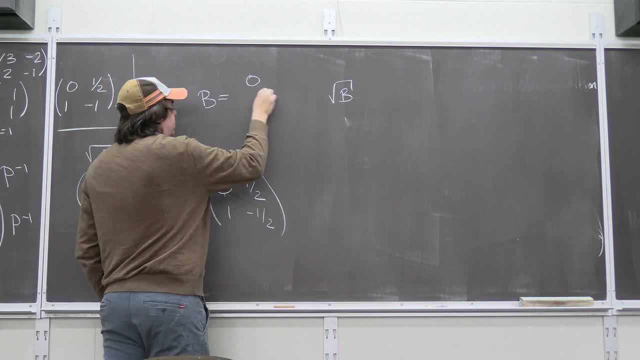 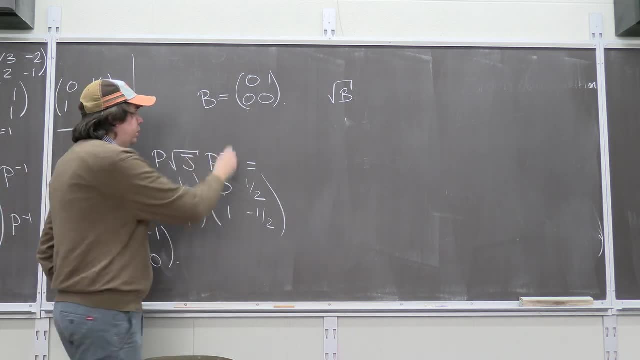 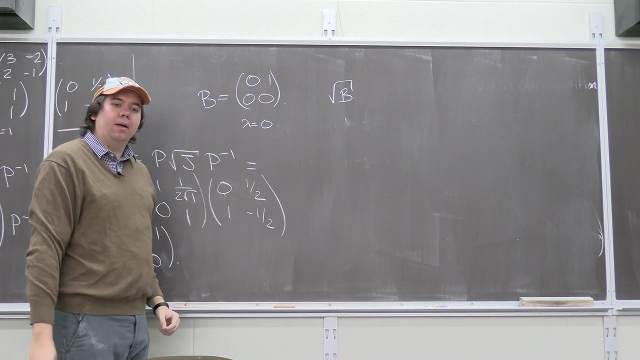 Where my B is equal to the matrix 0, 0, 1, 0. Well, it's like this is already a Jordan block. This is just the Jordan block where lambda is 0, right 0 is with a 1 on the superdiagonal. so this should just be. 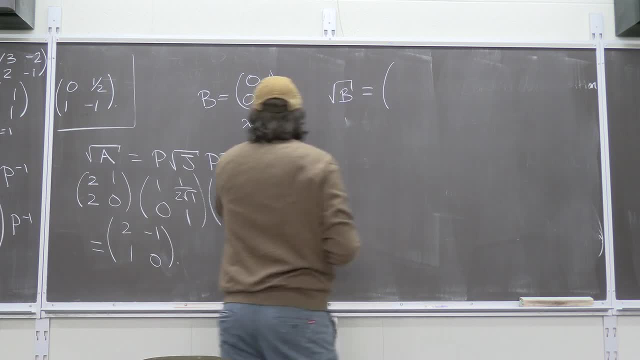 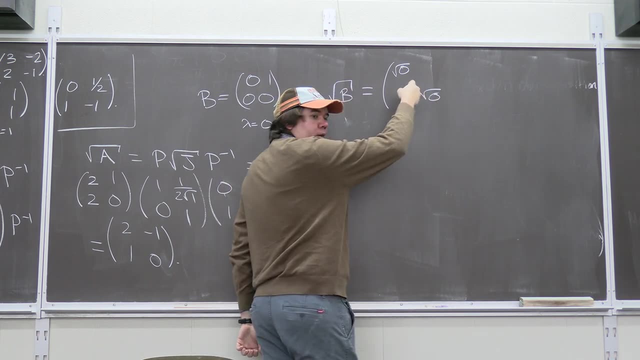 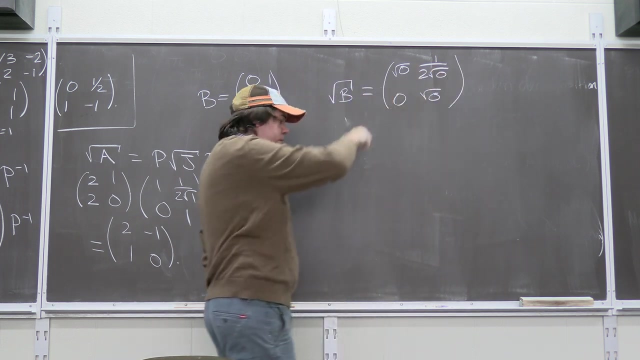 according to a formula, You plug in 0 into the square root, so it's gonna make square root 0, square root 0, but then, right here You take the derivative square root, So 1 over 2 times the square root, you plug in 0 and like: 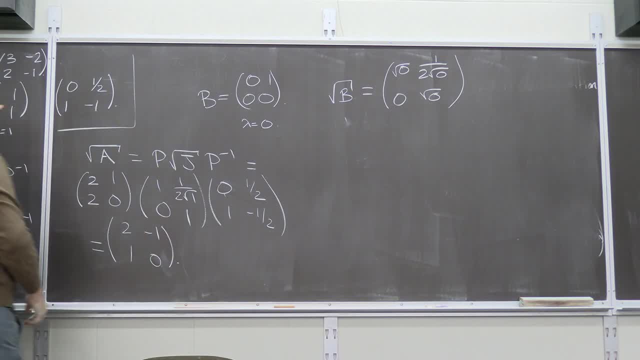 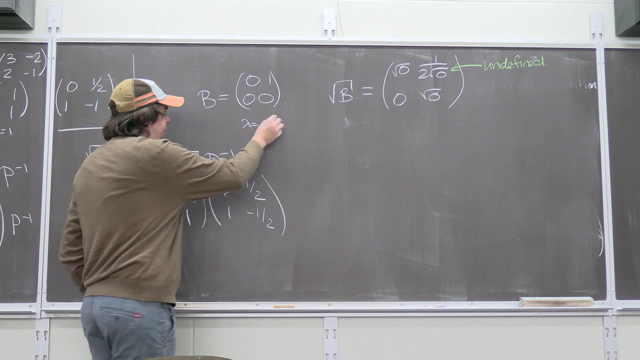 Oh, dividing by 0. This is not defined. All right, this is undefined. So it's like this: this failed. Why does it fail? Well, it's that convergence thing. it turns out that my, you know, eigenvalue here is 0 and my, my. 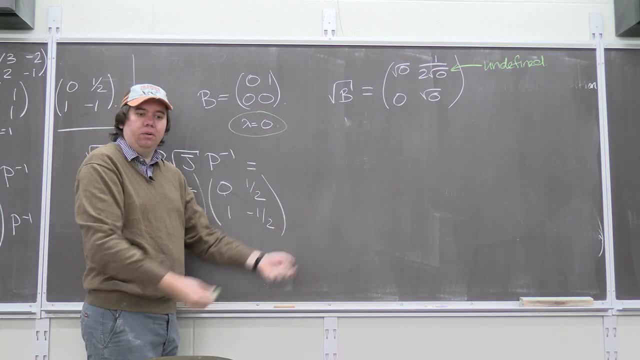 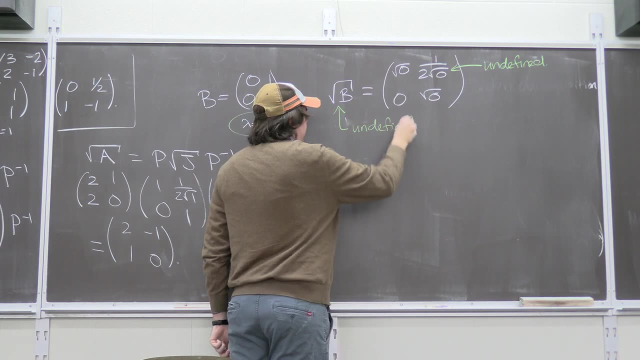 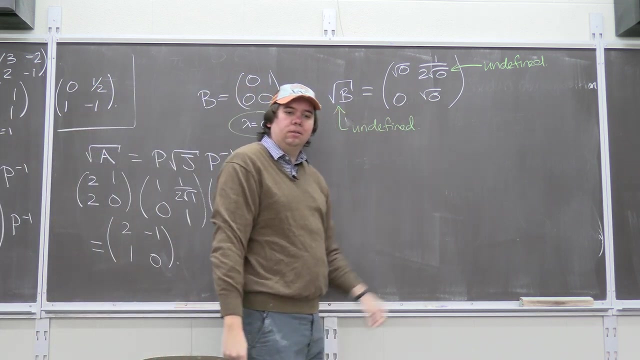 Function isn't analytic at 0, So it's not going to converge at zero right, And so this is actually undefined. We just can't define the square root of b. So from some functions you have convergence problems that when you try this out you'll run into issues like this. 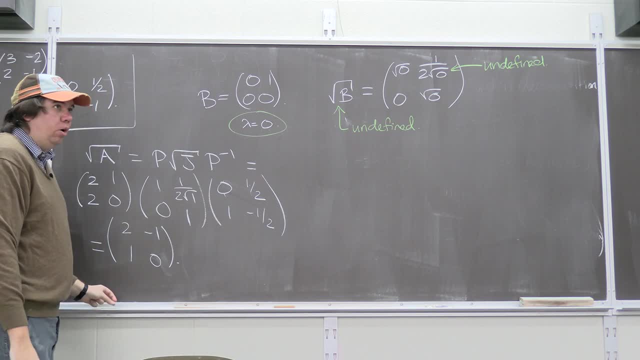 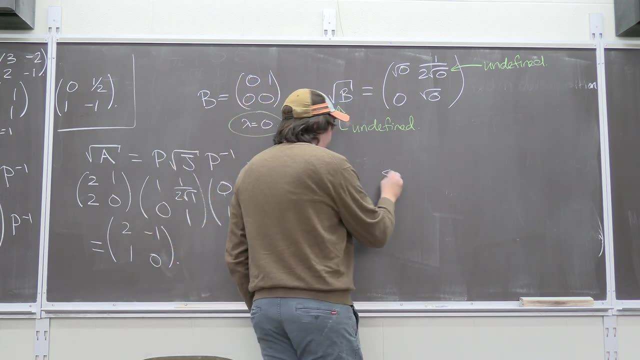 That's fine, which means it's not defined there. Okay. but now that you have this like in your problem set, you prove some cool things. I don't remember all the ones you proved, but one thing you can prove is like sine squared of a. 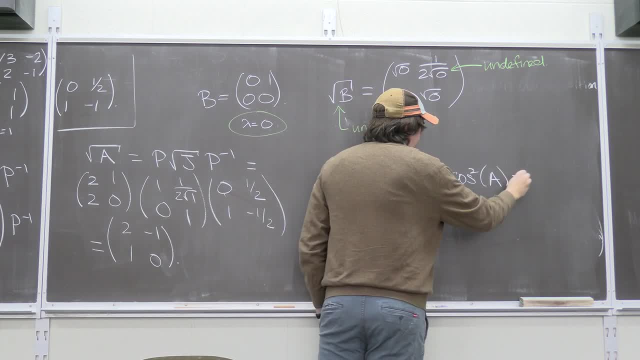 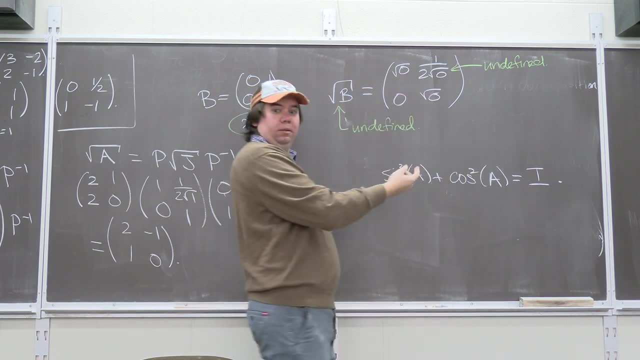 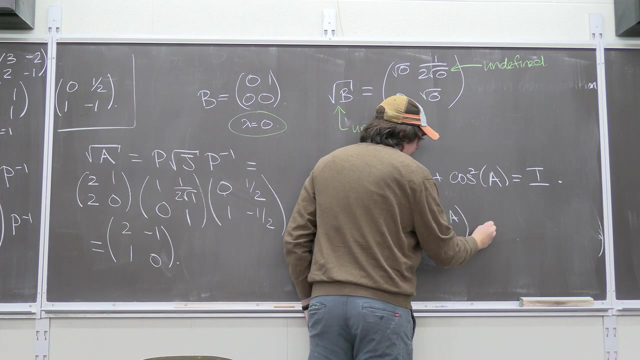 plus cosine squared of a. This follows immediately from what we've shown today. What do you think this should come out to be? Identity for any matrix? a Like whoa, that's cool. Or you'll show something like: the determinant of e to the a comes out to be e to the trace of a. 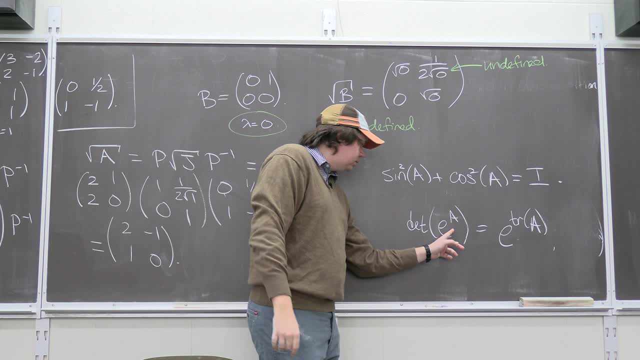 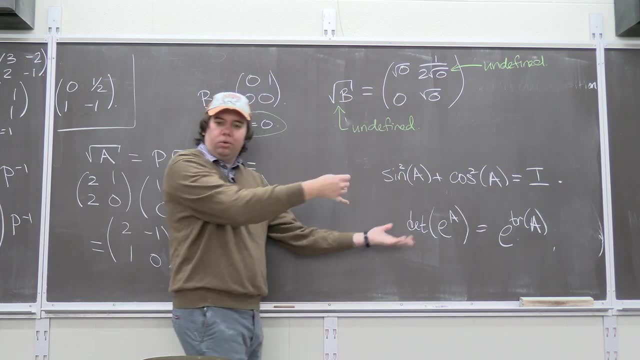 So you get the. these are scalars. This is a number, right, This is a matrix, but the determinant of the matrix gives you a number. This is e to a number. So these are both numbers and you show like you get all these cool identity relationships. 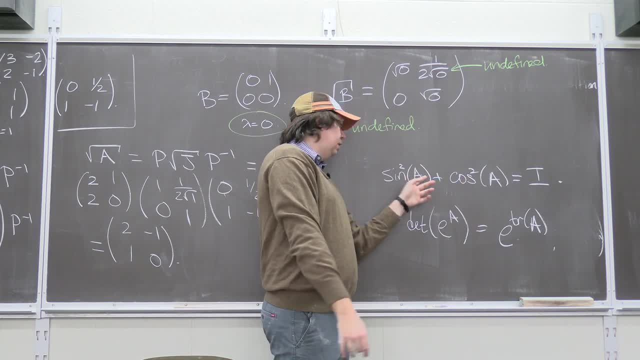 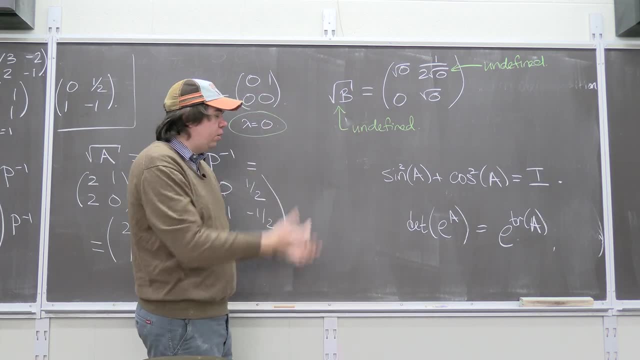 and you can just extend. It's pretty much like if things hold true for numbers, they largely hold true for matrices as well. There's some exceptions, right, But we've just been able to extend all these results from scalars to matrices. So we'll end there.